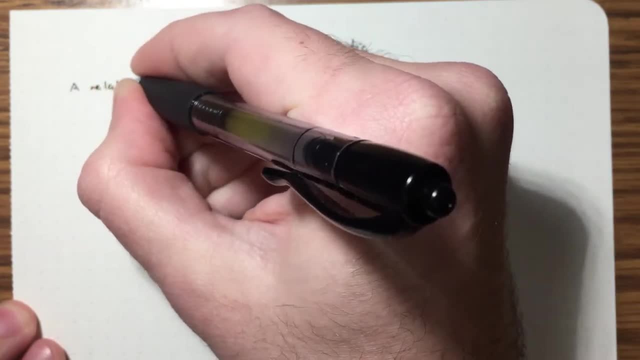 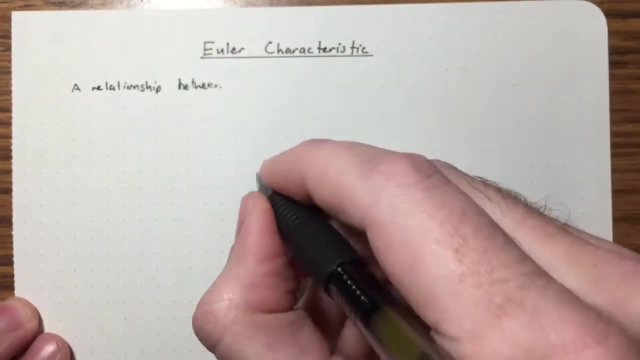 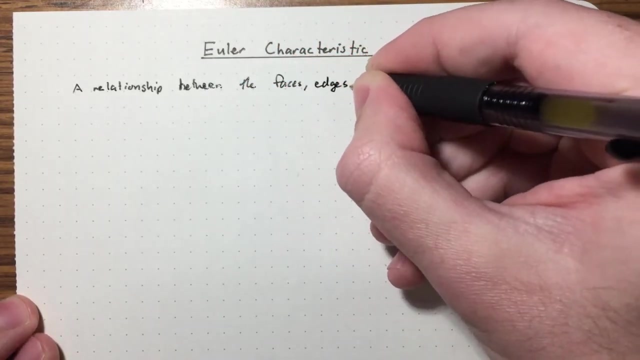 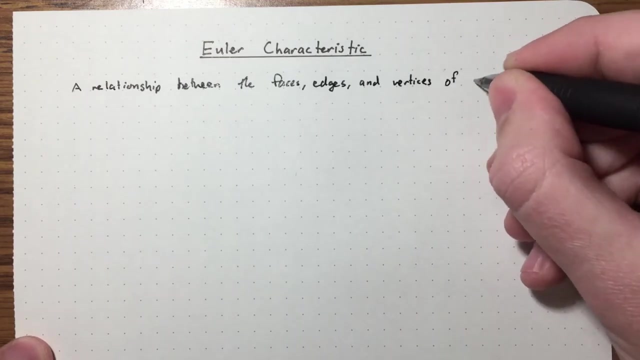 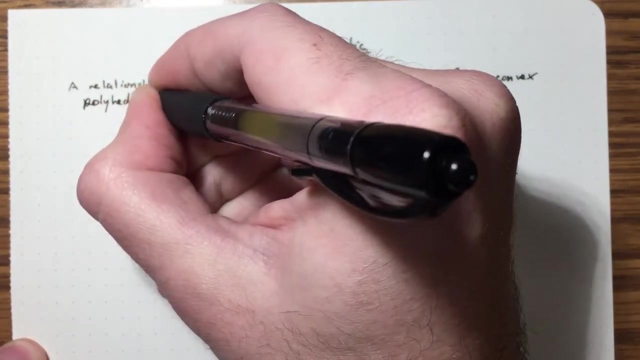 So the Euler characteristic is a relationship between three numbers, So it's a relationship between the faces, edges and corners And vertices, at least in the version I'm going to talk about of a convex polyhedron. What's a polyhedron? 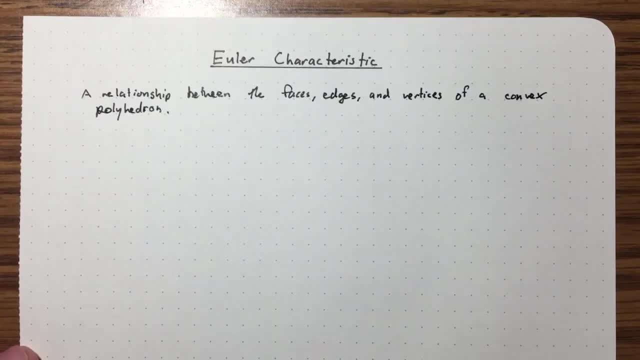 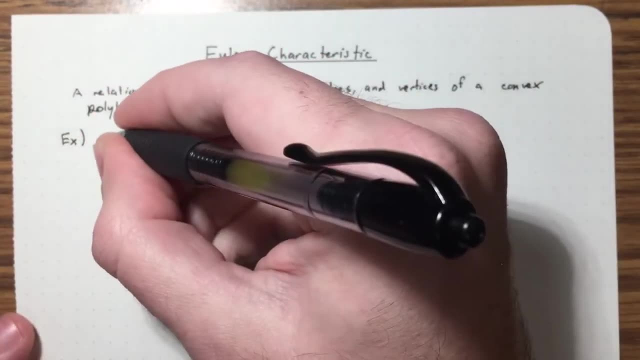 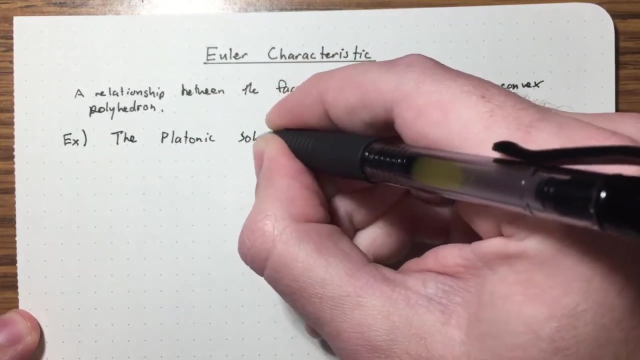 A polyhedron is a three-dimensional analog of a polygon, So I'll give you some examples of convex polyhedra. So the most basic example is what are called the platonic solids named after Plato, And there are five of these. 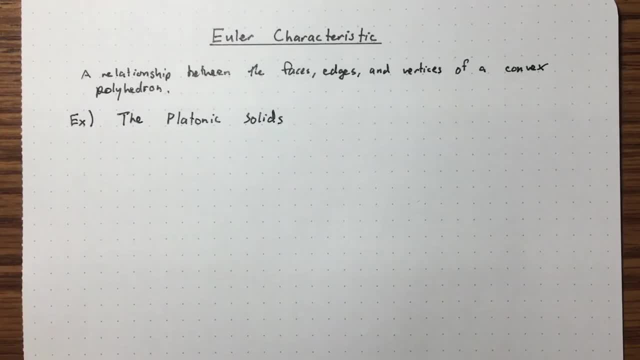 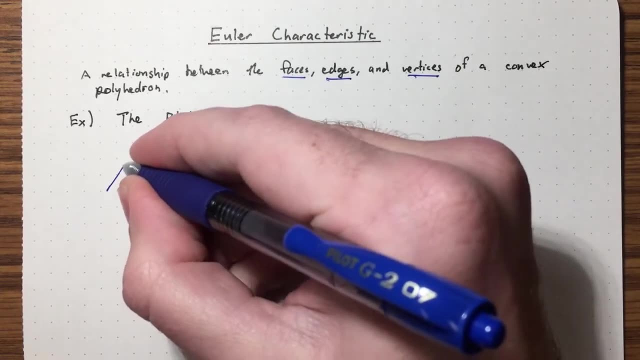 These are what are known as regular polyhedra, So you're only allowed to use one kind of shape as the face of the polyhedron. So if you use triangles, well, there are actually a few different ways you can use triangles, So I could do it like this: 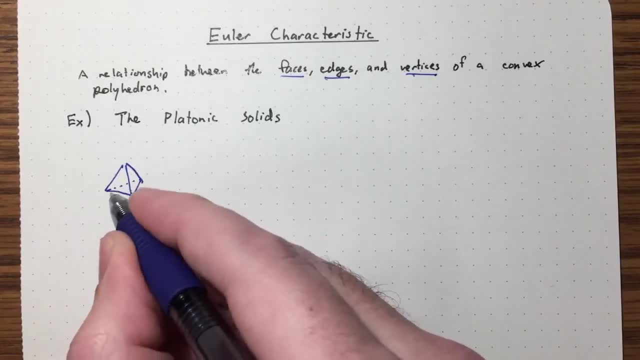 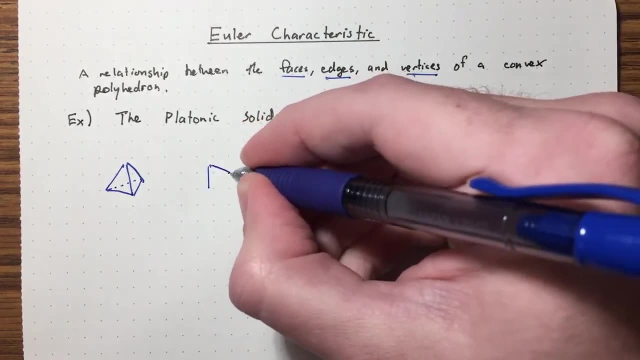 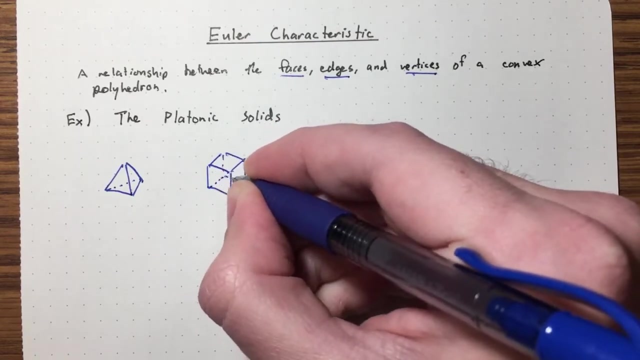 I could put together four triangles here. So the base is a triangle and I have three triangular sides, Or I mean the one that we are all very familiar with is a cube, So I'll try to draw a cube here. So it's another platonic solid. 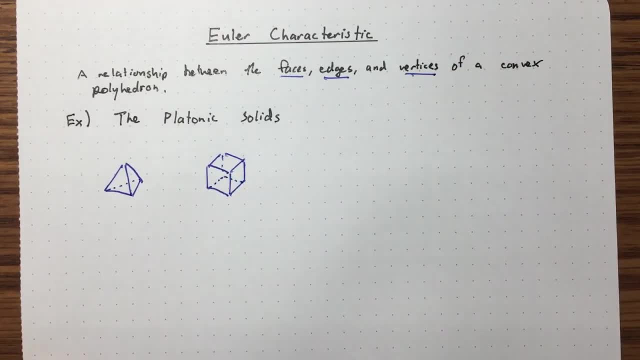 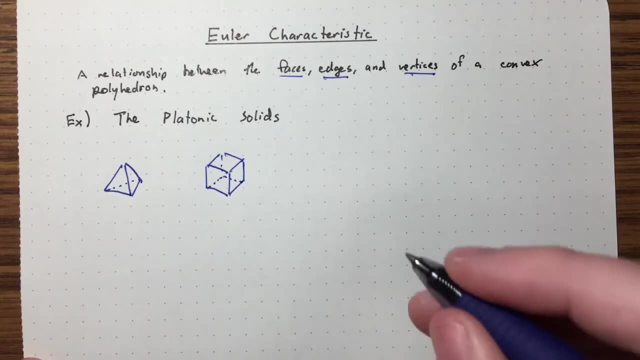 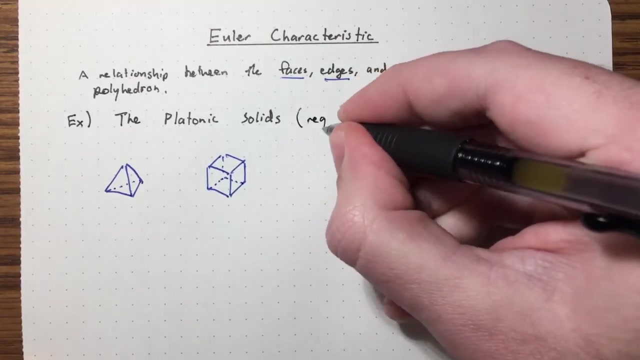 By the way, not only are you allowed to use one shape for the faces, but all of the vertices have to look the same. Okay, Okay, So for it to be a regular polyhedron. So these are also called regular polyhedra. 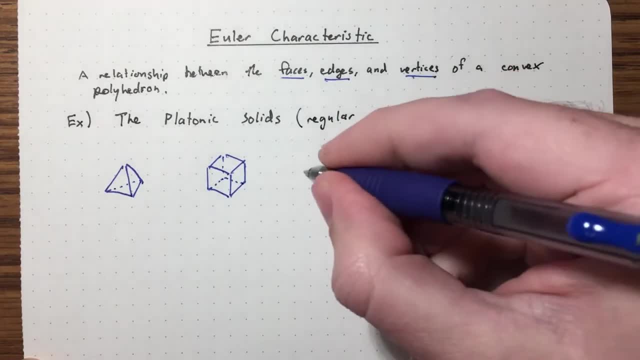 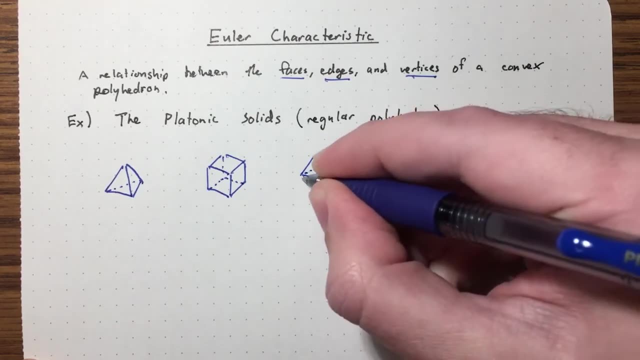 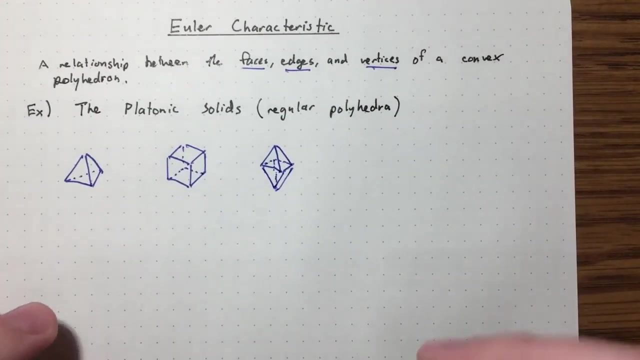 Polyhedra is the plural of polyhedron. Okay, and then we can have this one called the octahedron, So it's going to look like this: This one actually has eight triangular faces, And I'm a little scared to draw this one. 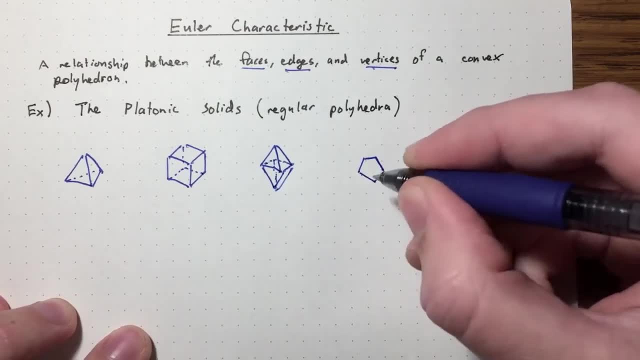 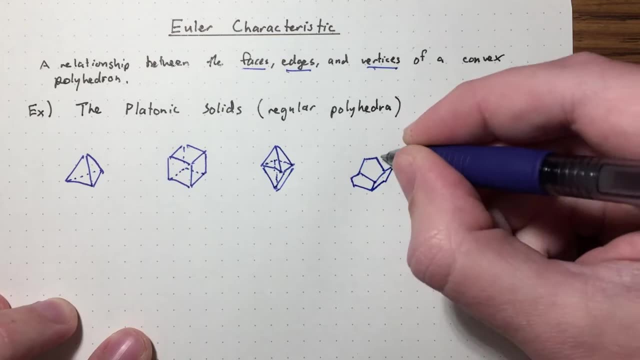 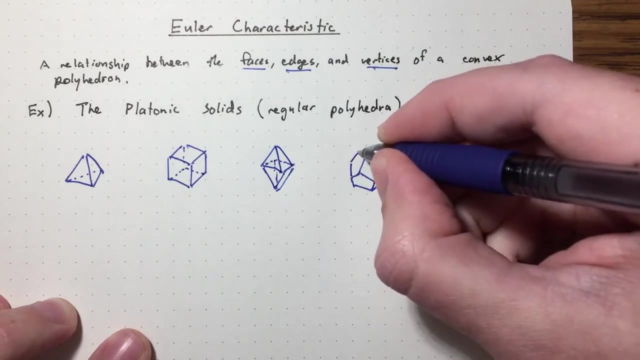 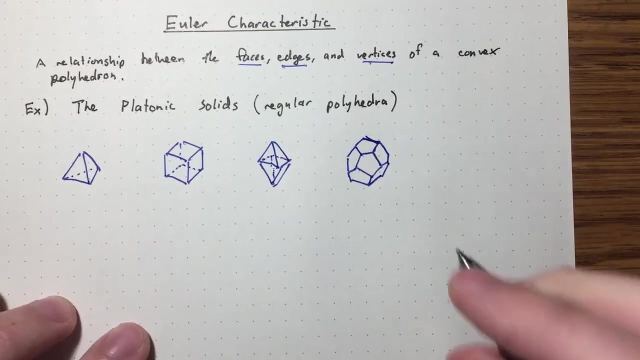 But we can actually use pentagons. You might have seen this one before. This is called the dodecahedron, Something like this maybe. Okay, so the faces are all regular pentagons, Something like that. It's a dodecahedron. 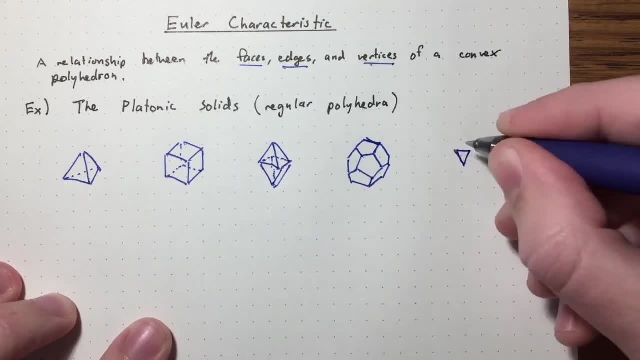 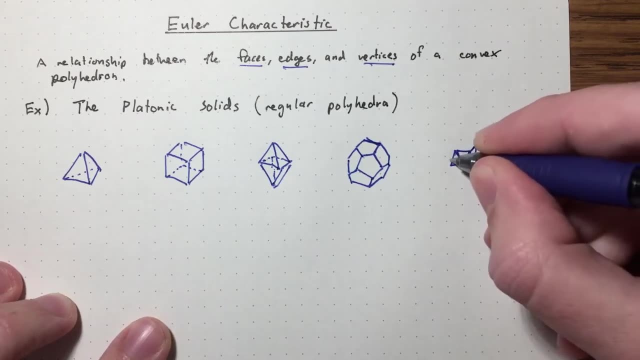 And then, finally, we have the icosahedron, And this again uses triangles only. I'm going to concentrate in order to draw this, But all of the vertices have to look the same. So in this one, you see, there are five triangles that meet at one vertex. 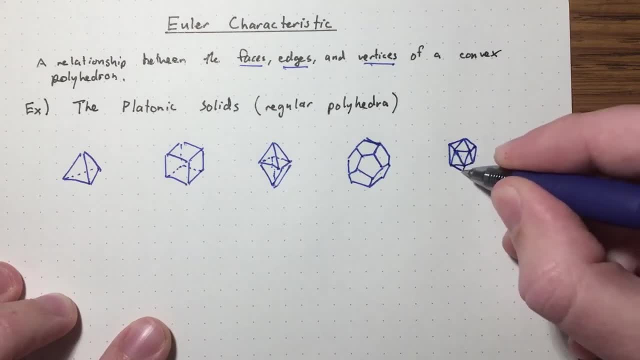 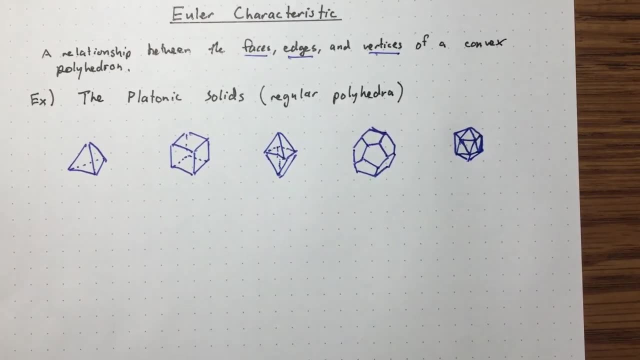 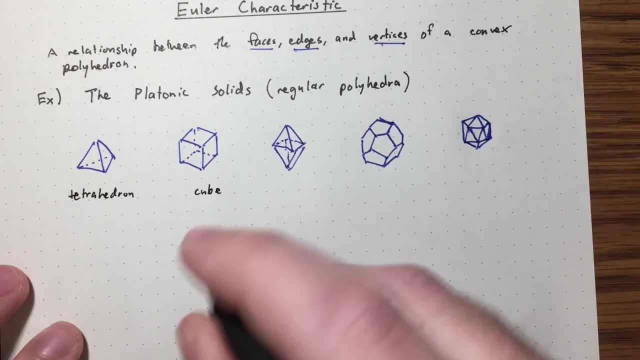 That's true for all the vertices. It kind of comes down like that: Okay, I'm not even going to try to draw the back part. Yeah, So what are the names? This is the tetrahedron. Okay, This is the cube, or hexahedron. 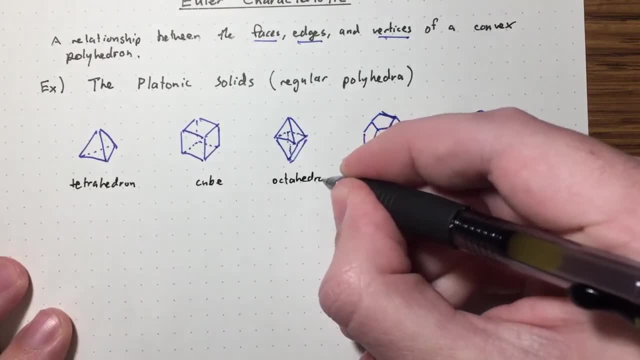 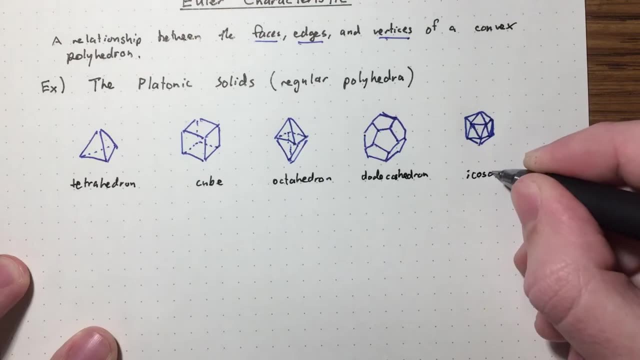 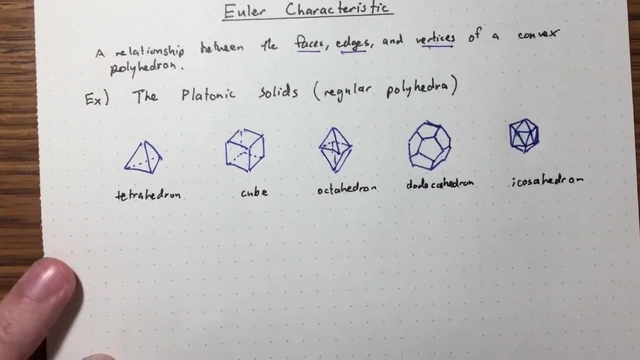 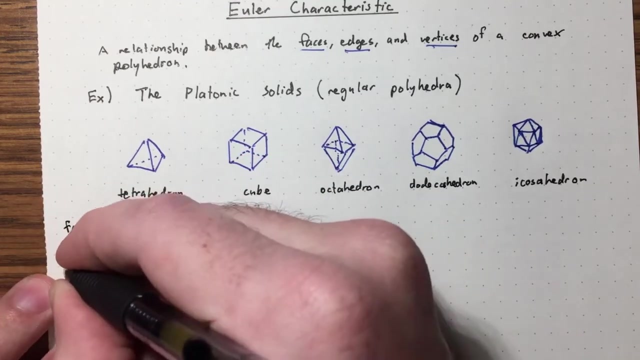 This is the octahedron, This is the dodecahedron And this is the icosahedron. Okay, So where does the Euler characteristic come in? So we're going to look at the faces, edges and vertices. 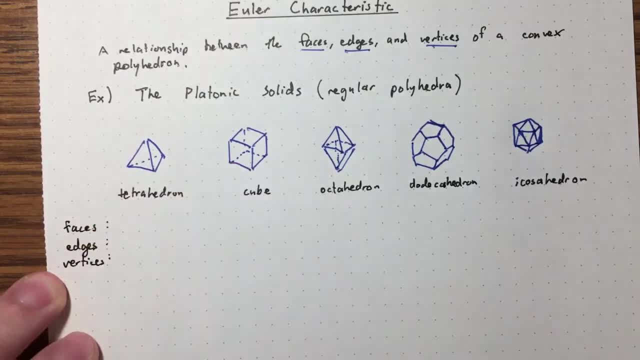 Okay. So how many faces do each of these have? Well, that's actually in the names. So tetra means four, Hexahedron, the cube is six. There are six faces on a cube. These are the squares. 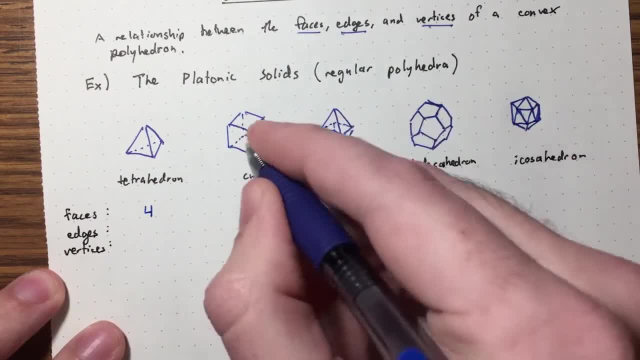 Octahedron has eight faces. These faces again are just the flat surfaces, So there are eight triangular faces. The dodecahedron- you can't really see the back of it, but take my word for it: It has 12 pentagons. 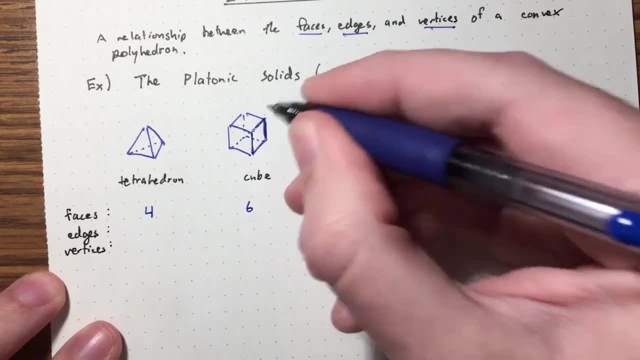 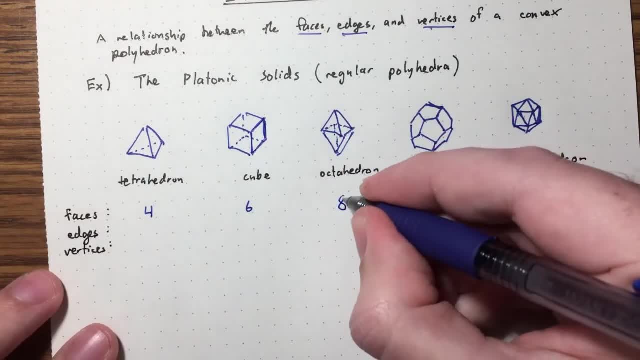 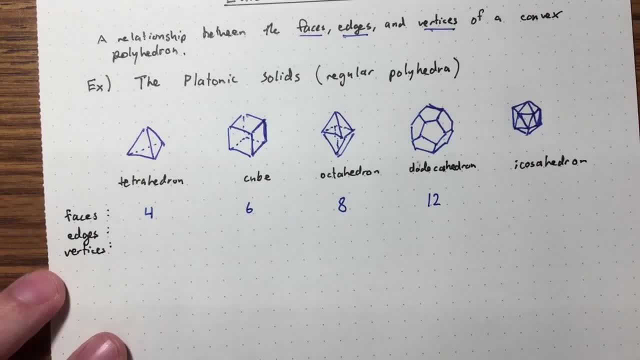 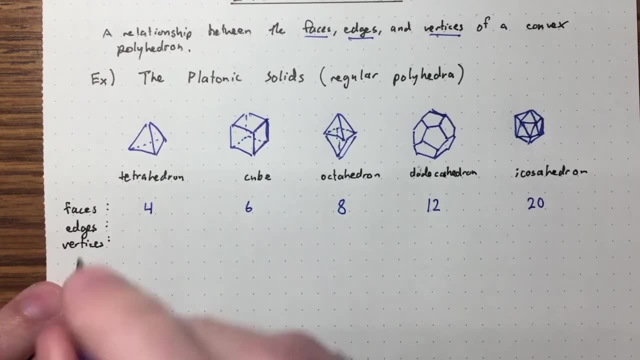 The dodecahedron. you can't really see the back of it, But take my word for it. it has 12 pentagons. The icosahedron has 20 triangles, Okay Edges. The tetrahedron has six edges. 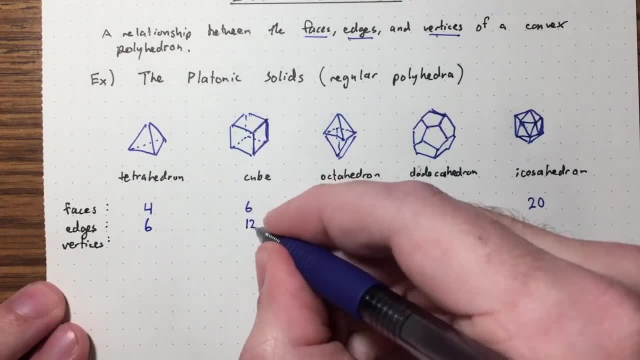 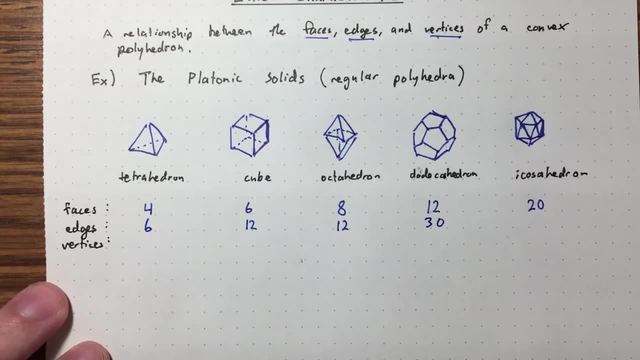 You can just count them. The cube has 12 edges And so does the octahedron, actually The dodecahedron, you will take my word for it. You can just count them, And they are four scoop edges. 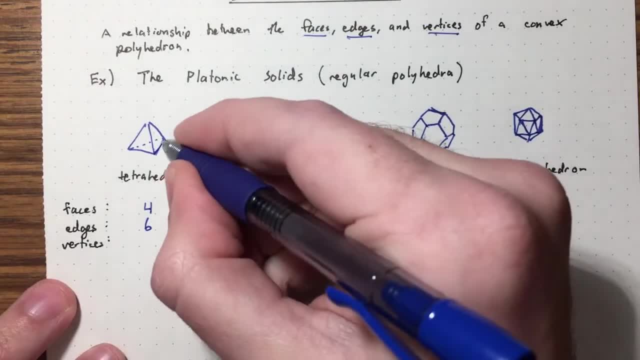 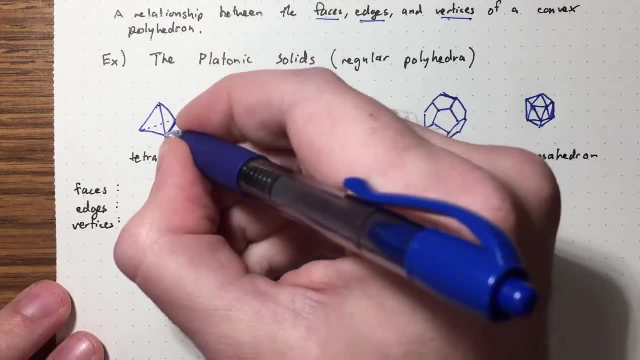 And the icosahedron also has 30 edges. So these are the edges here: straight lines connecting two faces And the vertices. so what are the vertices? They're just the points, okay, So they're where the edges meet. 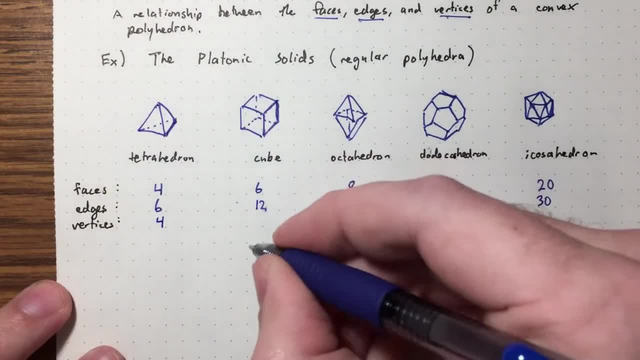 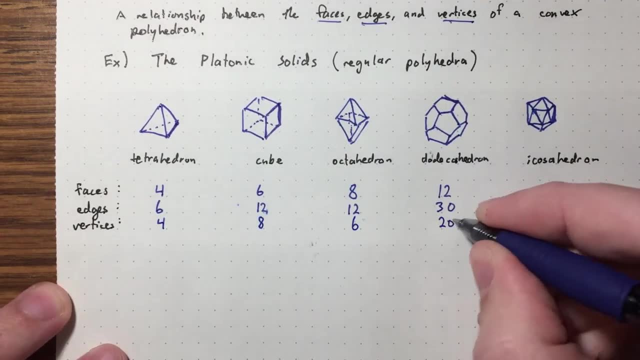 The tetrahedron has four vertices. Again, you can just count four of them. The cube has eight. The octahedron has- let's see- one, two, three, four, five, six. The dodecahedron has 20.. 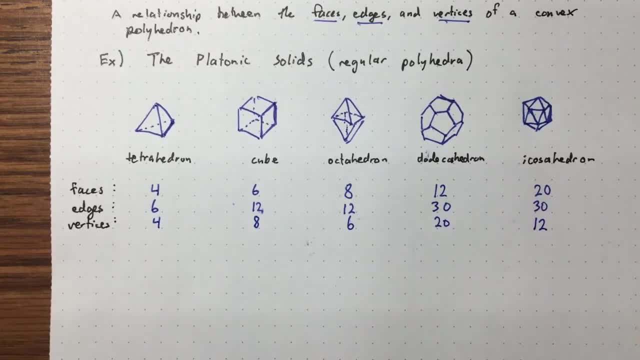 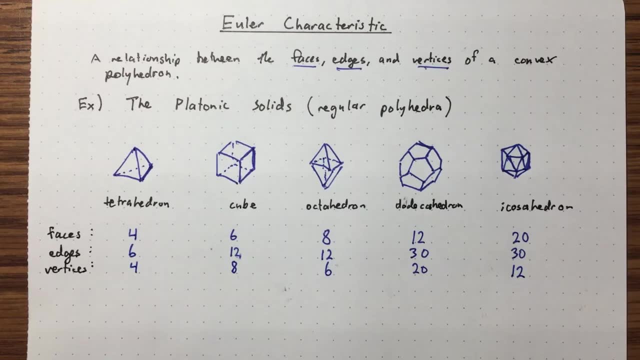 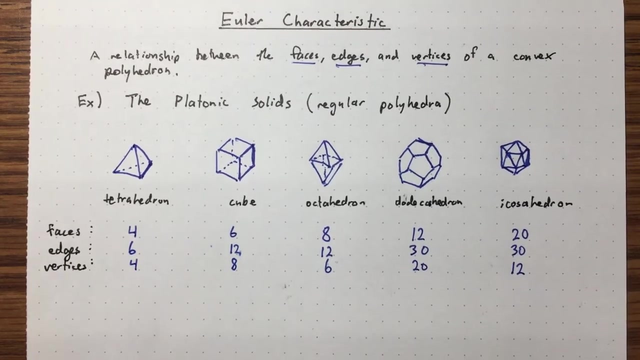 And the icosahedron ends up having only 12 vertices. Okay, at this moment I'd actually like to pause and give you the opportunity to try to see if you can find a relationship between these numbers. So, for each of these shapes, 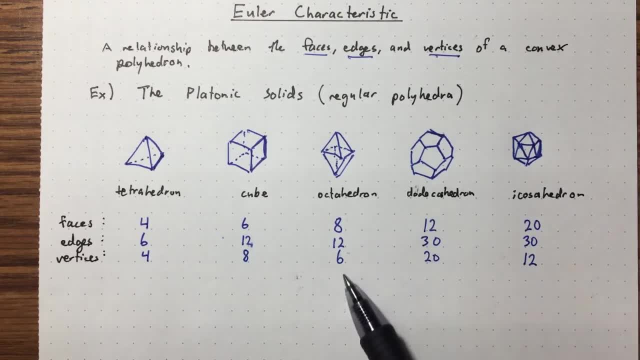 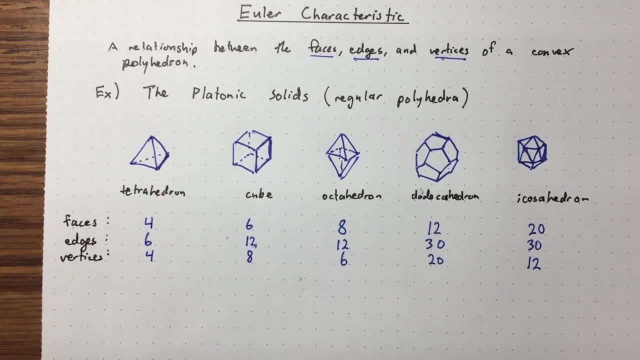 each of these platonic solids. is there a relationship between these three numbers, faces, edges and vertices? And it turns out there is, And it works for all five of them. So this is a great chance to pause your video, see if you can figure out a relationship. 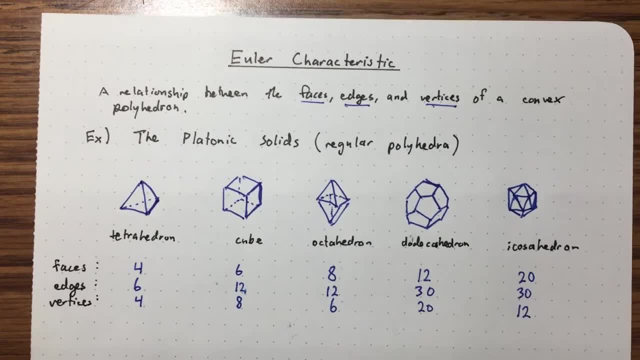 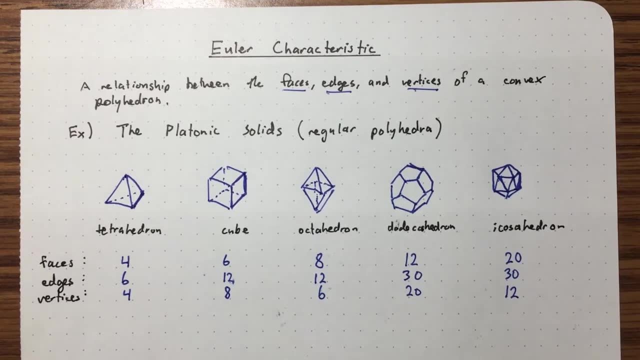 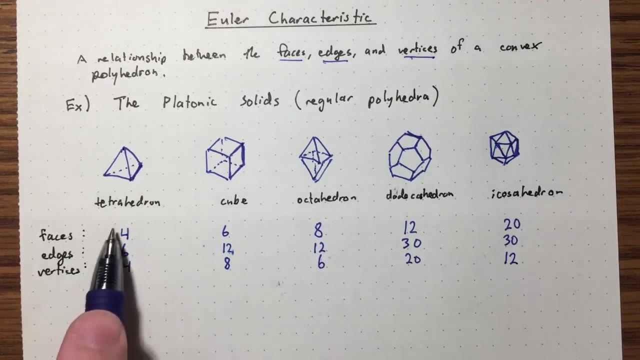 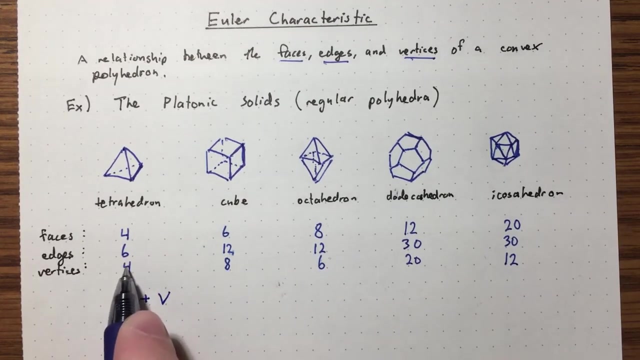 between these three numbers, Then I'll tell you what the relationship is. Okay, so what you might have noticed- and this is what Euler discovered- is that if you take the faces and you add that to the vertices, okay, so four plus four, that's eight. 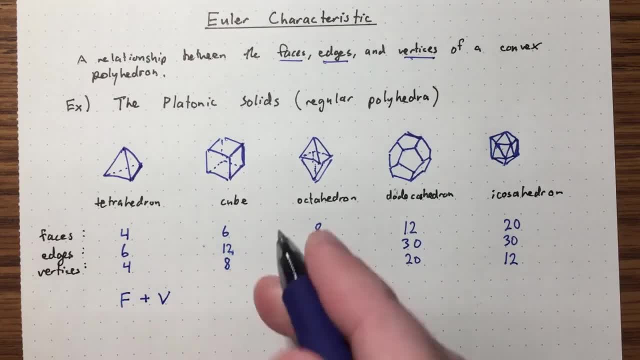 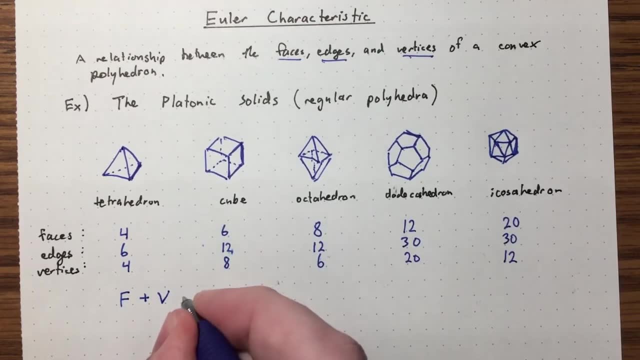 Eight is two, Four more than six. But look at the cube. Six plus eight is 14.. 14 is two more than 12.. It turns out that works for all of these. So faces plus vertices is the edges plus two. 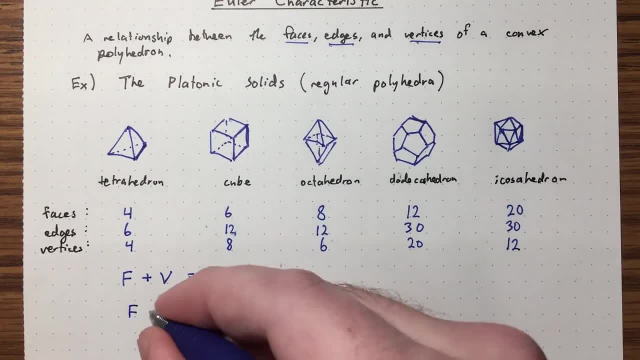 Okay, so if I move everything on the same side, so faces minus edges, I'll put them in this order, Because faces are sort of like two-dimensional objects. Edges are one, Edges are one-dimensional objects And vertices are zero-dimensional objects. 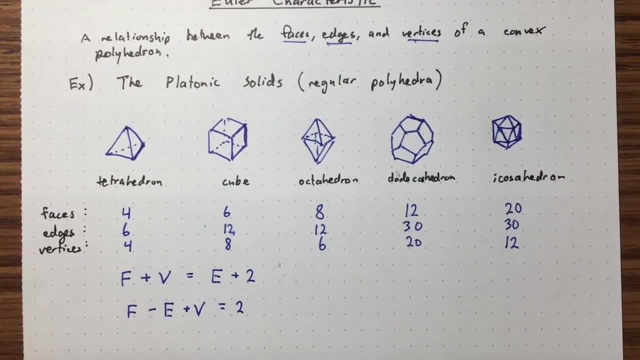 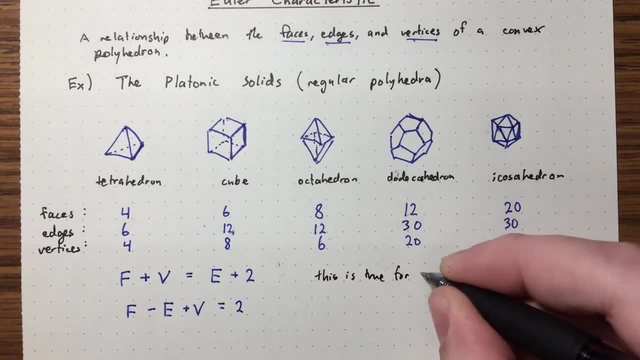 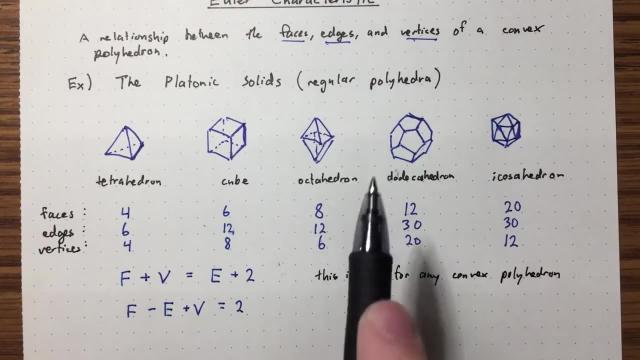 So faces minus edges, plus vertices equals two, And this is actually true. This is true for any convex polyhedron, Not just these regular ones. You can actually have different shapes, like a soccer ball, for example. It uses pentagons and hexagons. 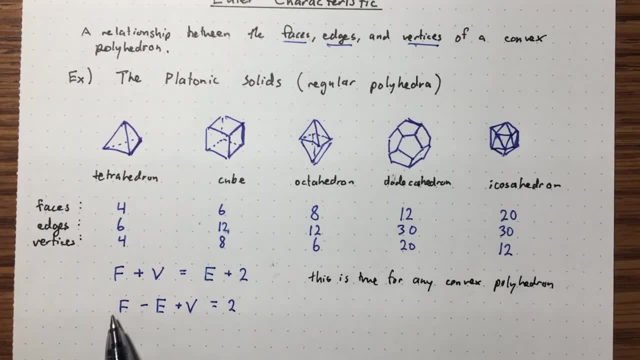 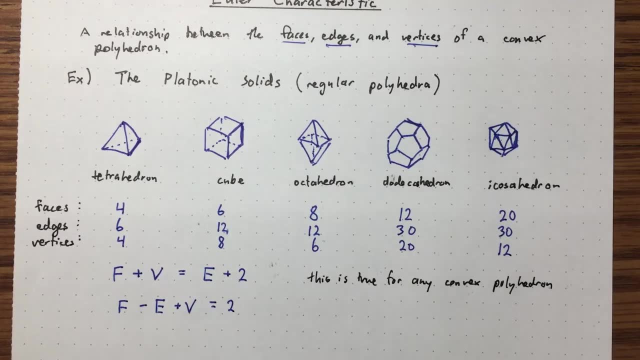 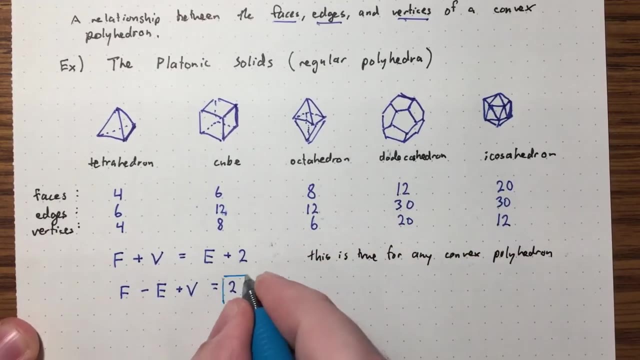 But if you count up faces, edges and vertices- and you have faces, edges and vertices, you always get a number two. That's pretty remarkable, And so this was found by Euler And this two right here. so the value of faces minus edges, plus vertices. 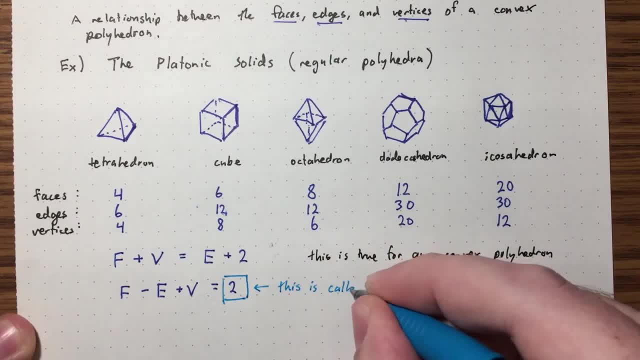 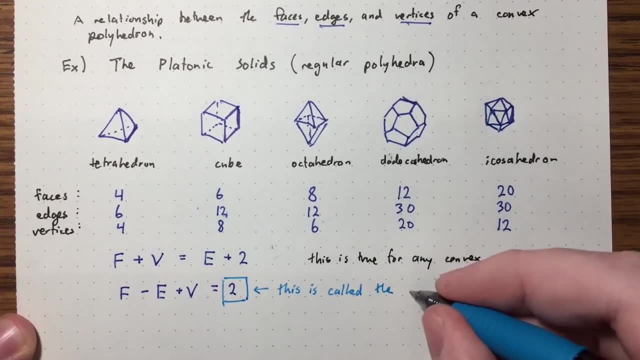 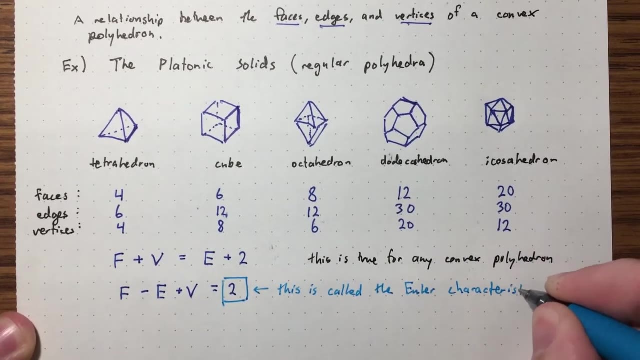 this is called the Euler characteristic. So the Euler characteristic is faces minus edges plus vertices, And for a convex polyhedron it's always two. So the Euler characteristic is always two for a convex polyhedron. Okay, So this is cool and everything. 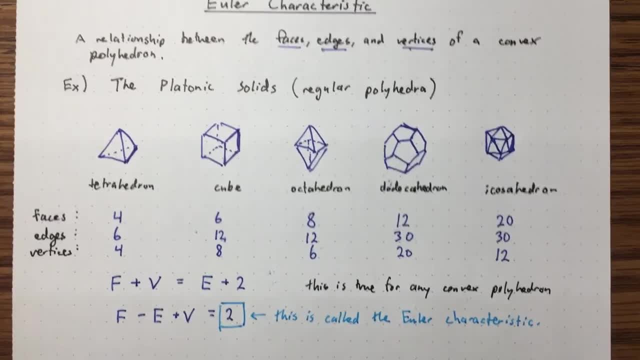 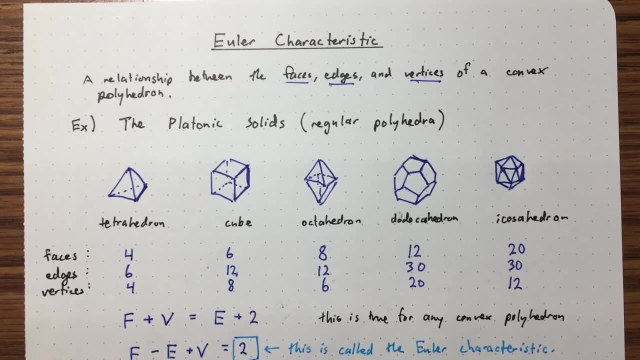 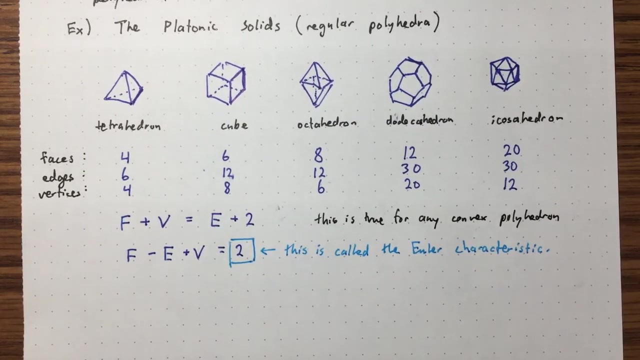 but where does linear algebra come into this? What does linear algebra have to do with polyhedra? Okay, so the amazing thing is that it turns out that this relationship right here that you might have just found by playing around with these numbers, this is actually the rank nullity theorem in disguise. 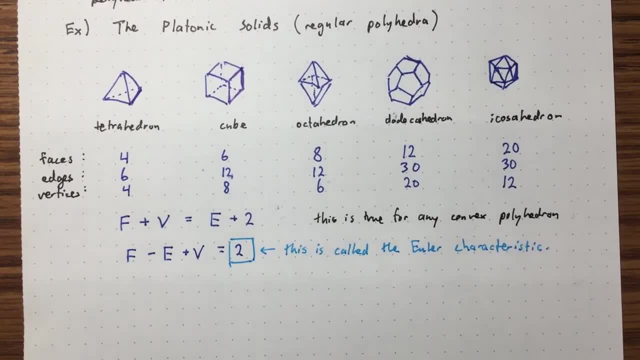 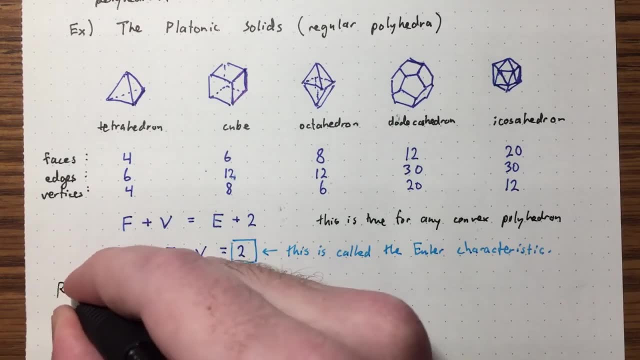 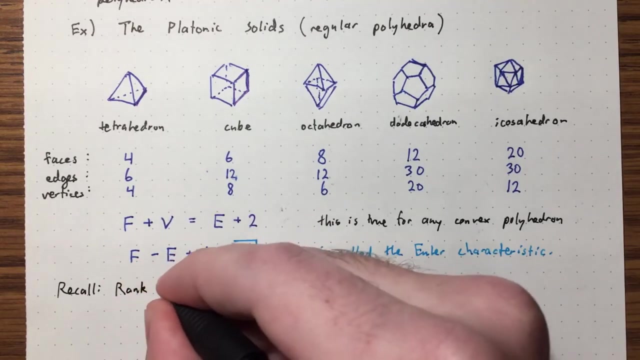 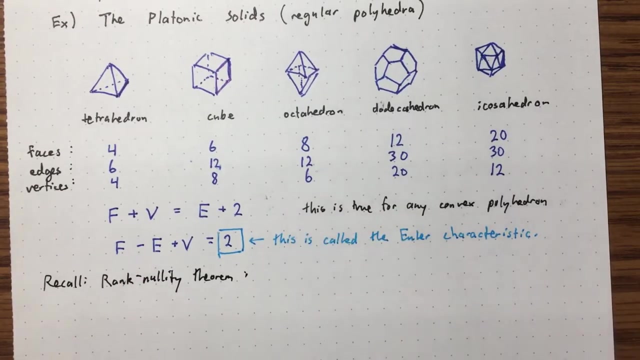 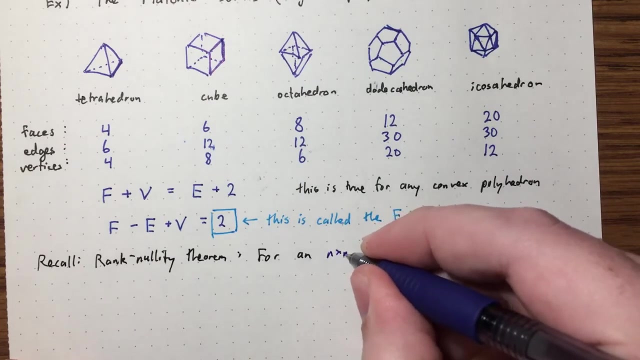 So hopefully you're intrigued by that. Let's see how that works. So let's just recall what the rank nullity theorem is. The rank nullity theorem, What does it say? It says that for an. Let's see. It says that for an n-by-m matrix. 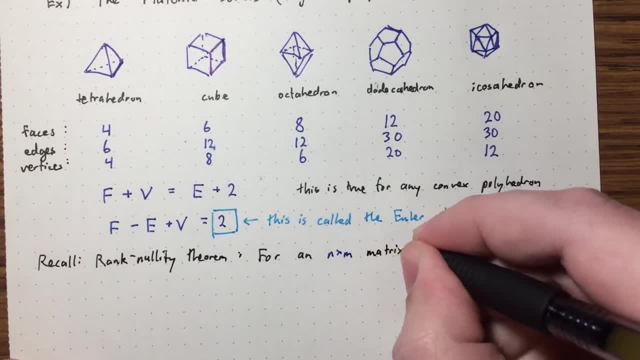 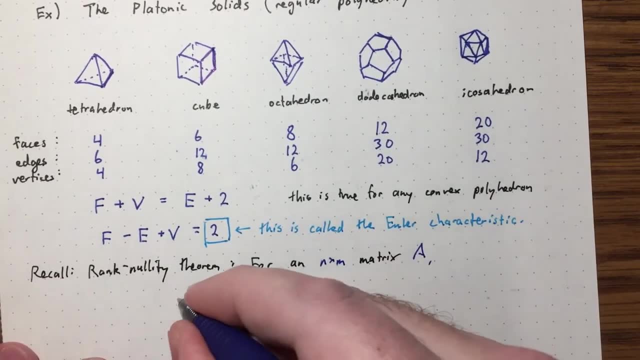 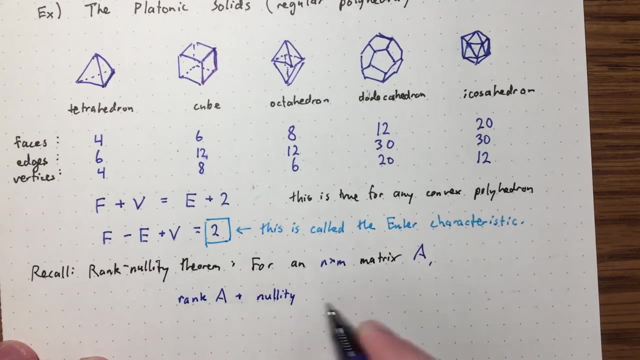 n-by-m matrix A, the rank of A plus the nullity of A, and the rank is the dimension of the column space. the nullity is the dimension of the null space, and that's always going to equal. Which one should I write? 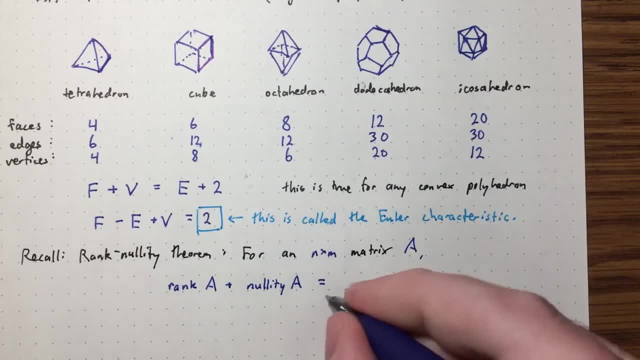 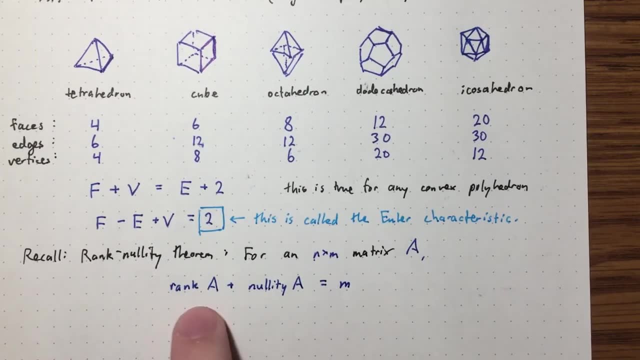 M or N? M? right, It's the number of columns. This is rows, that's columns. Okay, so number of columns is always going to be the sum of the dimension of the column space and the dimension of the null space. 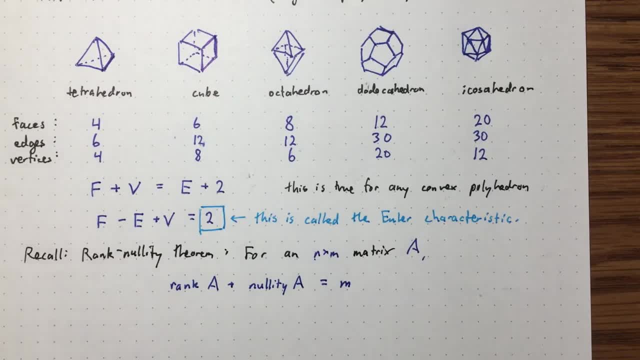 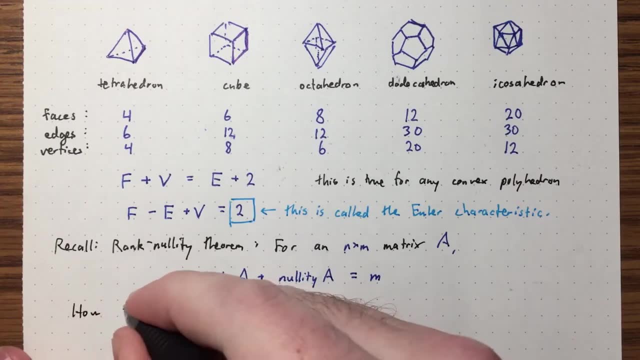 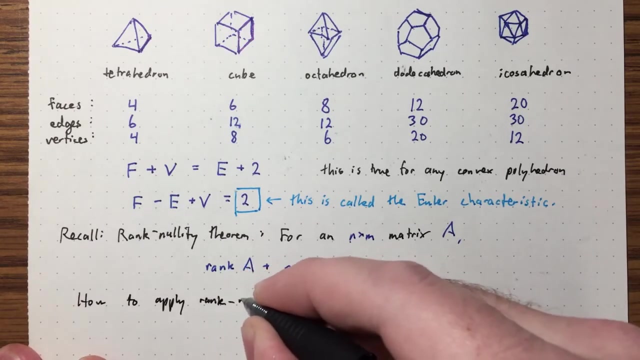 Okay, how do we apply that to this problem? Well, we need a matrix, right? So we need a matrix to start with. So yeah, let's just ask that question: How to apply Rank nullity to this problem. So yeah, if we need a matrix. 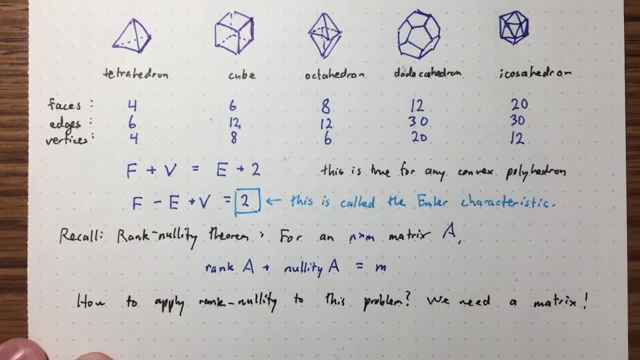 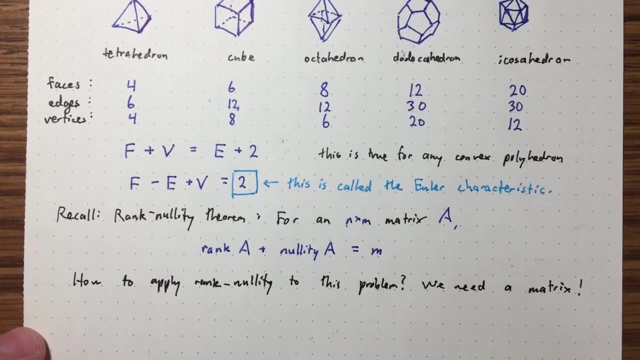 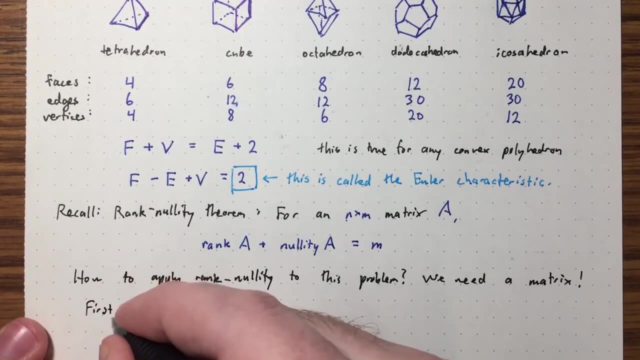 what is the matrix going to be? Well, it turns out it's going to be known as the incidence matrix of a graph that we're going to associate to each of these polyhedrons. So first, given a polyhedron, any polyhedron, 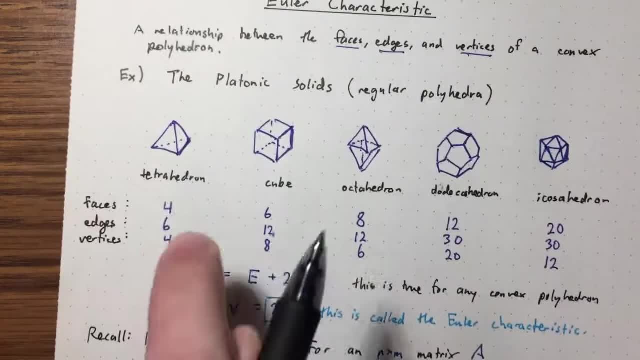 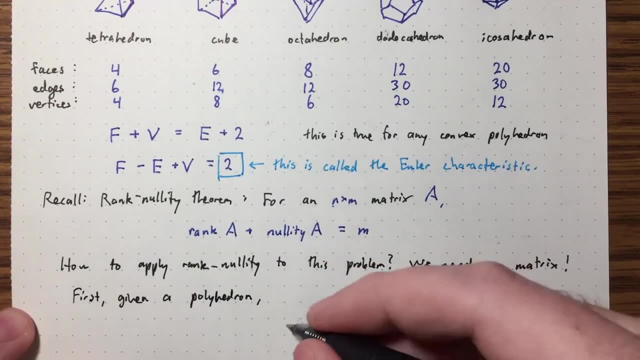 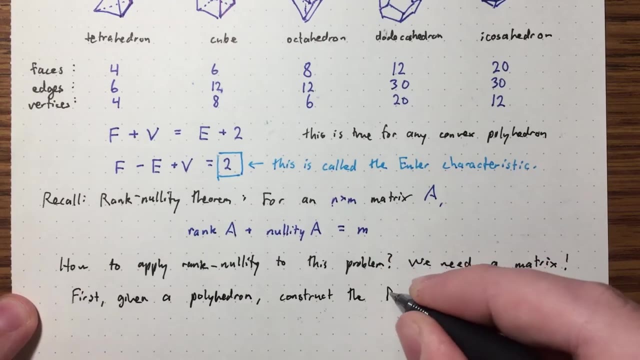 we can take one of these, for example. Maybe what we'll do is we'll work with the tetrahedron when we're going through this calculation, just to have something concrete to look at. So, given a polyhedron, construct the flat. 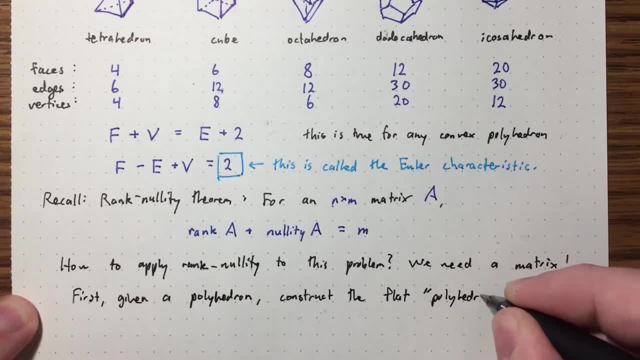 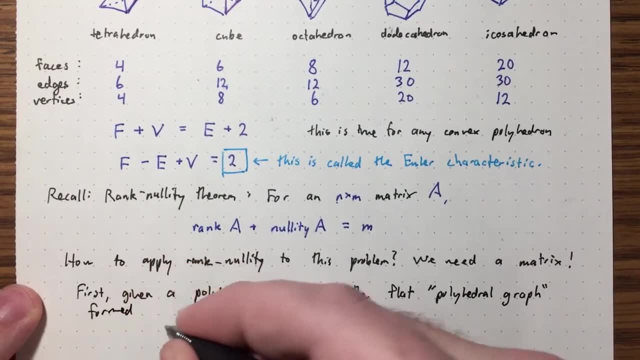 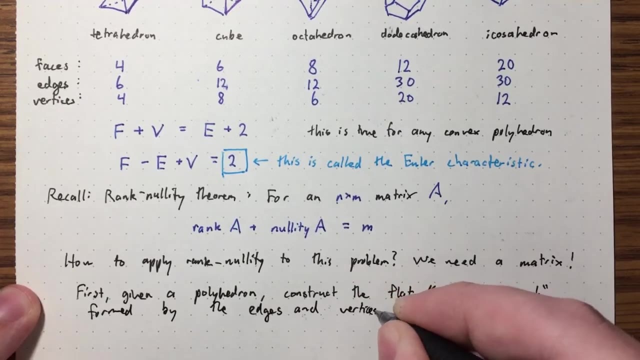 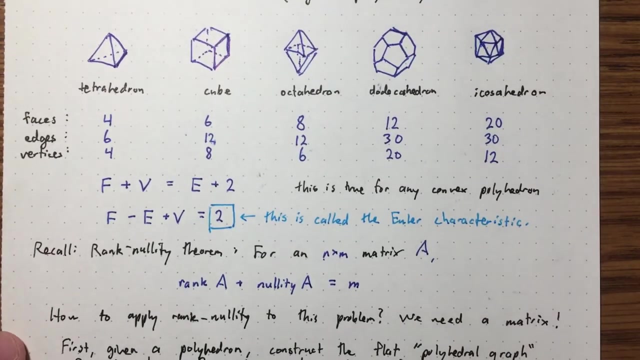 We're going to call it a polyhedral graph, And by graph I mean something with nodes and edges and network. So that's going to be formed by the edges and vertices of the polyhedron. Okay, so let's take the tetrahedron, for example. 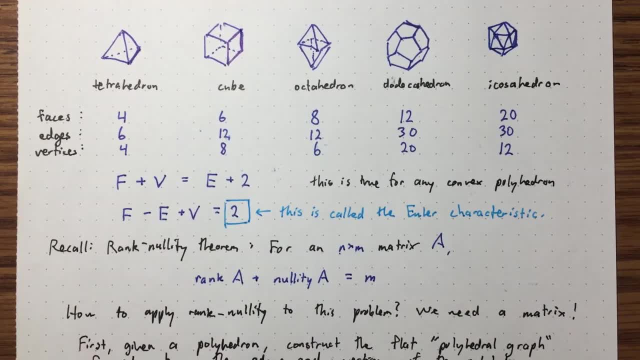 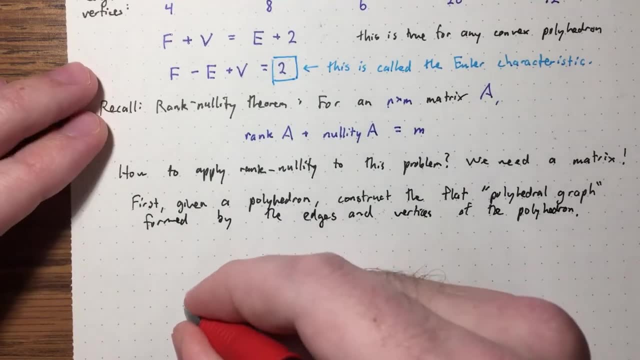 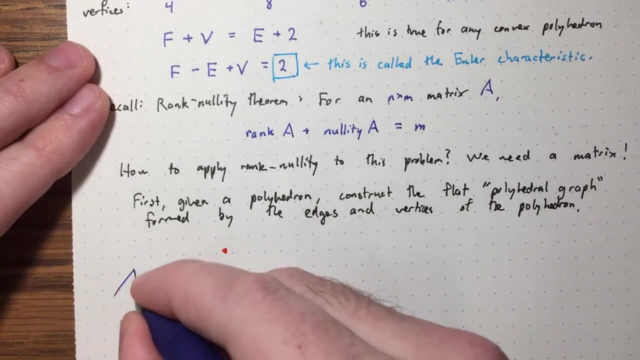 So what do we want? We want some colors. Let me decide what colors to use. So I'm going to take the four vertices of the polyhedron and let's draw it like this. So I'm starting with the tetrahedron again. 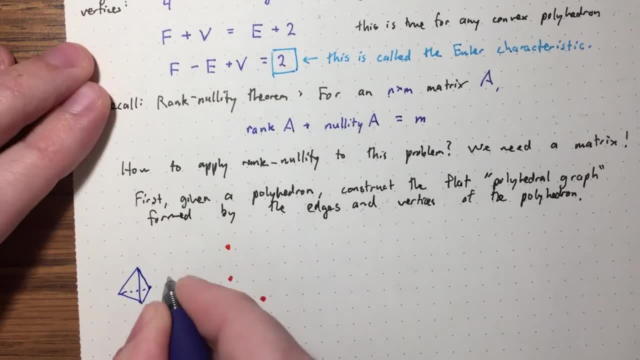 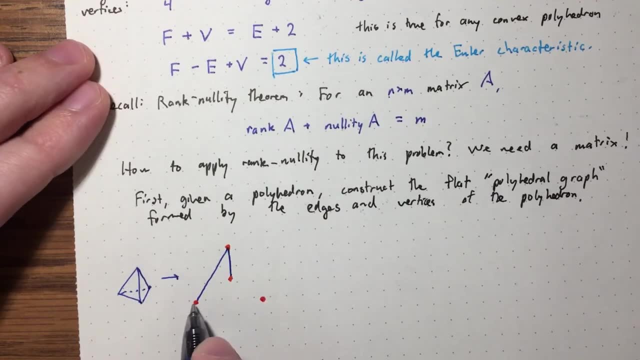 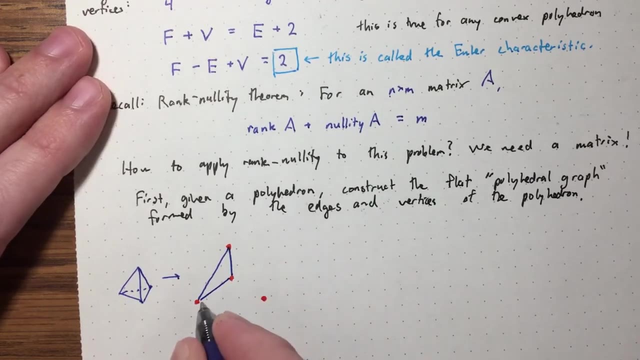 So I have my tetrahedron And I'm going to associate to it this graph. So this is the top vertex and these are the other three, And I'm putting the same edges on as this has, basically, And I'm just trying to make it lie flat. 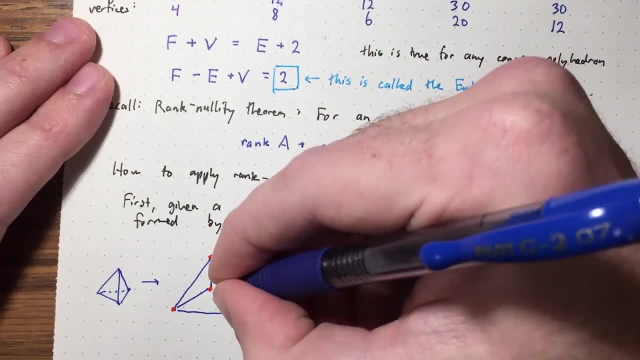 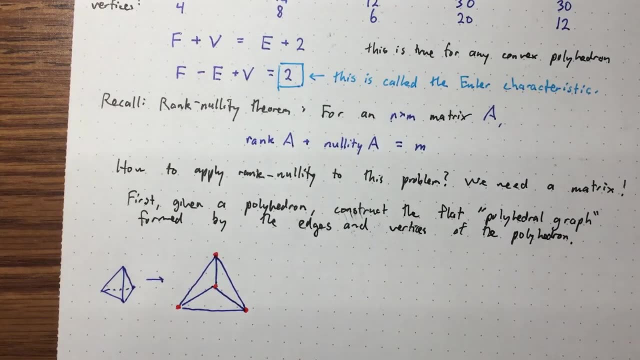 That's the idea. Okay, so it's going to look like this. You can also imagine removing the base of this tetrahedron, Just taking off one of the sides and then sort of squishing it down on a piece of paper. 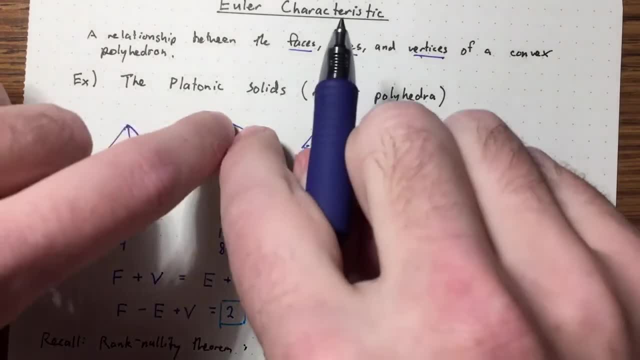 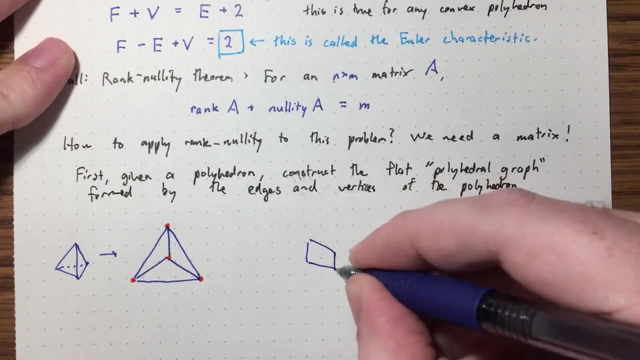 So let me show you what that would look like for the cube. Imagine removing one of the faces of the cube and then sort of squishing the rest of it down So it's lying flat. Here's what it would look like for the cube. 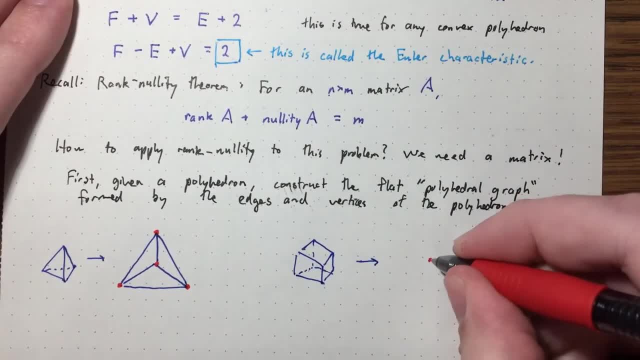 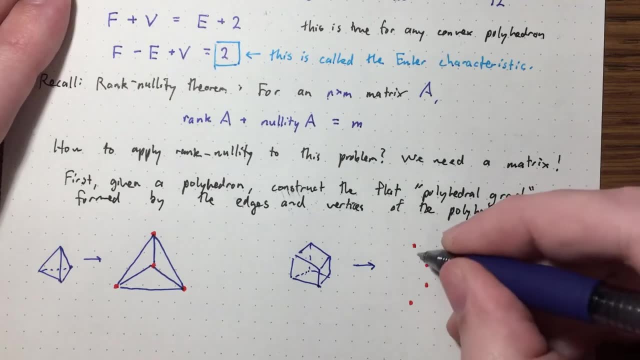 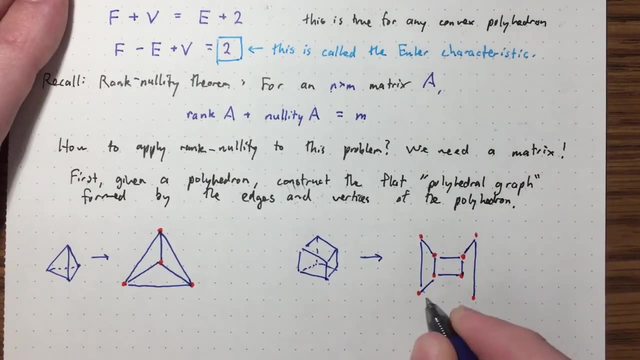 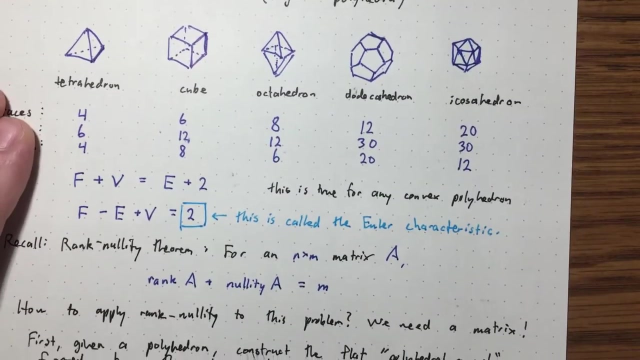 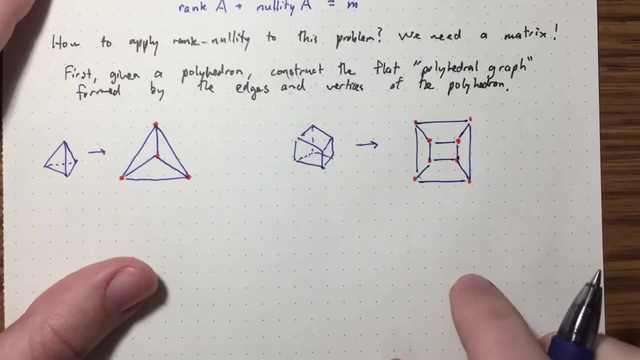 You, I have one of the faces and I sort of squish the rest down And it looks like this. You kind of see that, Um, it's like I removed the bottom and then just squished it flat. Okay, So there's my polyhedral graph for the cube. 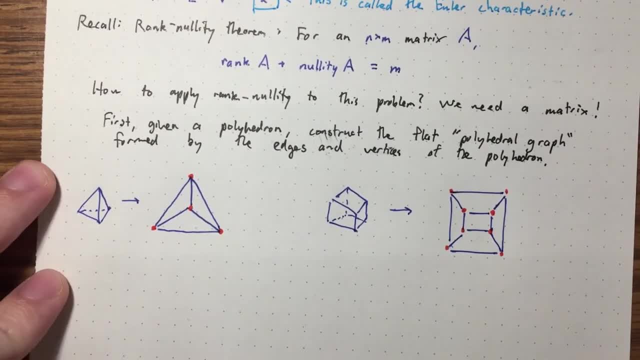 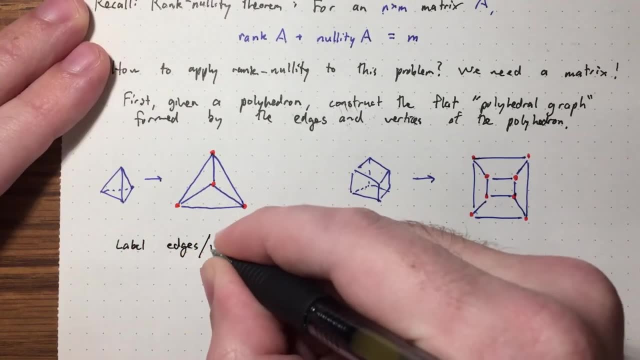 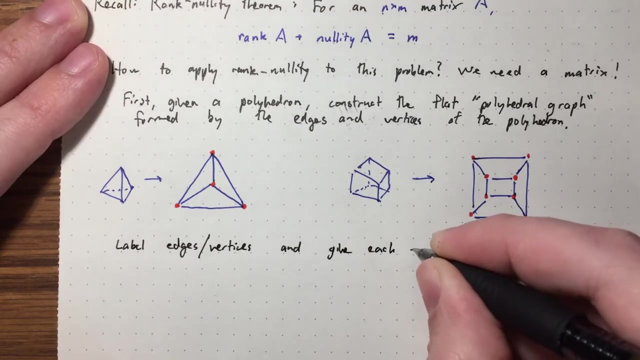 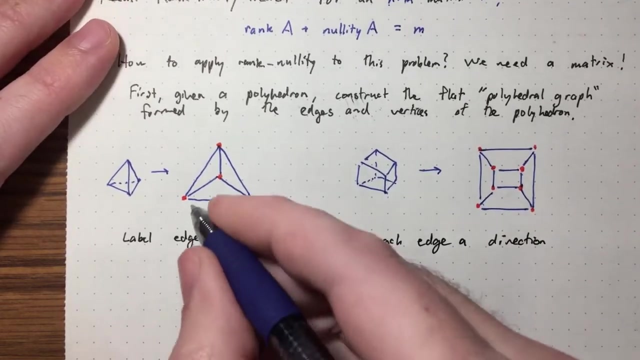 or the hexahedron. The next one I'm going to do is that I'm going to label the edges and vertices And I'm going to give each edge a direction. What do I mean by that? So let's do it with this one here. 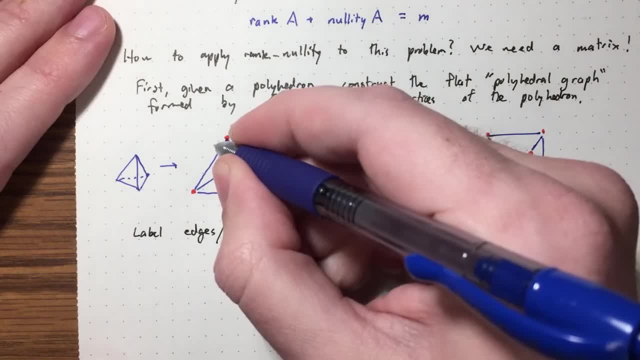 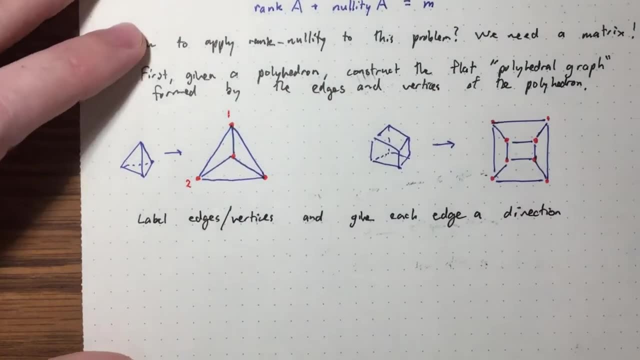 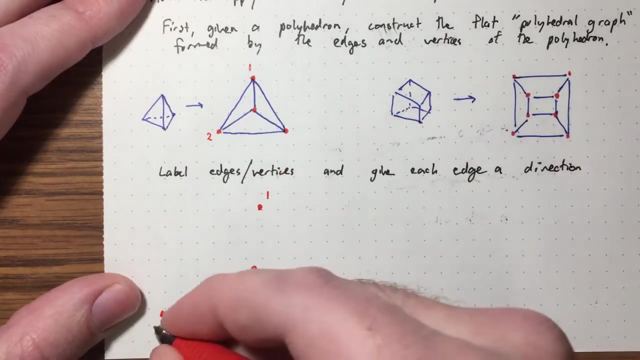 So I'm going to label. So let's label this one, one, two. So let me make a bigger picture. Sorry about that, Okay. So here's my graph. I'm going to label one, two, three, four. Draw all the edges in. 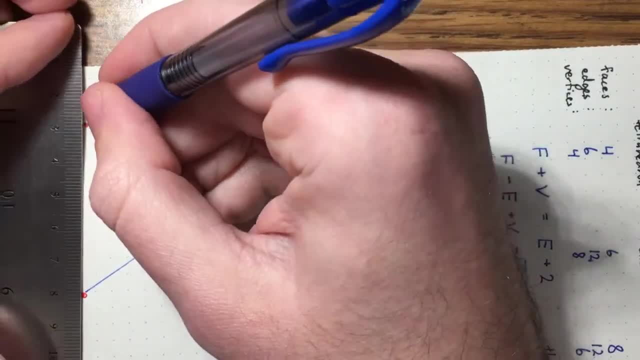 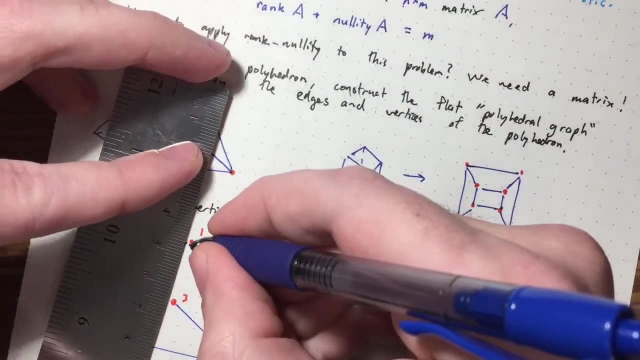 This is actually a very general construction that I'm going to do here. It has applications in lots of things other than polyhedral, like networks or electronic circuits, for example. So what I'm going to do is I'm going to- yeah. 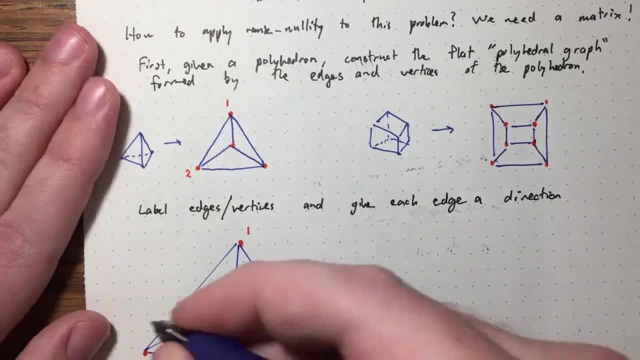 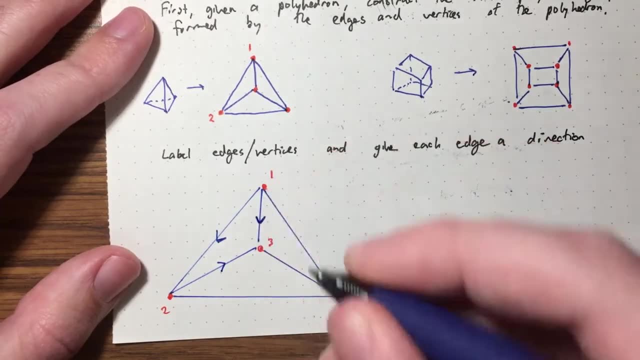 I labeled the vertices Great. Now I'm going to assign each edge a direction. So let's say that one's pointed that way, This one's pointed that way. You can choose them however you want. I want to be that way. 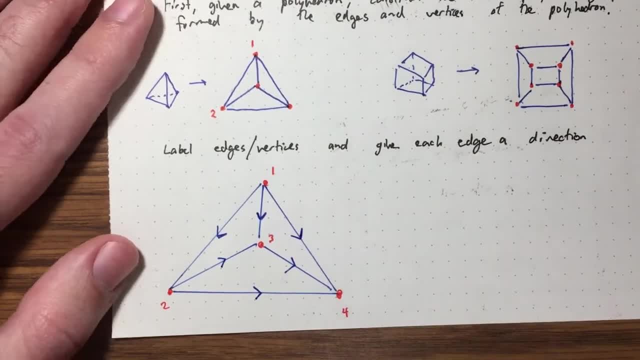 Let's- yeah, let's make this one pointed that way. Yeah, let's make this one pointing down also. It doesn't matter too much. Now I need to label the edges, So I'm going to label this one edge one. 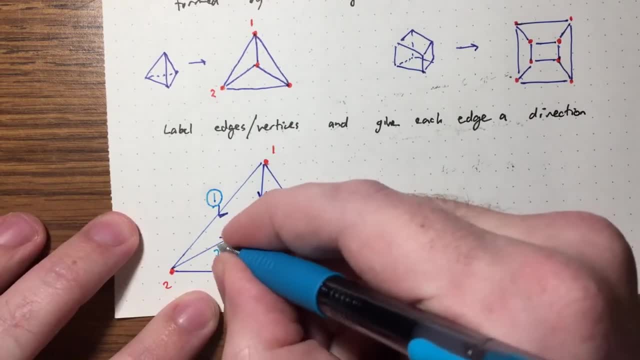 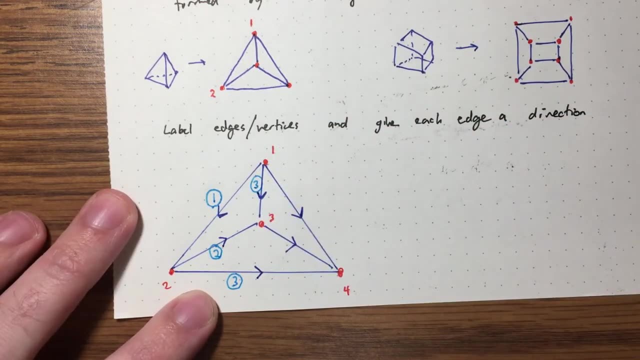 and I'll circle it so it looks different than the vertices. This will be edge two. This will be edge three. This will be- let's make this edge three. And this one will be edge four. Again, it doesn't matter, but this will be edge four. 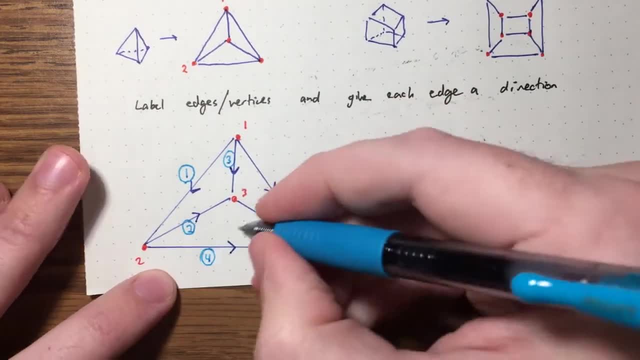 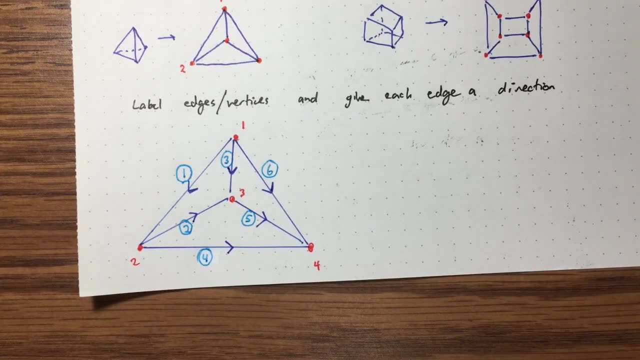 I just want sort of a loop here for the first three. This one will be edge five and this one will be edge six. Okay, Now is the exciting part: We're going to form the incidence matrix of this graph. So let me get a new piece of paper. 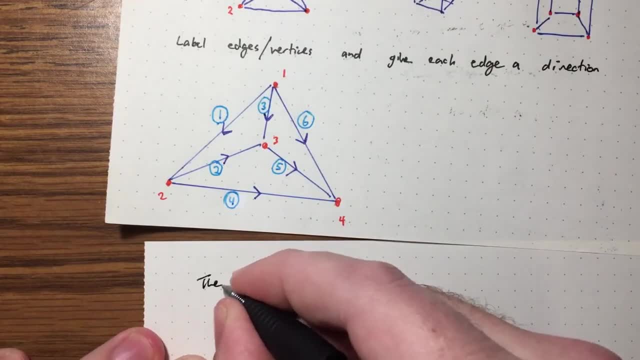 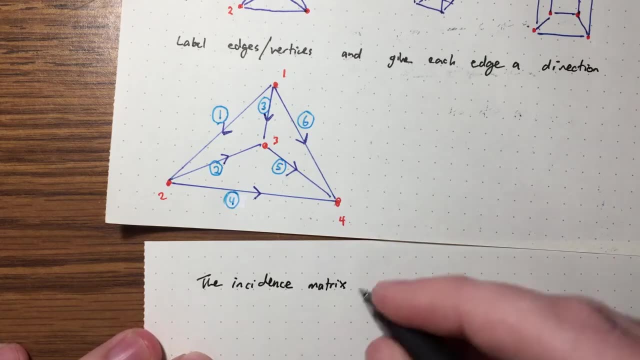 I'm going to keep this picture on here though. So now the incidence matrix. Again, this is a very general construction that you will likely see again. So the incidence matrix of a, specifically, this is a directed graph. The edges have directions. 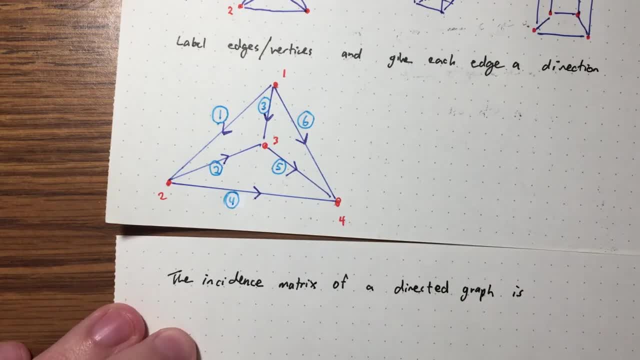 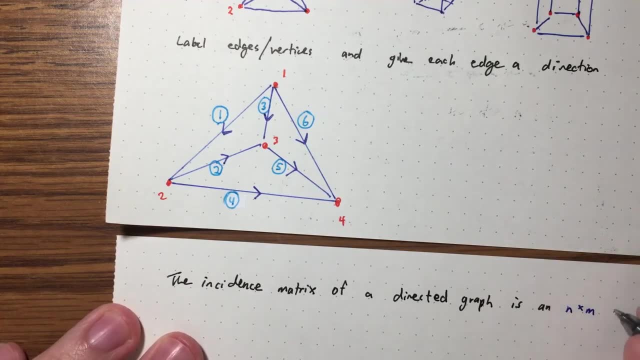 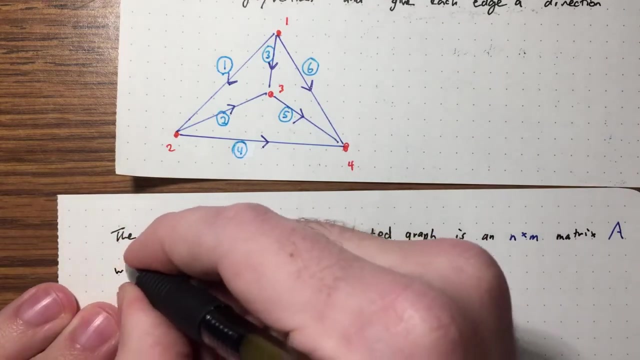 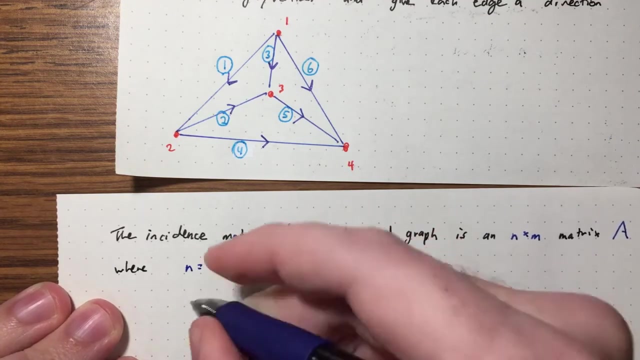 Is okay, it's N, N by M matrix. Let's give it a name, A, Where what is N going to be? N is going to be the number of vertices And M is going to be the number of edges. 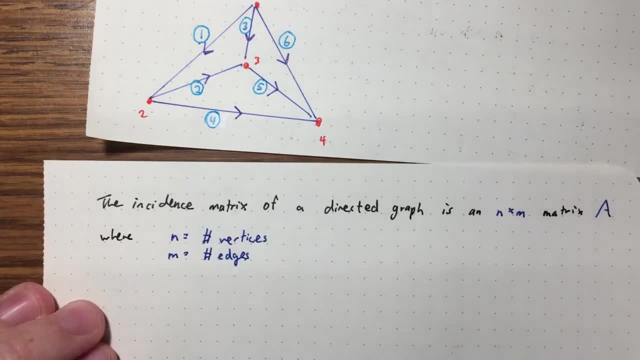 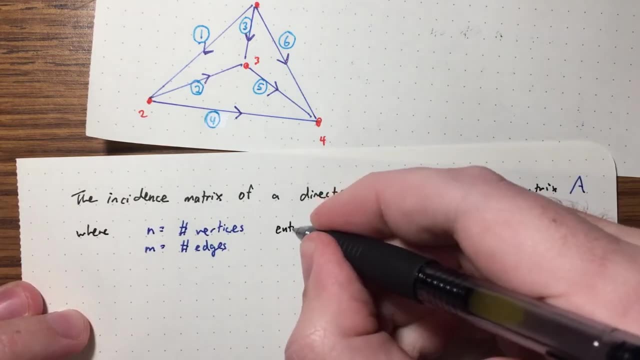 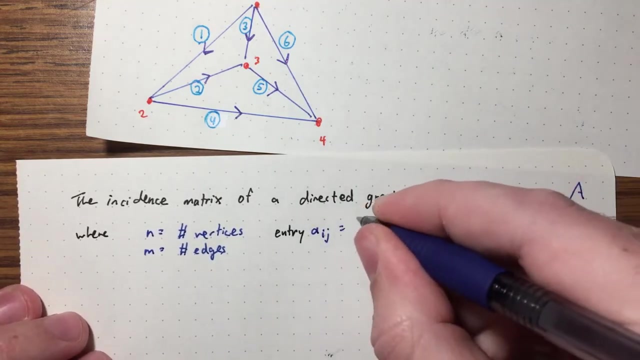 Okay, So, and then, yeah, what are the entries going to be? The entries? so yeah, let's say the entry A, I, J, And, remember, this means the ith row and the jth column. So it's going to be either a minus one, a one or a zero. 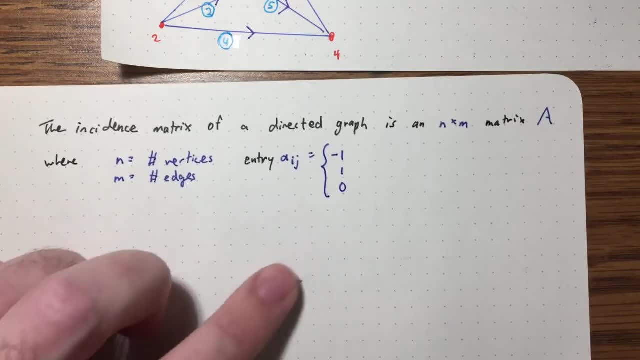 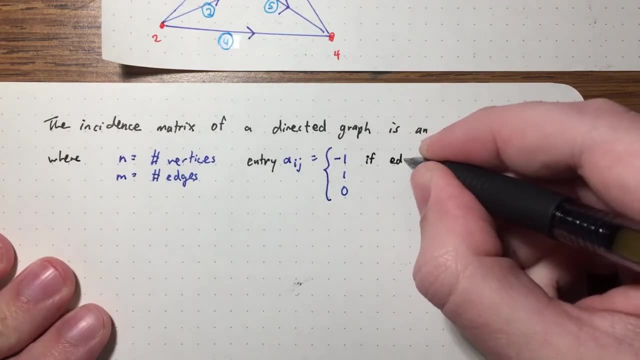 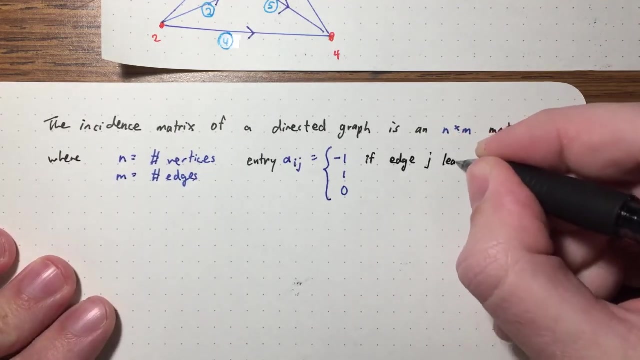 So this matrix is going to have a lot of structure. It's just going to be minus ones, ones and zeros. It's a minus one if edge- let me get this right- Yeah, if edge J leaves vertex I. I think that's what I want. 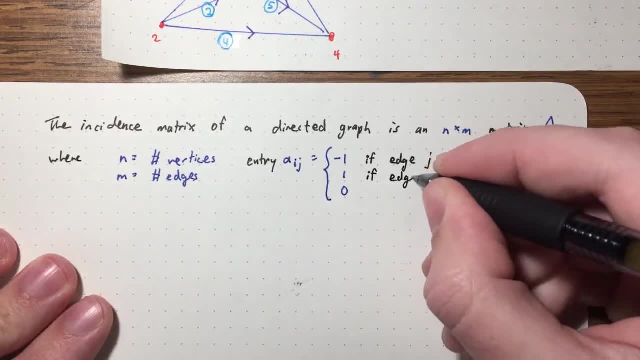 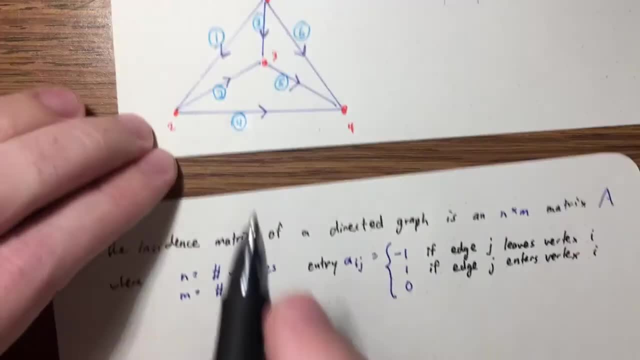 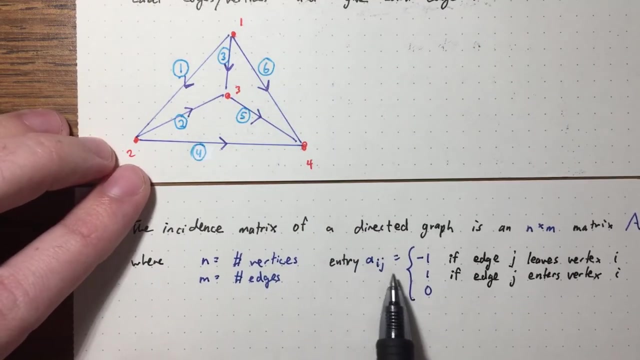 And then it'll be a plus one. if edge J enters vertex I, All right. So like, for example, vertex one, I see edge one leaving vertex one. So A one one should just be a minus one. It'll be a zero if edge J has nothing to do with vertex I. 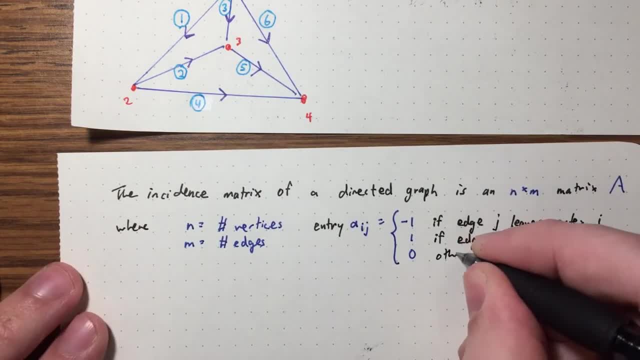 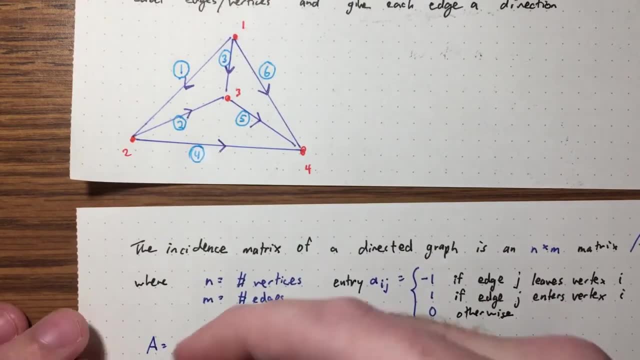 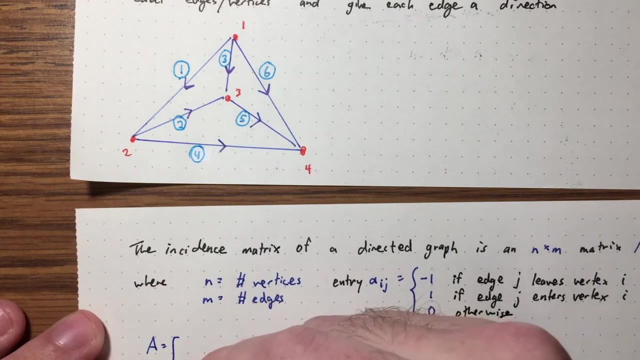 Right, So zero, otherwise. So let's do an example. We'll do our tetrahedral graph. So A is going to have how many rows? It'll have four rows, because my tetrahedron has four vertices. All right, In fact, let me leave some room to label these. 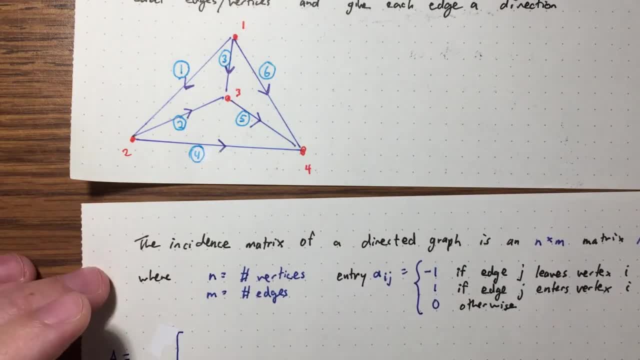 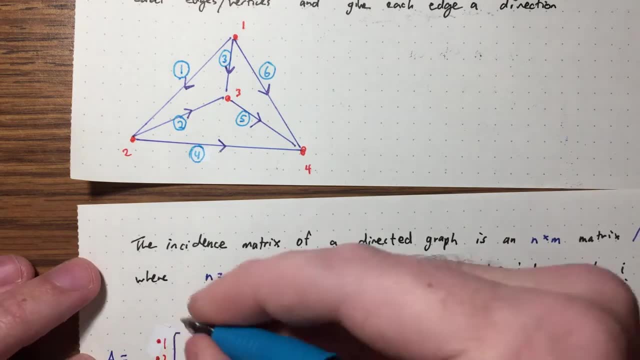 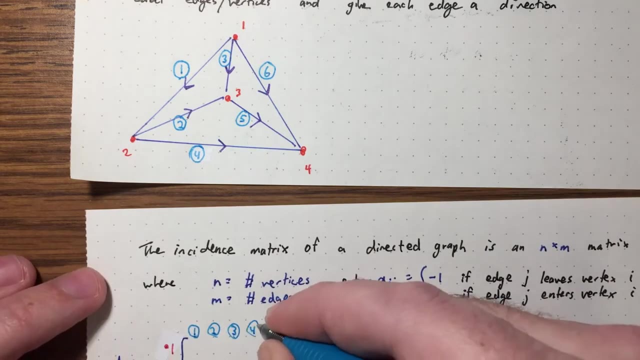 So this is my matrix A And I'm thinking of these as the vertices. So this is vertex one, vertex two, vertex three, vertex four And I'm thinking of my columns as edges. So I've got edge one, edge two, edge three, edge four, edge five and edge six. 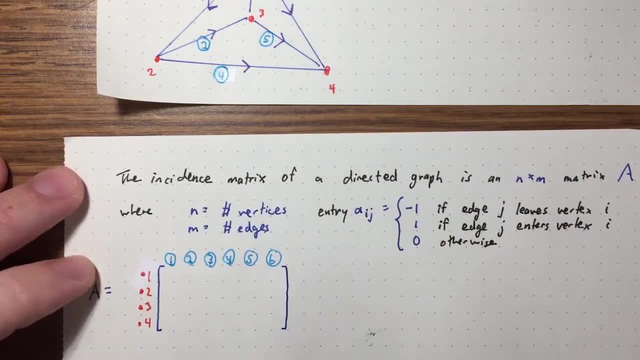 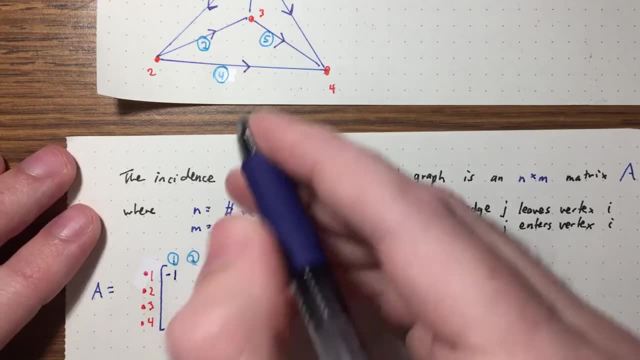 Okay, I'm looking at vertex one. I see edge one leaving it, So that's going to be a minus one. Edge two is way down here. It's not even connected to vertex one, So that's going to be a zero. 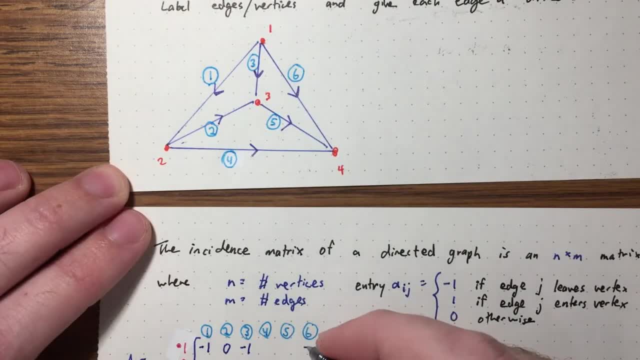 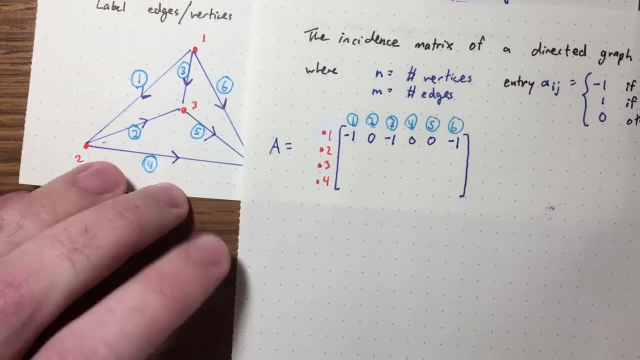 But I'm going to put a minus one because I see edge three leaving vertex one. I'm going to put a minus one there, And these two are going to be zeros, All right, So let's put this right next to there. How about this row? 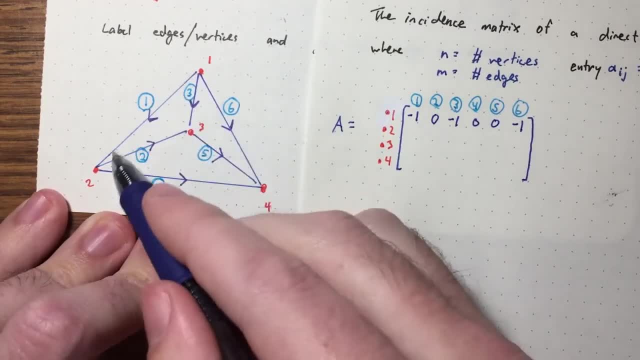 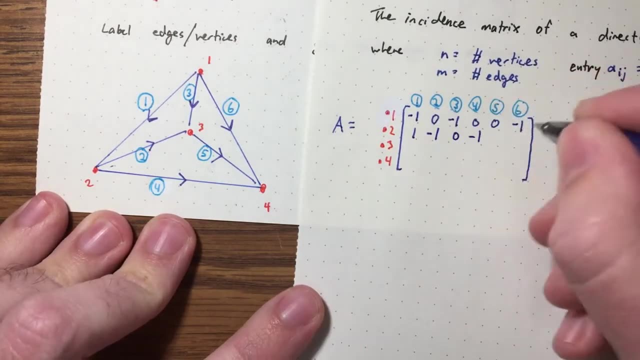 I'm looking at vertex two And I see edge one coming into it, So I'm going to put a one And then edge two is leaving. I'll put a minus one And edge four is leaving And the others are zeros. 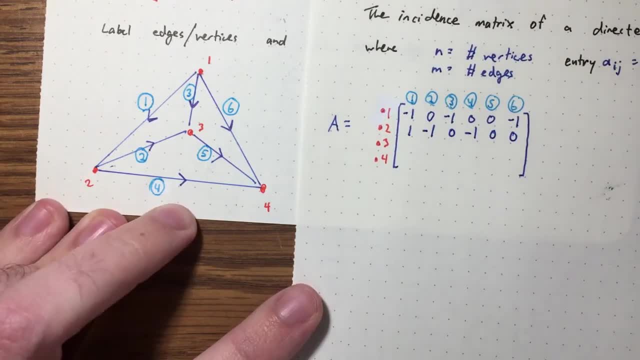 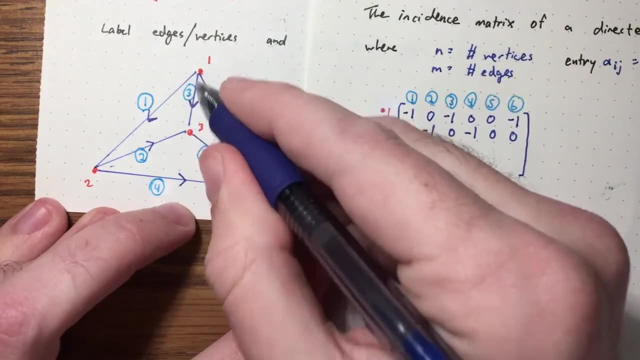 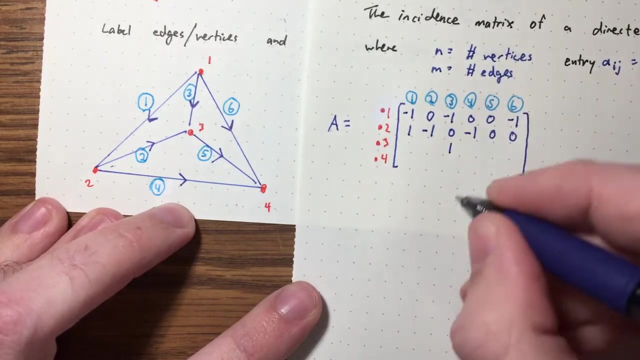 And then this one is a: See if you can finish the matrix yourself. by the way, Pause the video, Try to finish it yourself. Okay, So now for vertex three. Edge three is coming in. All right, I need a one there. 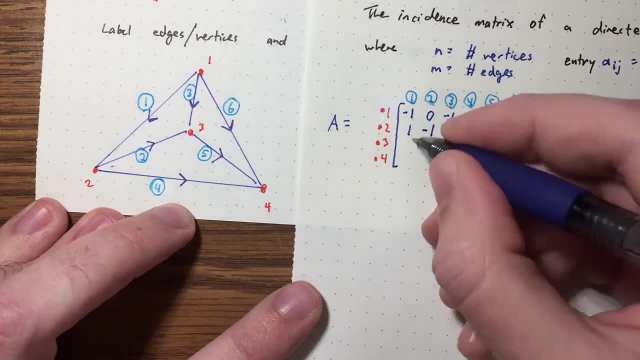 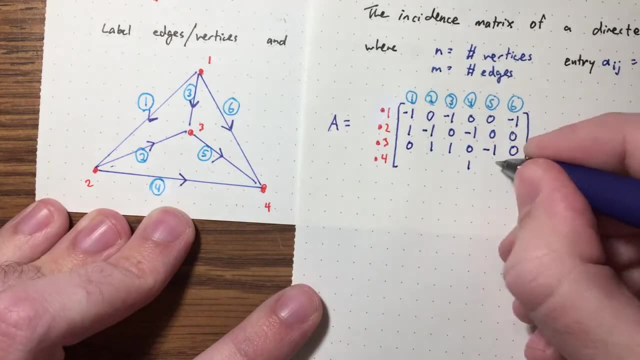 Edge two is also coming in, But then edge five is leaving. And how about vertex four? I see four, five and six are all coming in. The other ones are going to be zeros. Nice, So we just formed the incidence matrix of this graph. 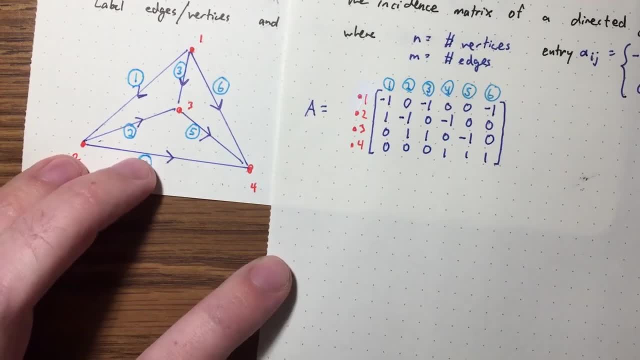 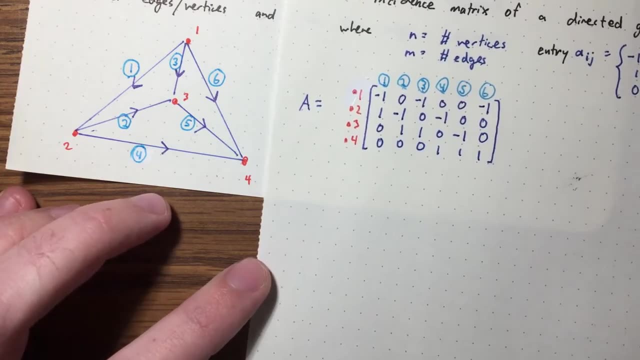 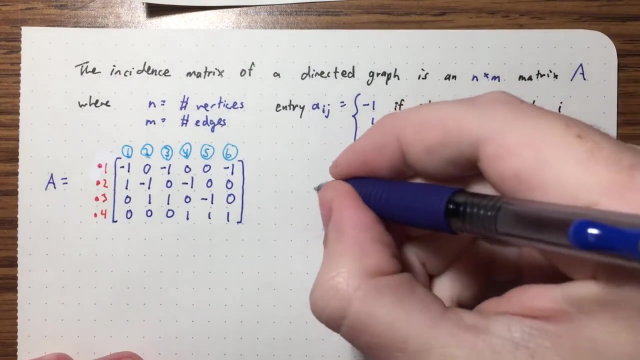 That's what this is called, And the idea is we want to sort of apply the rank nullity theorem to this matrix. This is the matrix that we want, But you know, it's often also useful to consider A transpose when we're dealing with the incidence matrix. 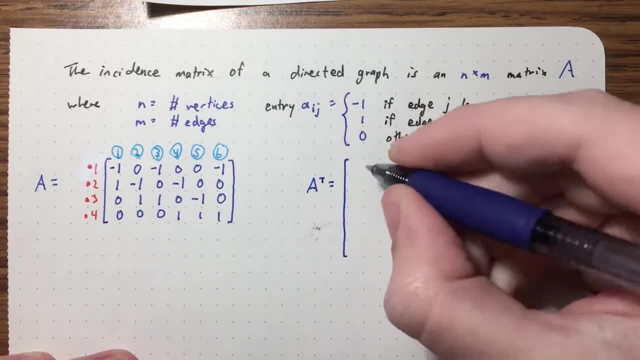 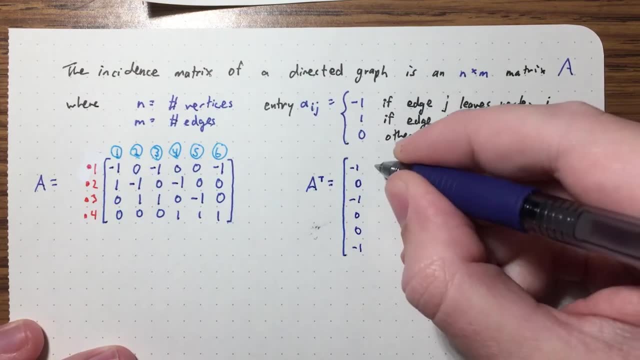 So what's A transpose going to look like? I'm just going to write it down here. Okay, The first column will be the first row of this: one One minus one, zero minus one, zero, zero And zero one one. 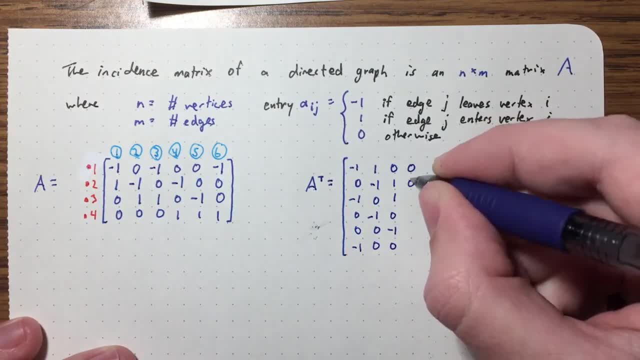 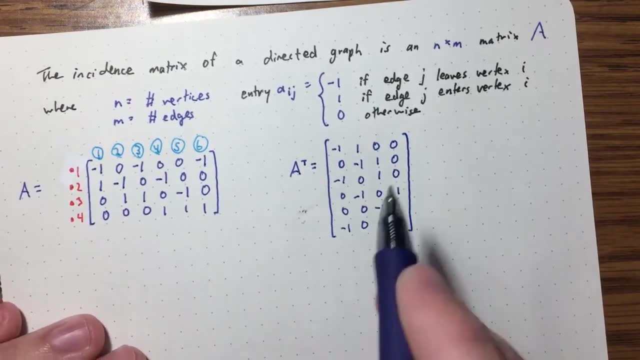 Zero minus one zero, One minus one zero, And then finally zero, zero, zero, One, one one, And that's A transpose. This reflected A along the diagonal, Whereas the rows of A became the columns of A transpose. 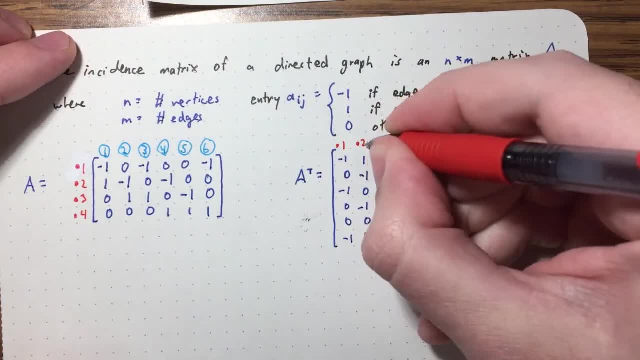 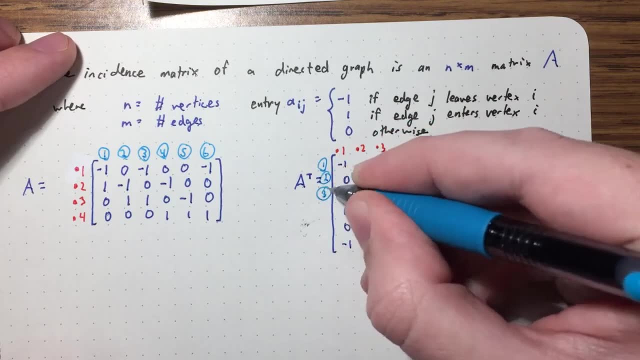 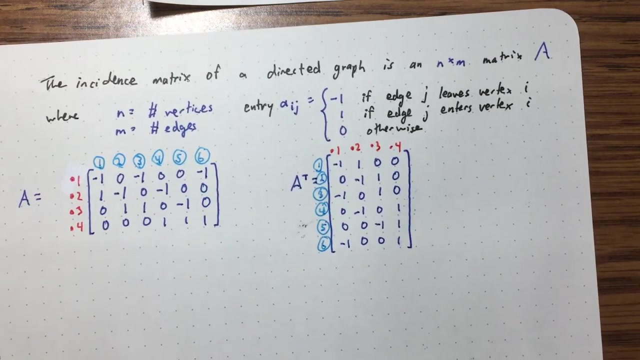 Okay, And in A transpose now my columns represent the vertices And my rows represent the edges, So I just like to have both these matrices written down. So we're about to compute some subspaces associated with these matrices. Okay, So first thing I'd like to do is I'd actually like to find the rank of A. 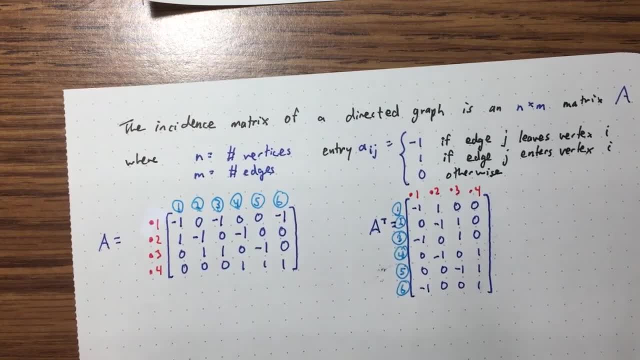 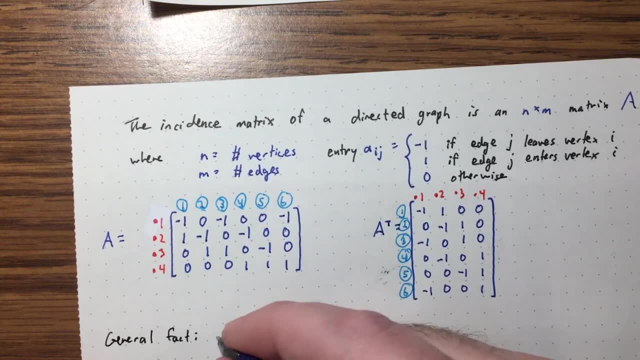 But there's a general fact actually. So here's a general fact. This is not just true for these matrices, but it's true for all matrices. I forgot whether we talked about this, but the rank of a matrix is the same as the rank of its transpose. 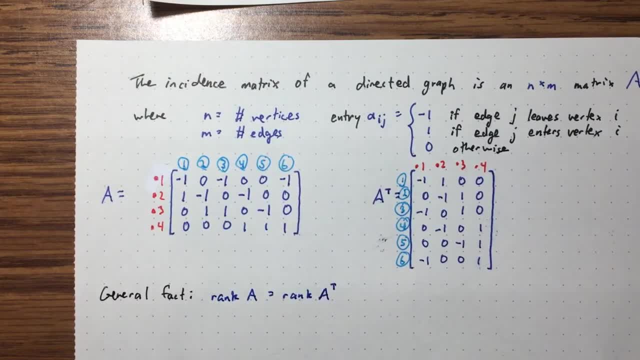 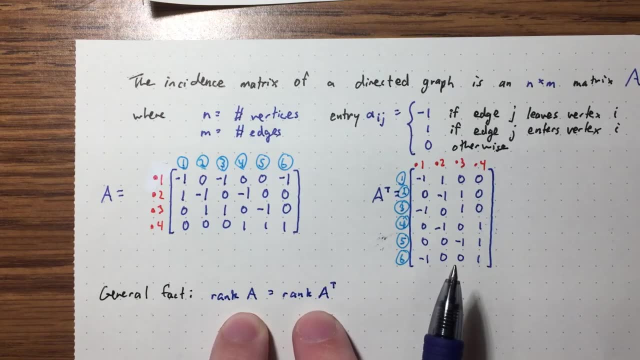 And that's because they're both going to have the same number of pivots, So we have the same number of pivot columns. I'm not saying the column space of A is the same, Same as the column space of A. transpose, Of course not, right. 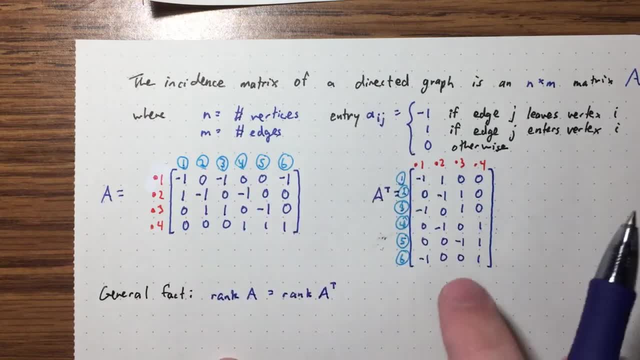 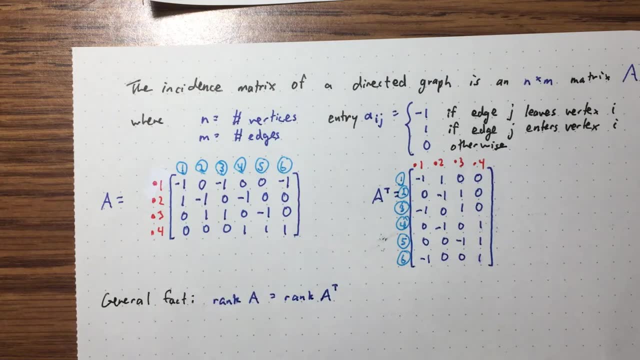 Because here the column space is in R4. And here the column space is in R6. It can't be the same, But they have the same dimension. That's because the dimension of the column space is related to pivots- How many pivots there are. 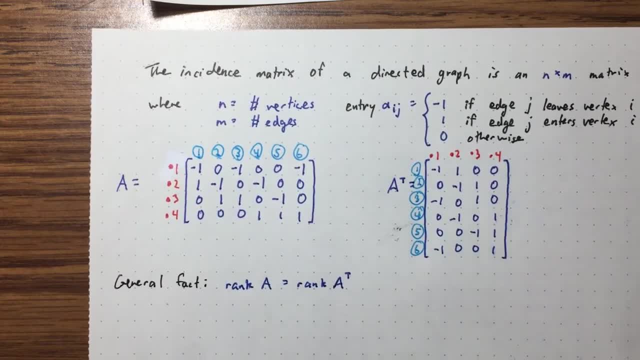 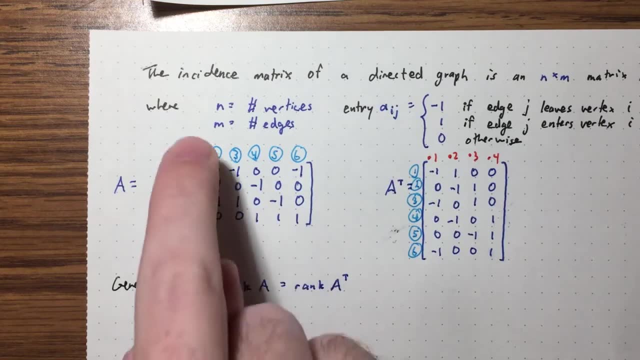 And the number of pivots of a matrix is equal to the number of pivots of its transpose. So if I wanted to find the rank of A, in other words how many linearly independent columns I have, I could instead do the same problem with A transpose. 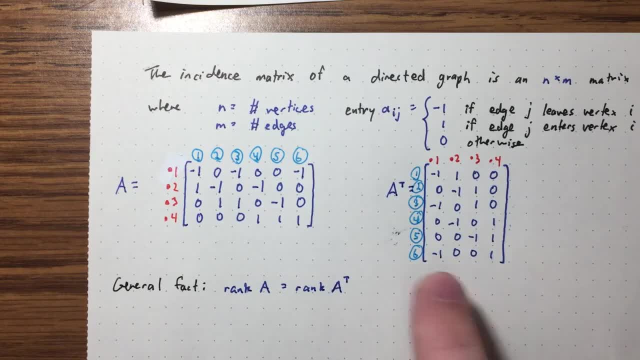 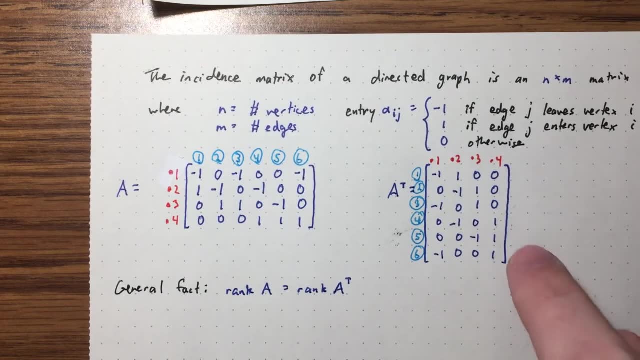 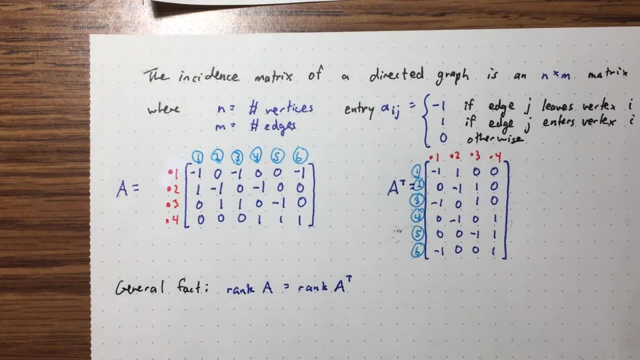 Which I don't know, maybe looks a little bit easier because I have four columns instead of six to deal with And by the rank nullity theorem we could instead try to find the null space of A transpose, And that's actually what I'd like to start off by doing. 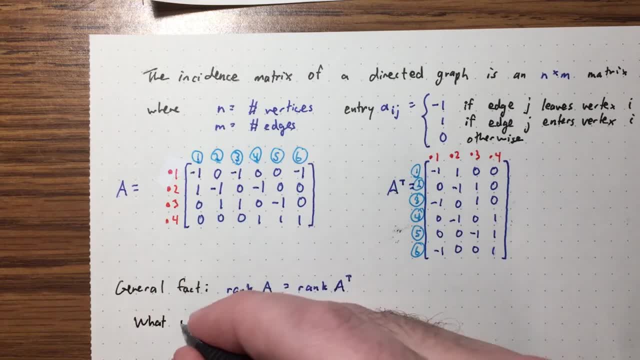 So what is? because, again, the number of columns here is going to be the rank plus the nullity. So I want to ask: what is the null space of A transpose? We're also going to look at the null space of A. 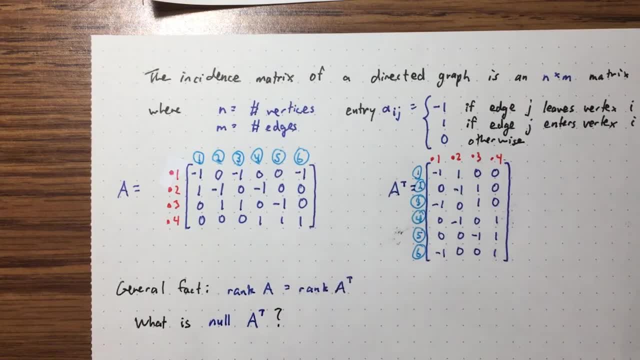 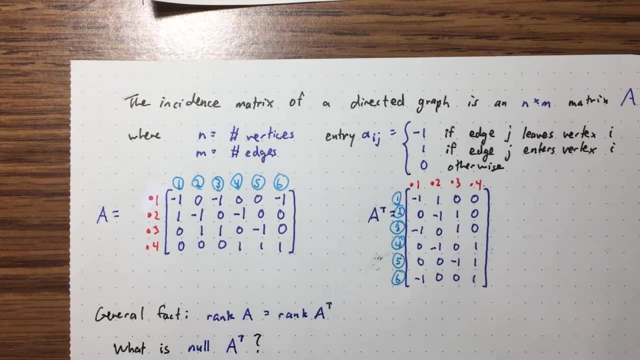 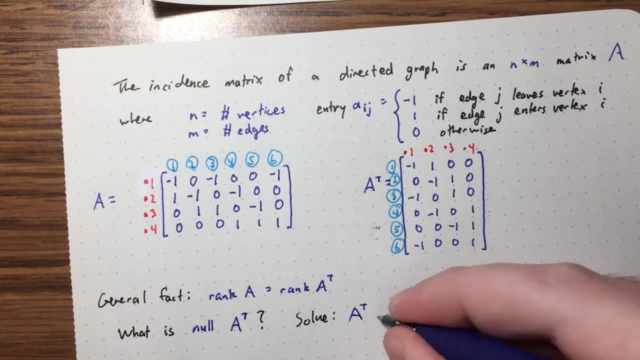 But I want to start with A transpose. Okay, What do we think? Well, how do we find the null space? We want to solve, as always. okay, we want to solve A transpose. X equals 0.. We want to solve this equation. 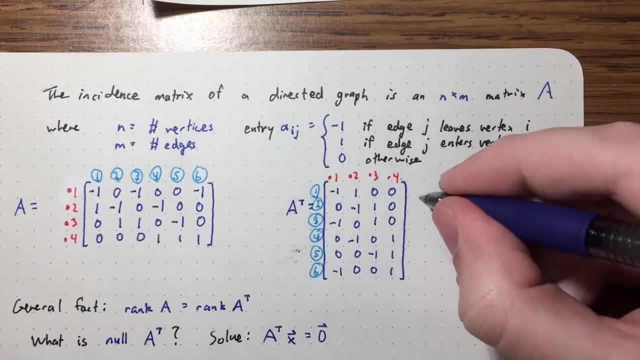 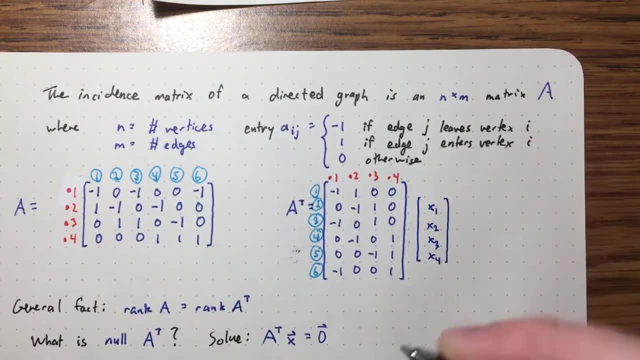 Find all the solutions. So is it okay if I write in a little Vector X here: X1, X2, X3, X4.. I don't want to copy down this matrix a bunch of times. I want to solve this equation. 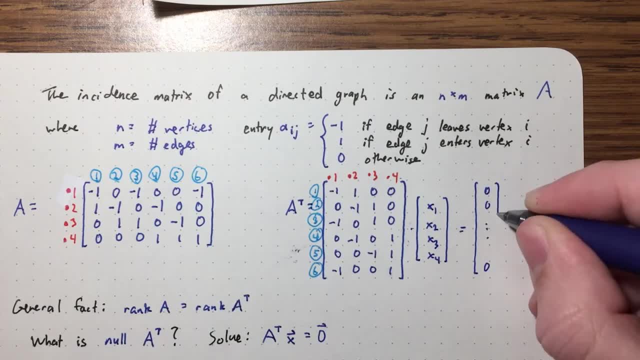 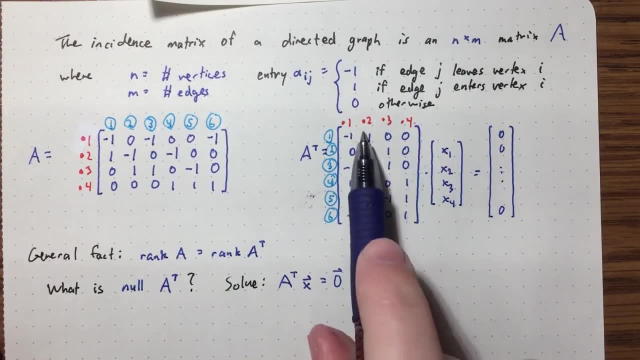 This equals 0.. Okay, Well, I mean, look at the rows of this matrix, right, There's a lot of structure. So what do we see in the rows of this matrix? There are only two numbers. There's a minus 1 and a 1.. 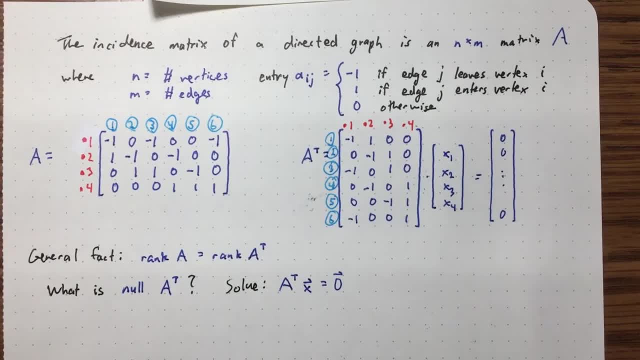 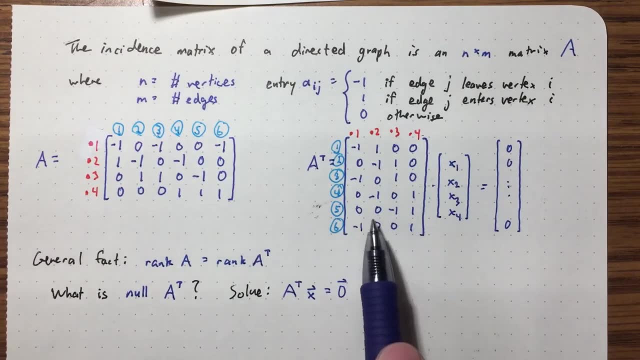 This is extremely common for matrices that come up in real life. There's often structure that you can exploit, And so here we see, there's only two numbers in each row that are non-zero: A 1 and a minus 1.. And well, why is that? 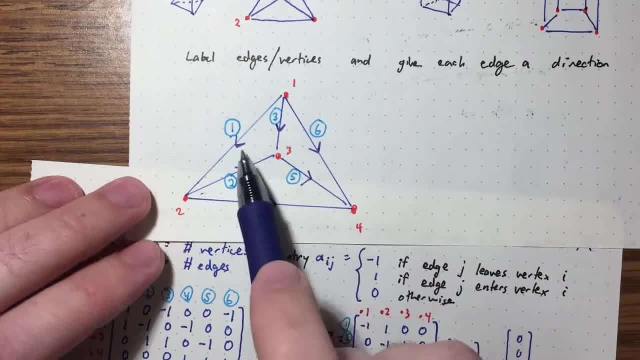 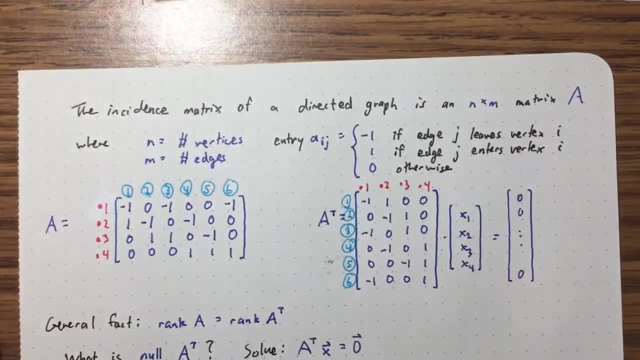 It's because for any edge right, it's going to come from some vertex and it's going to, you know, it's going to leave some vertex and it's going to enter some other vertex. So I should always see a 1 and a minus 1.. 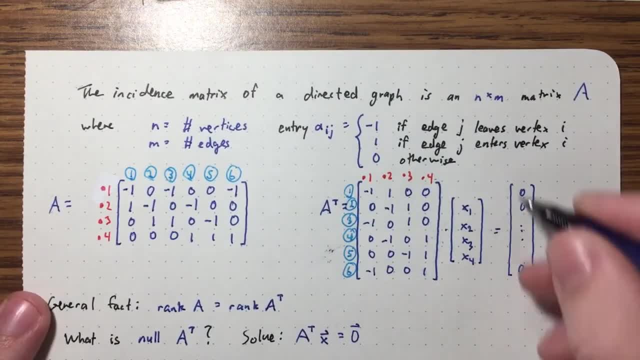 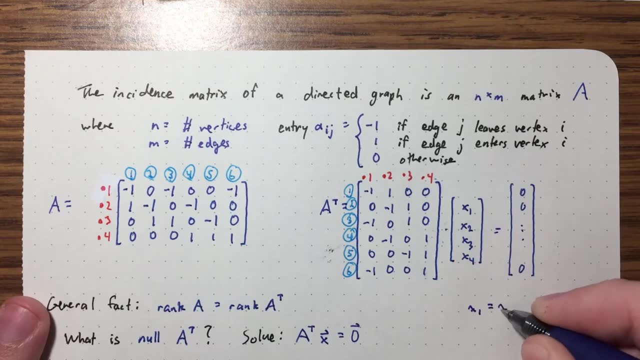 So if we start writing down the equations, what do we get? We just get like: I'll write down the first few rows. We get x1 equals x2, right Minus. x1 plus x2 equals 0.. So x1 equals x2.. 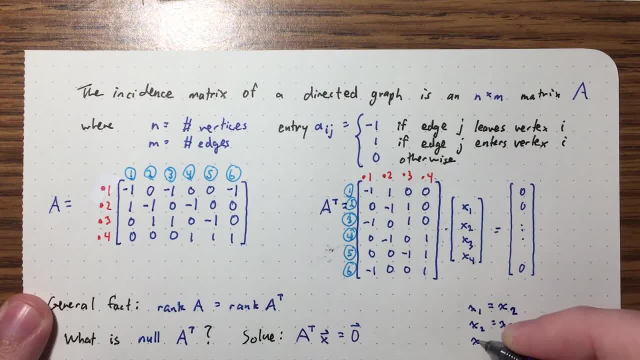 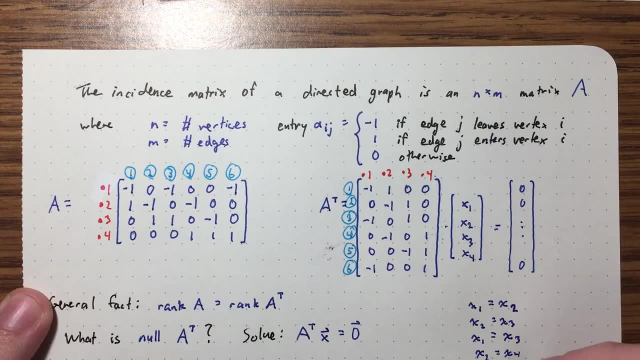 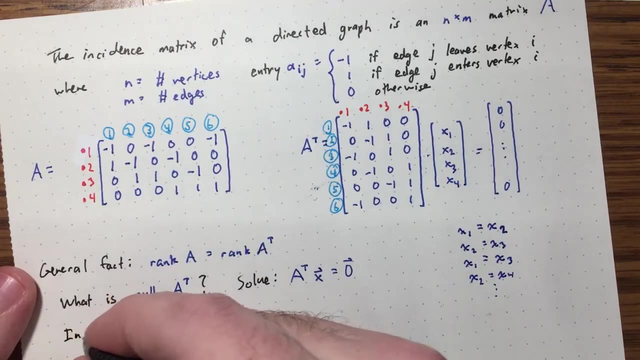 The second row tells me: x2 equals x3.. The third row tells me: x1 equals x3. That's redundant. We already knew that x2 equals x4. And so on, right, Okay, So in general, where are these coming from? 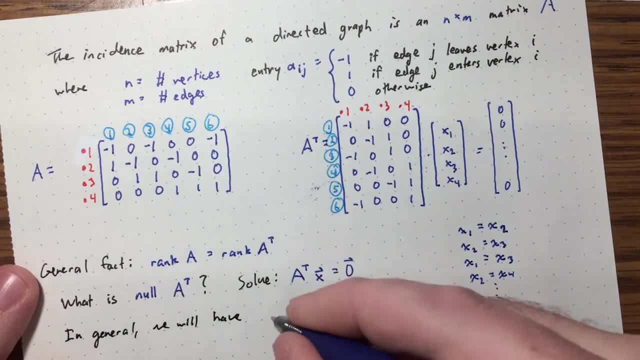 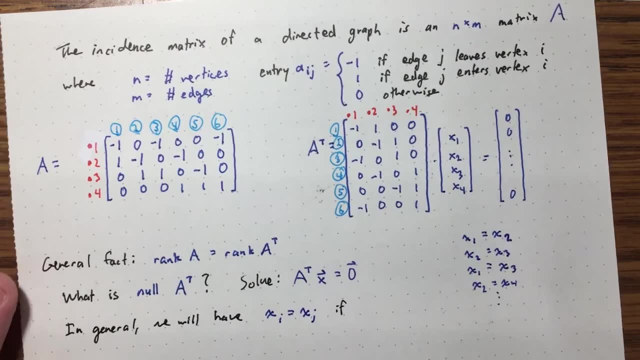 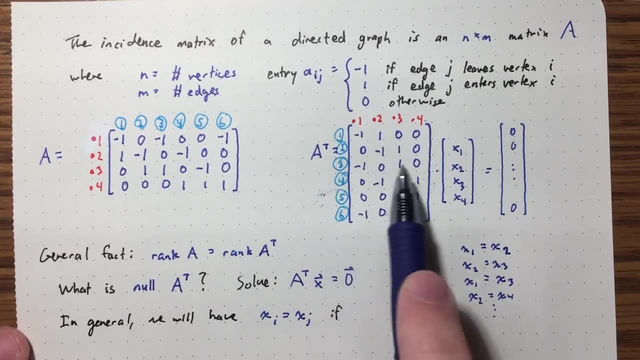 We will have xi equal to xj in our solution. if can you tell when we're going to have xi equal to xj, When are we going to get this relationship? Well, if there's some edge going from vertex i to vertex j, right. 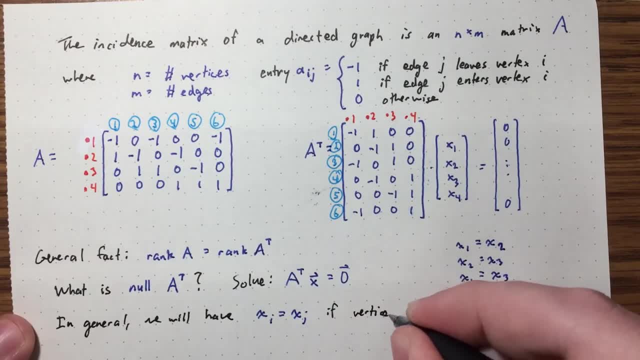 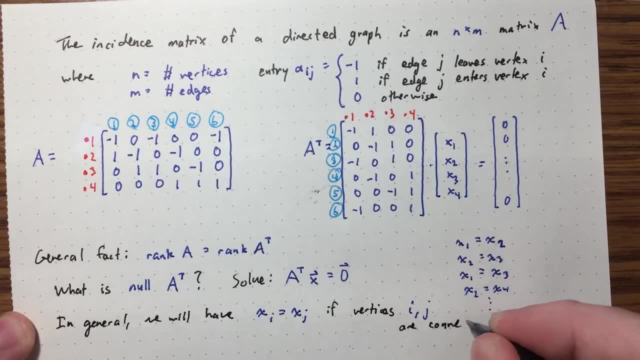 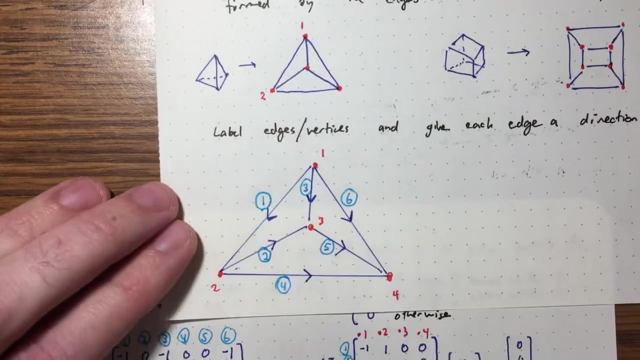 If vertices- one way we can say it- if vertices i and j are connected by some edge, By some edge, right? Okay, But you see, the graphs that we're starting with are connected graphs. Okay, So we can get from vertex 1 to vertex 3.. 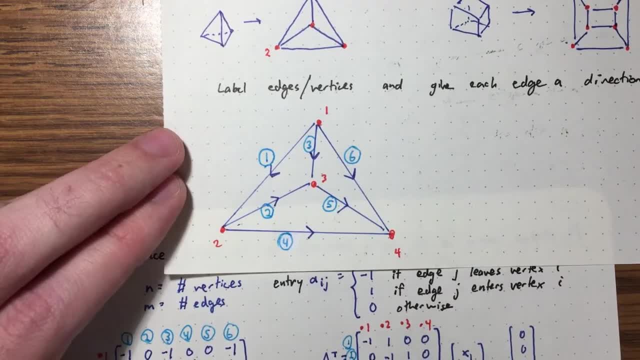 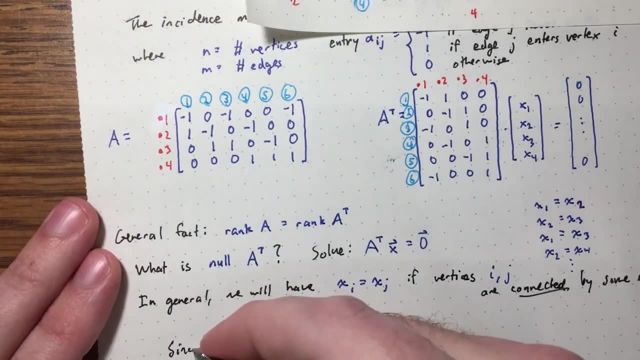 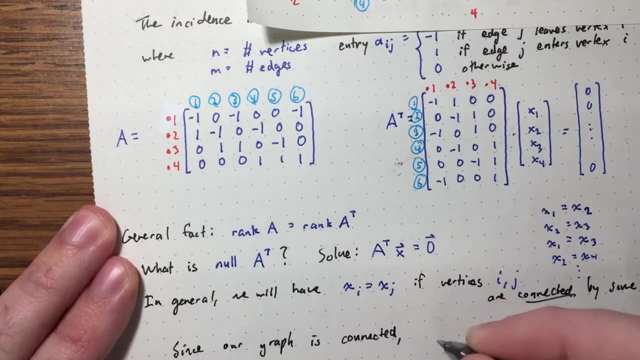 And we can get from vertex 3 to vertex 2.. So x1 has to equal x3,, which has to equal x2.. Which has to equal x4, because everything's connected. So, since our graph is connected, we have actually all of these x's being equal. 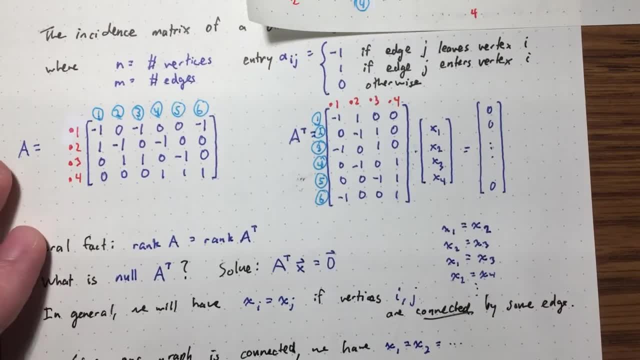 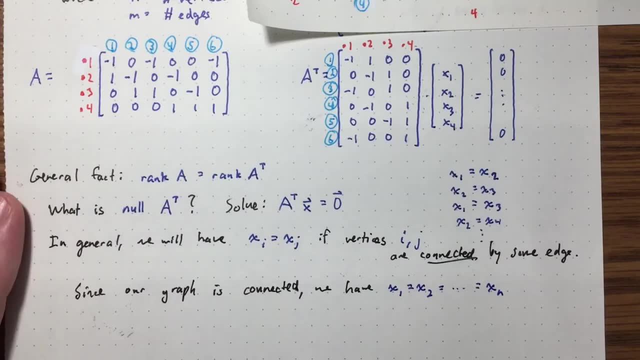 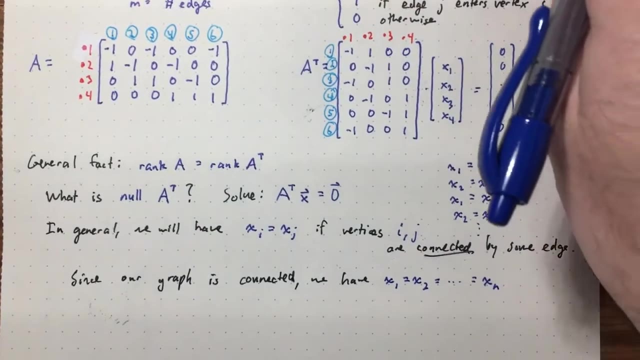 x1 equals, x2 equals, etc. All the way up to well. in general, it will be xn, Right? In our example, it's just four vertices. Okay, So what's the null space? Well, notice that we're free to pick one of these variables. 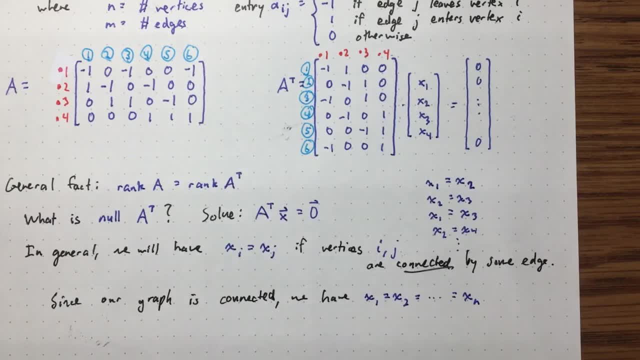 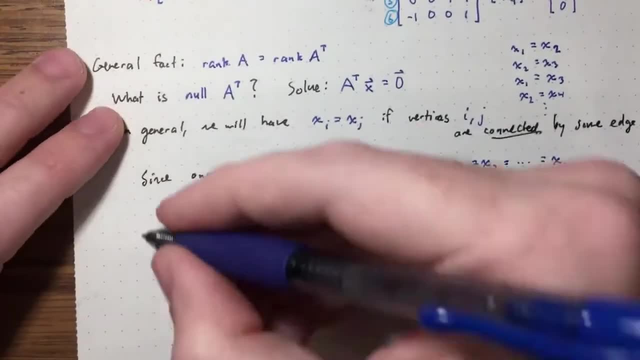 Right. So, for example, we can pick x1 to be whatever we want, But then, as soon as we pick x1, all the other ones have to be the same number, Right? So we have. this is our solution: x1,, x2, all the way down to xn. 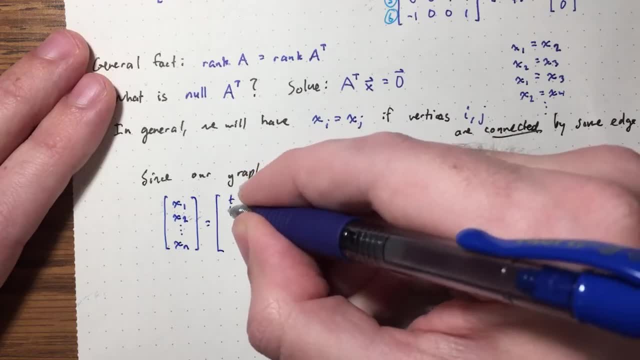 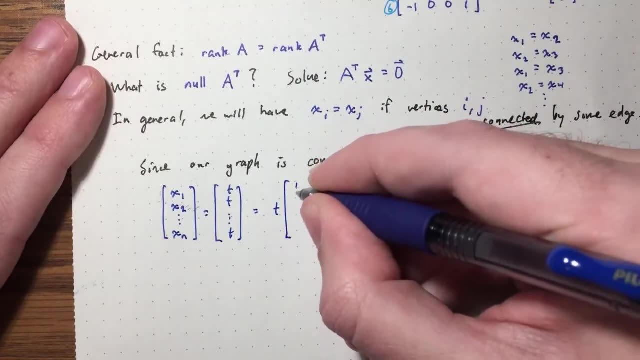 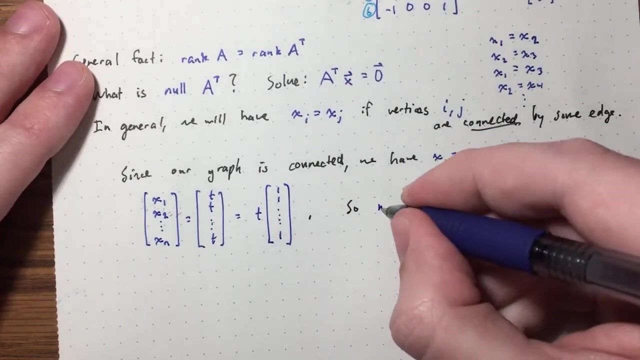 Is t, t, t for any number t that we want. We can rewrite this as t times 1, 1, 1, 1, 1, 1, 1.. Okay, So the null space is actually just spanned by. 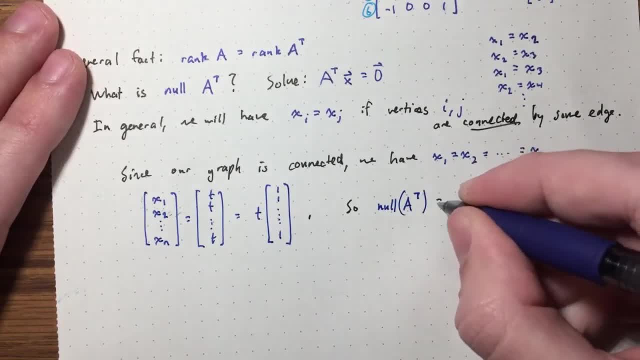 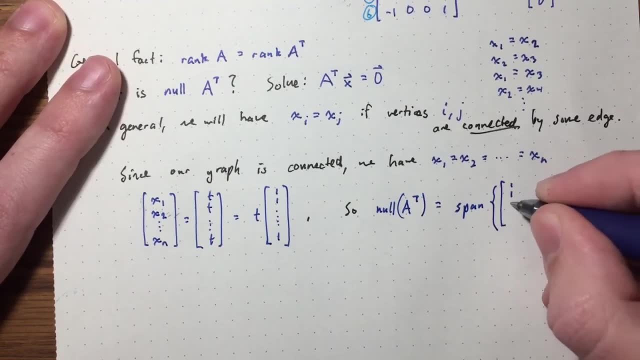 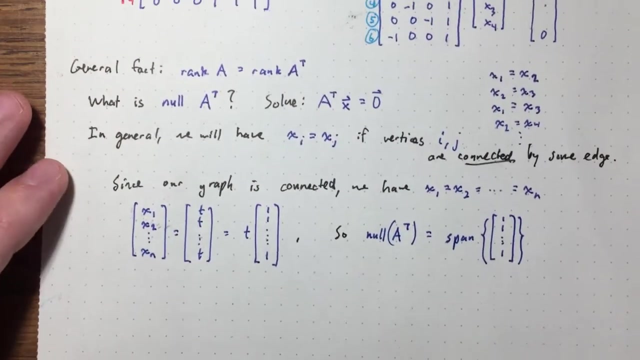 null space of A transpose is: it's just spanned by the vector 1,, 1,, 1.. All ones. This is in general for any of these polyhedral graphs. Okay, So in our example it will be four ones. 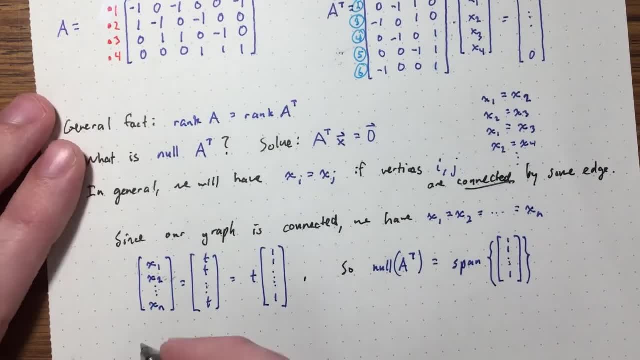 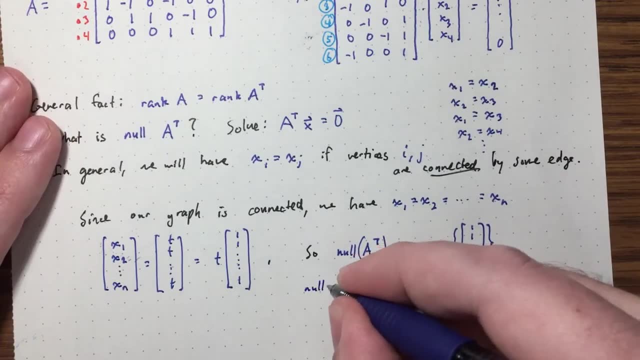 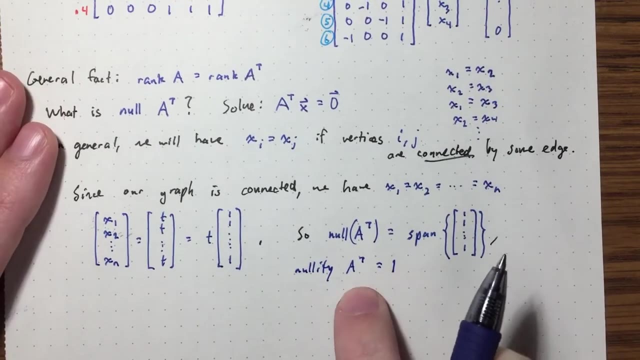 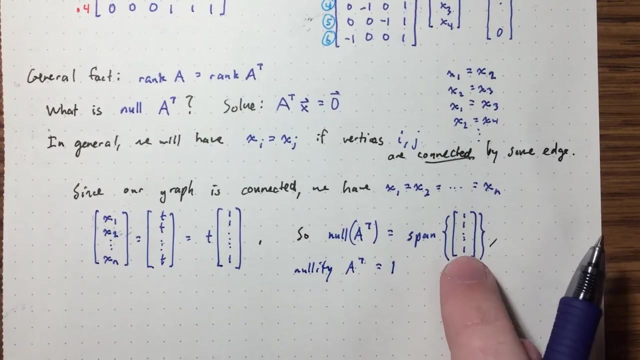 Okay, So what's the nullity? So the nullity of A transpose is 1.. Right, Because, again, what does the nullity mean? Right, It's the dimension of the null space. Okay, But we saw that the null space is spanned by one vector. 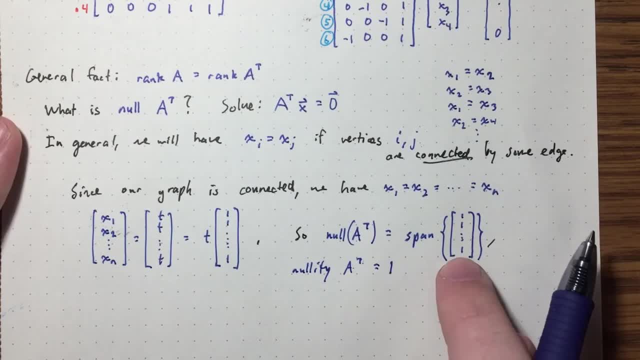 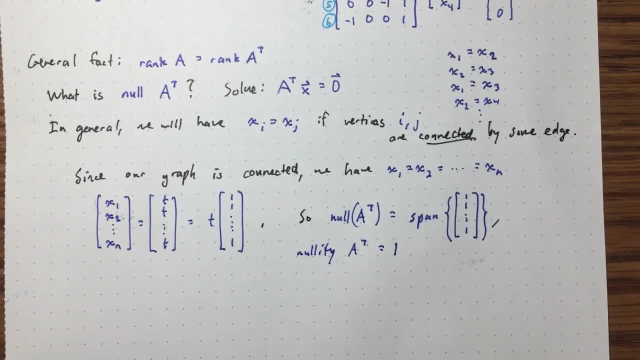 So it has a this: 1, 1,, 1, 1, 1 is a basis for the null space. Okay, So there's only one element in a basis, So the dimension of the null space is 1 in this example. 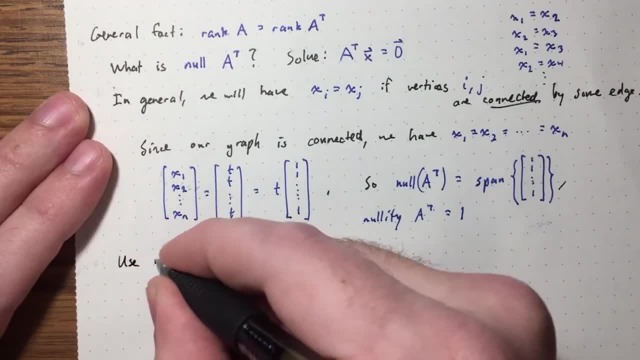 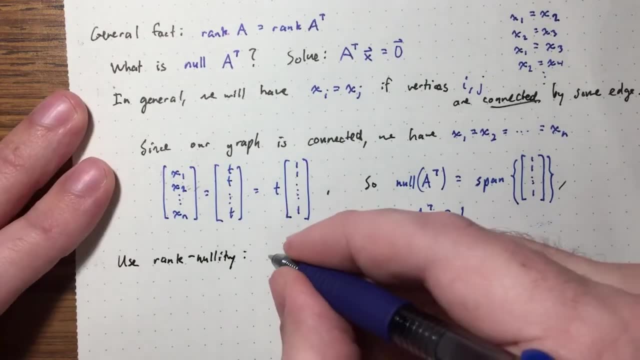 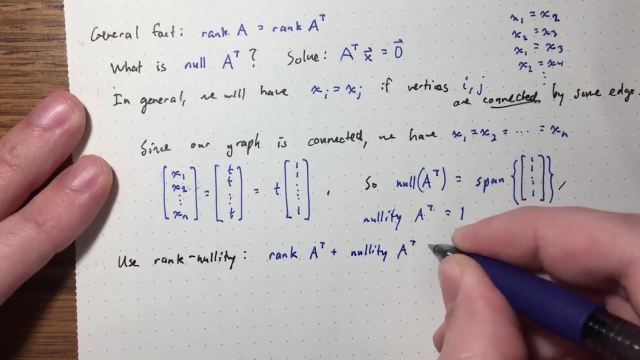 Okay, Now let's use rank nullity for the first time. We're going to use it again, But we'll use rank nullity for the first time. We know that the rank of A transpose plus the nullity of A transpose equals 4.. 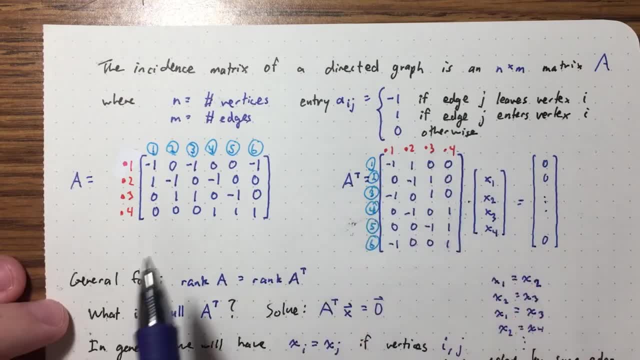 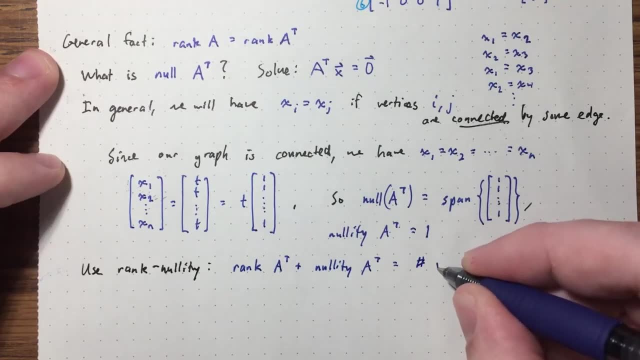 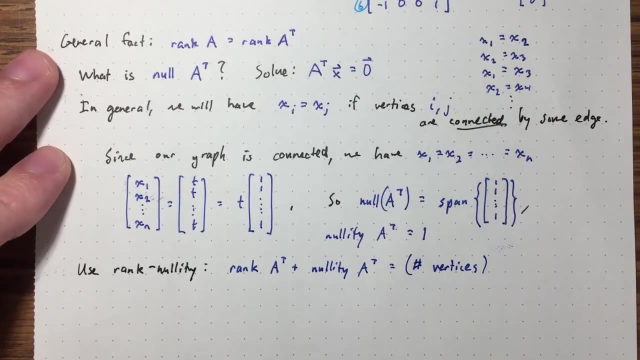 But instead of 4,. I'm going to write down what it is in general, Like: what are the number of columns? It's the number of vertices. Okay, So it's the number of vertices, Right, But we just showed that the nullity is 1.. 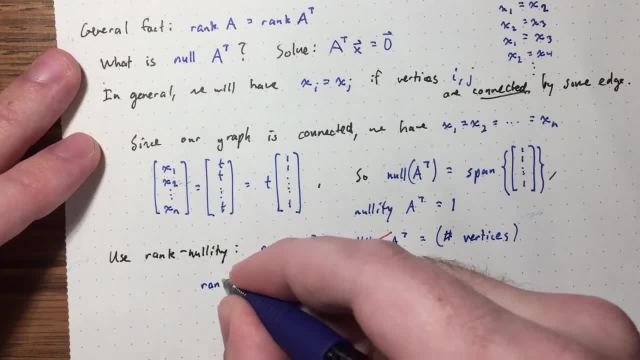 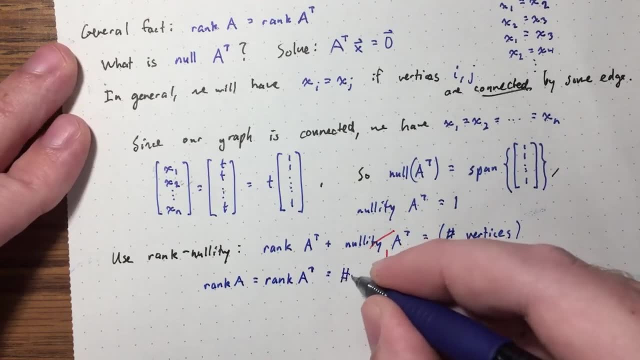 So the rank of A transpose, which is actually the same as the rank of A. So let's use that So we know the rank of A is the same as the rank of A transpose, which is the number of vertices minus 1.. 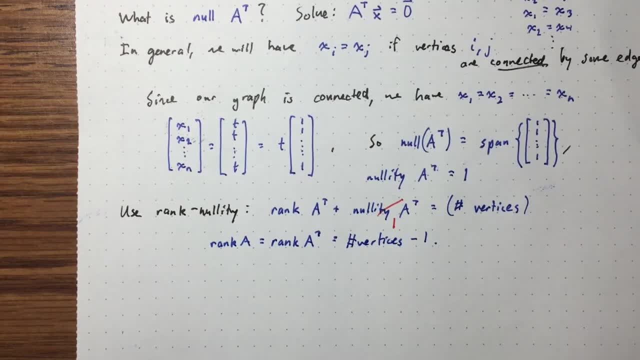 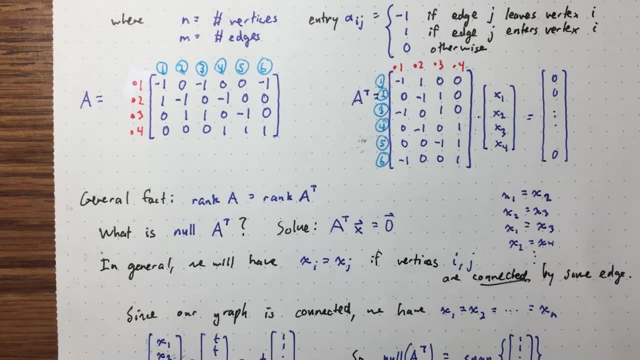 Okay, Very cool. So that's the first thing we wanted to figure out: What's the rank of A? If we're going to use rank nullity, let's also try to figure out what the nullity of A is. Now we'll write down the rank nullity theorem for this matrix A. 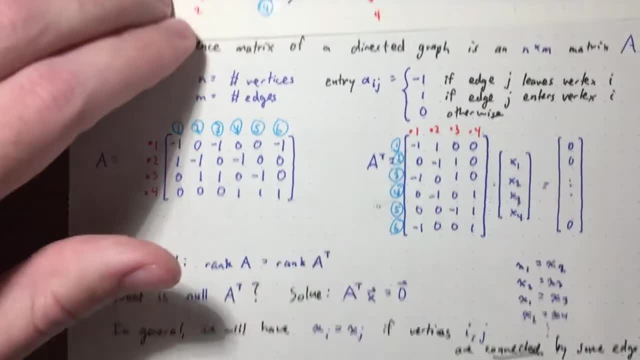 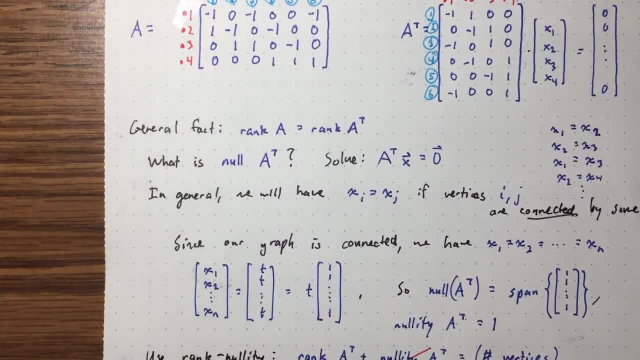 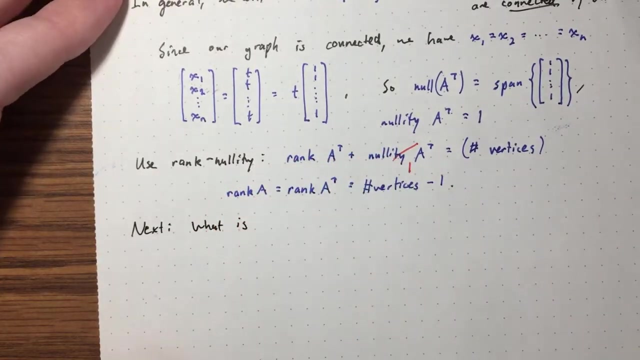 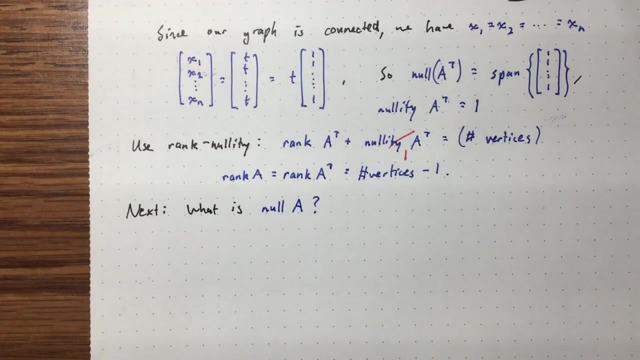 But we know that the rank of this matrix is the number of vertices in our polyhedron minus 1.. So next, what is the nullity of A? Let's start with the null space. What's the null space of A? We know the rank of A. 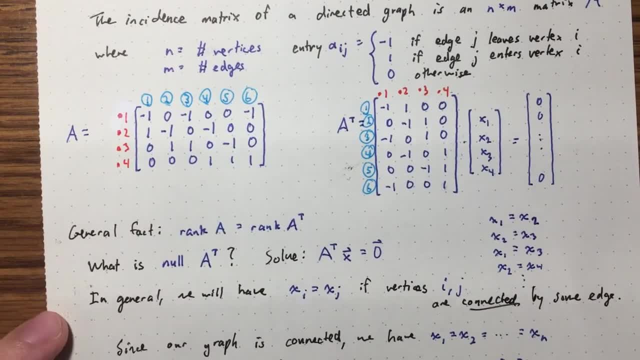 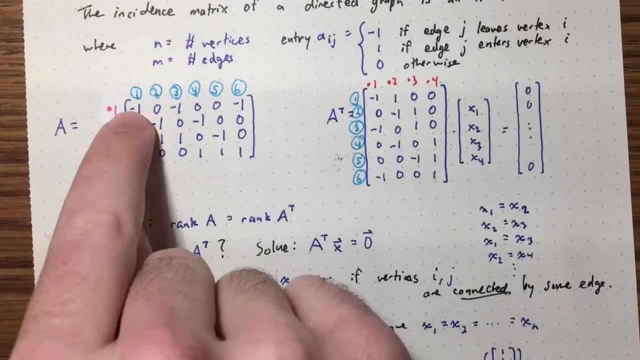 Well, by rank nullity theorem, we know what it should be. Do we know what it should be? It should be the number of edges minus this, Because the rank of A plus the nullity of A should equal the number of edges. 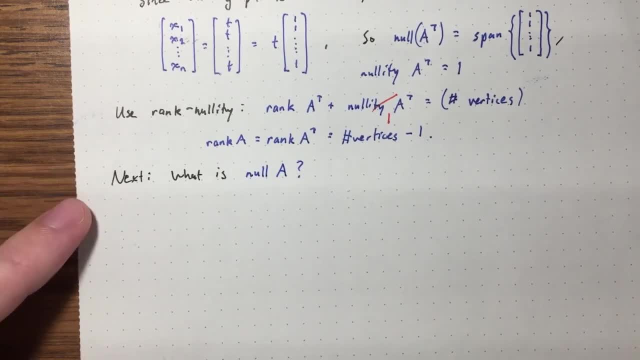 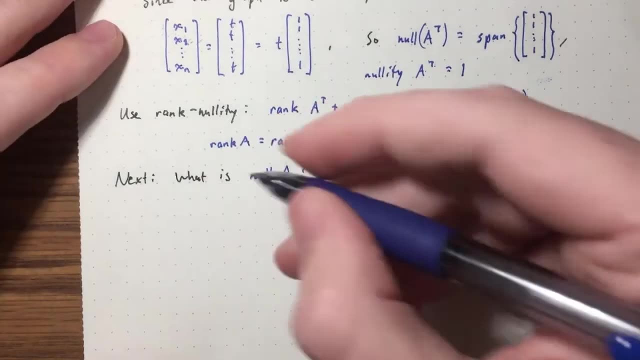 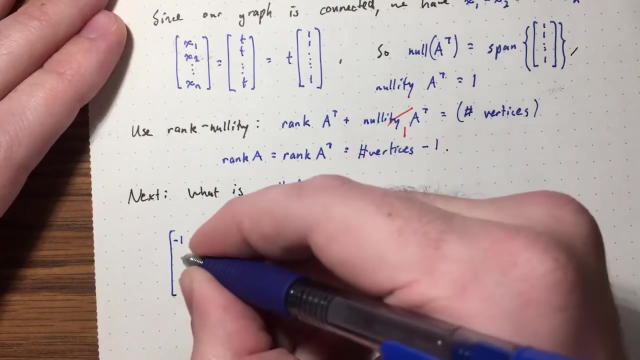 But let's see if we can understand the nullity of A in terms of things that are related to our polyhedron. Okay, Can I write down the matrix one more time, maybe. So I'm going to write down our matrix A. I want to solve the equation: AX equals 0.. 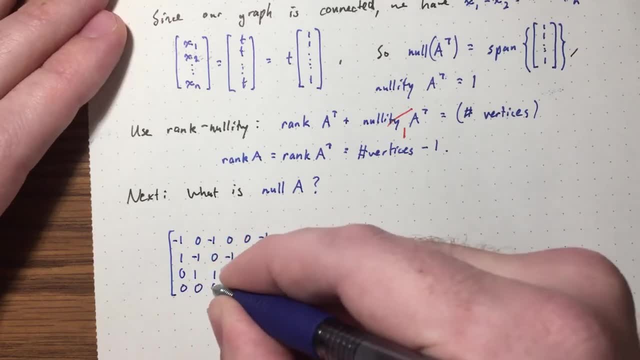 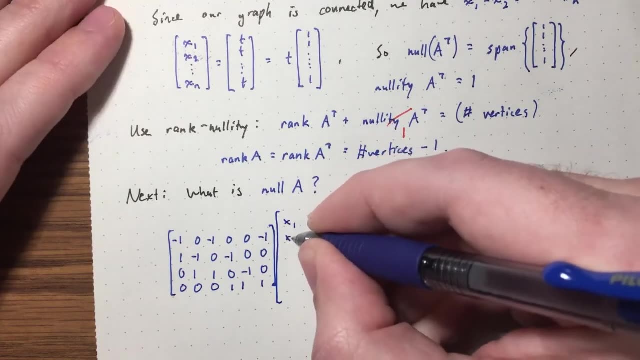 0, 1, 1, 0, minus 1, 0, 0, 0, 0, 1, 1, 1.. And I'm going to multiply it by a vector of X1, X2,, dot, dot, dot, down to X6 in our example. 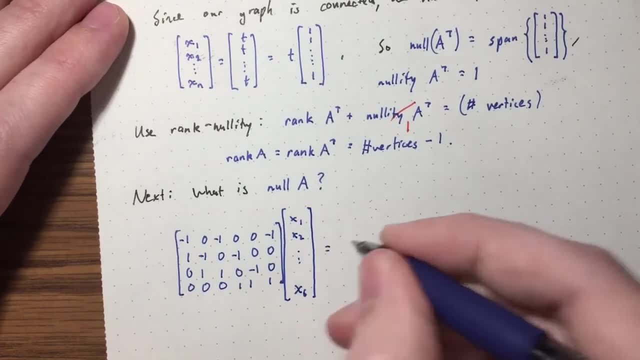 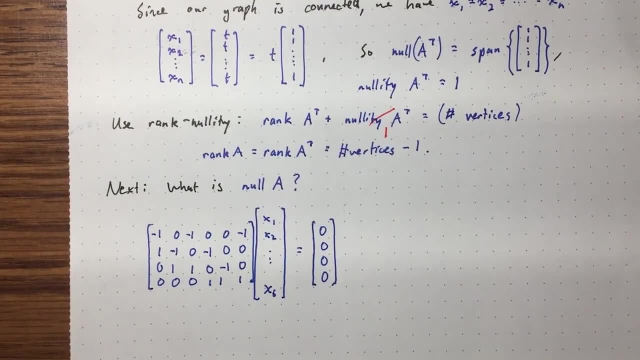 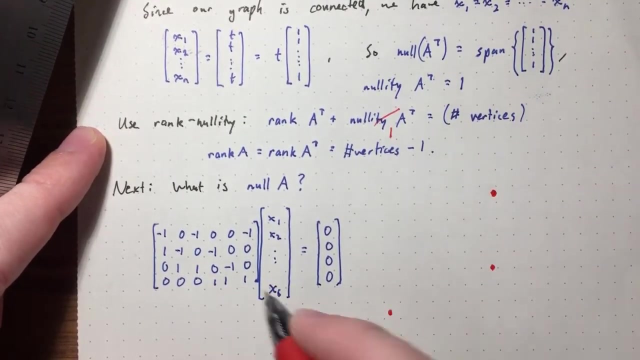 That 6 is just M, It's the number of edges, And this is going to equal all zeros. Okay, So I'd actually like to copy down my graph once more, Because it turns out, vectors in the null space here are going to have a really beautiful geometric meaning. 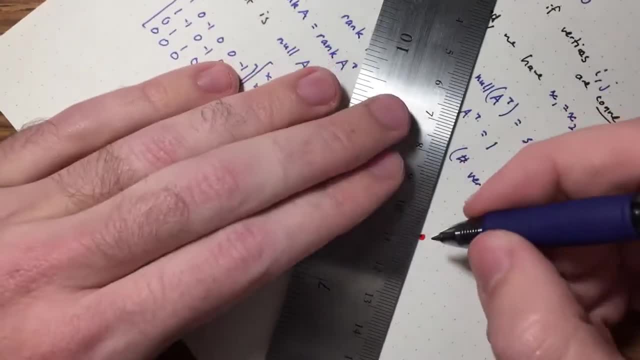 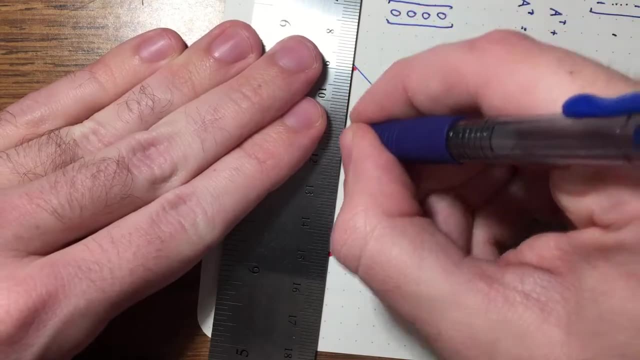 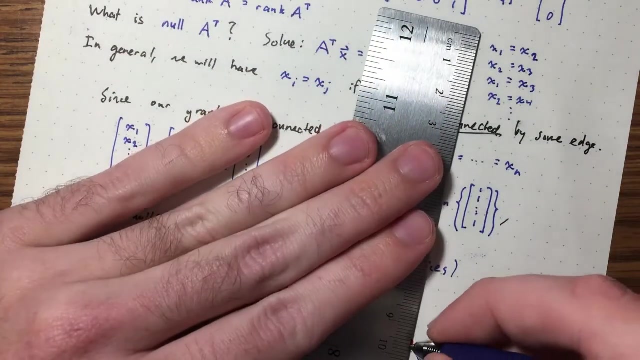 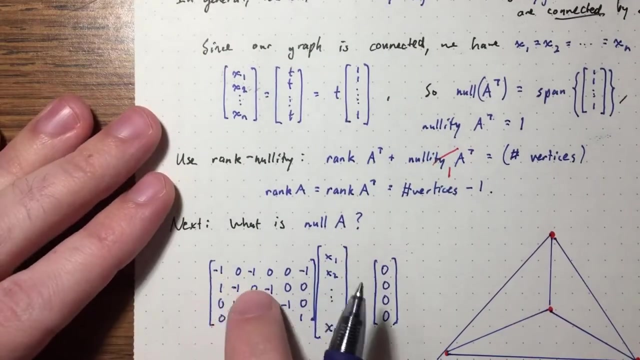 Okay, Um, So I'm going to do my tetrahedral graph And how do, yeah, how do we think about these vectors in the null space? Well, they're associated to, so they're sort of the weights for the column vectors. 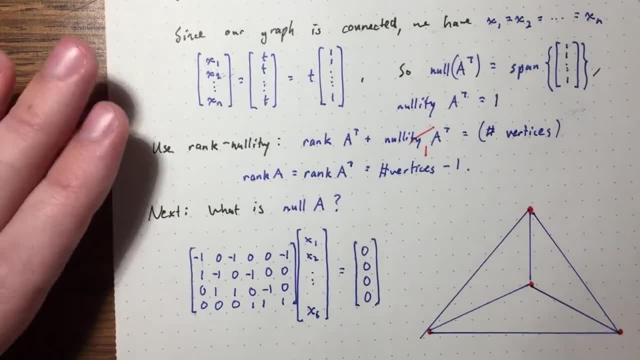 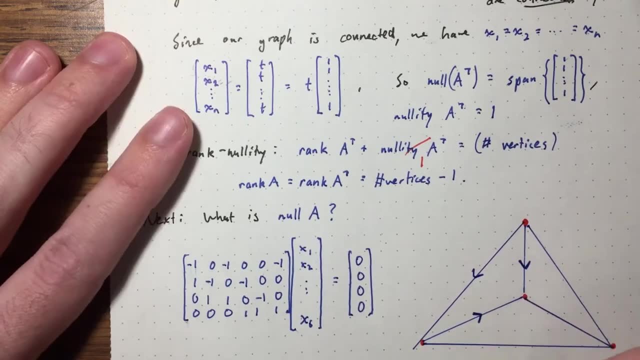 Right, So for each edge I have a column Um, So To each edge I'm sort of associating a weight: X1, X2,, X3,, X4,, X5, X6.. Okay, So Um. 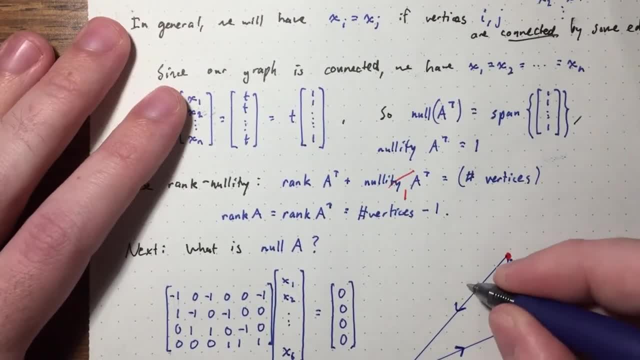 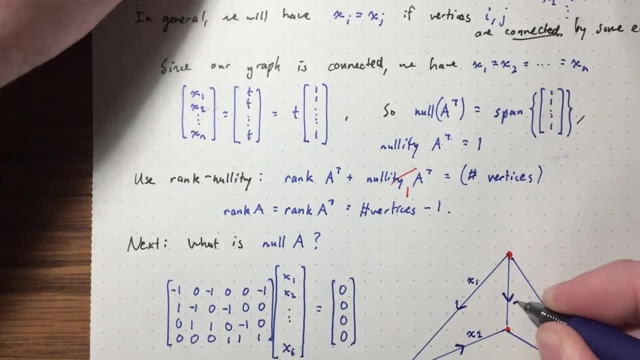 Yeah, X1 is here. X2 is here. Um, Which one is? 3 again, It's this one. Just copying down my graph from before, This is X4., X5. And X6.. And then here's our vertex 1, 2.. 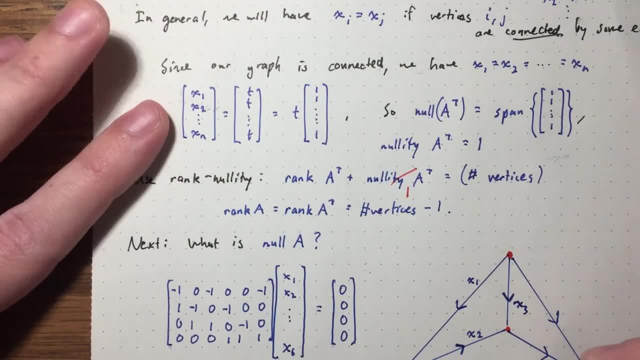 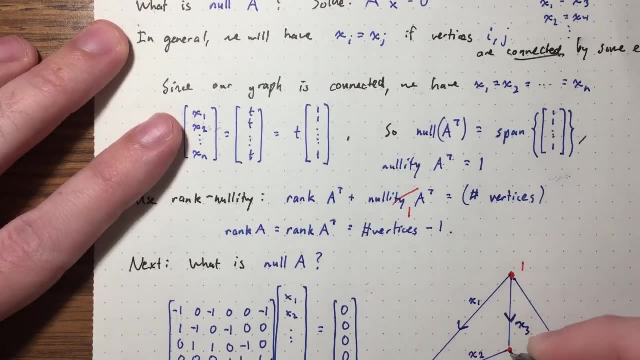 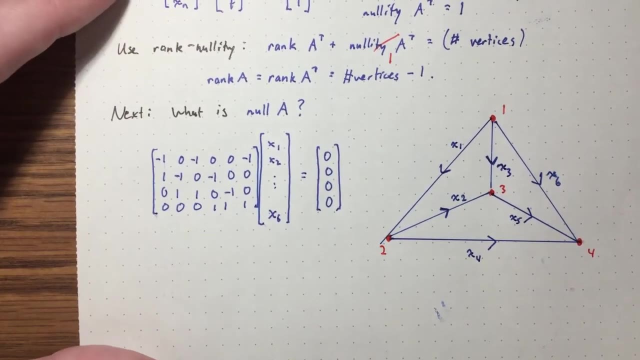 Uh, 3.. X4., X5., X6., X7., X8., X9., X11., X12., X13., X14., X15., X16., X17., X18., X19., X20.. 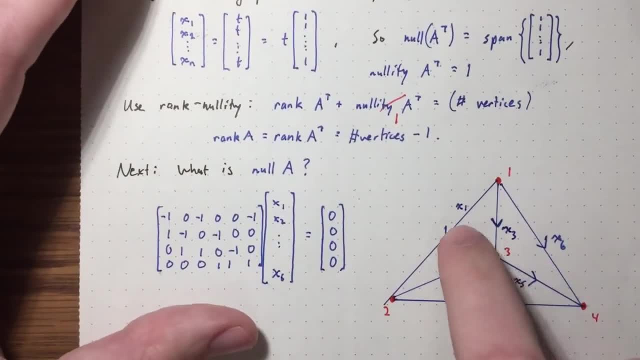 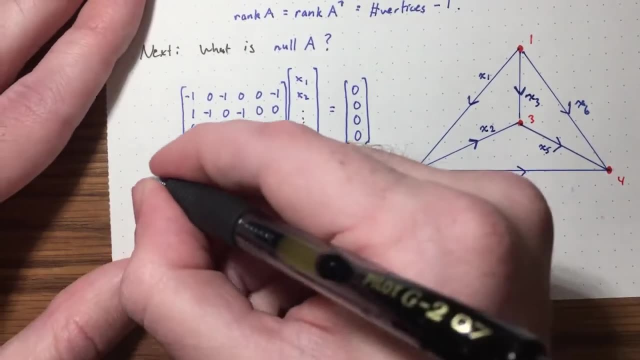 X21., X22., X23., X24., X25., X26., X27., X28., X29., X30., X31., X32., X33., X34., X35., X36., X37. X38., X39., X40., X41., X42., X43., X45., X46., X47., X48., X49., X50., X51., X52., X53., X54., X55.. 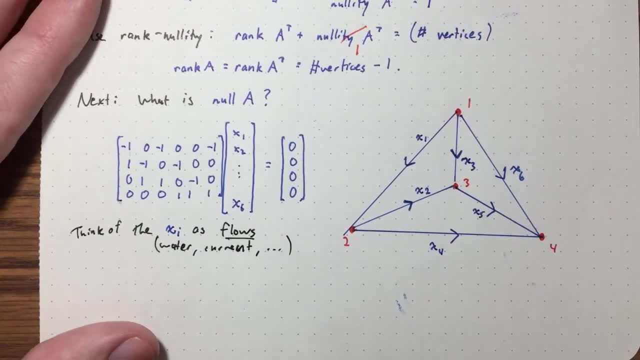 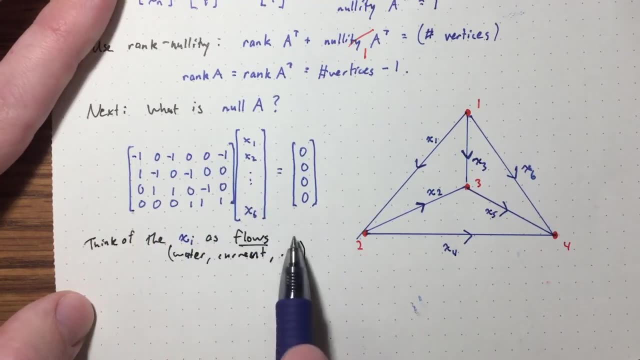 X56., X57., X58., X59., X59., X60., X61., X62., X63., X64., X65., X67., X68., X69., X70., X71., X72., X71., X72., X73., X74., X74., X75., X74., X72., X75., X76., X78., X89., X10., X11., X12., X12., X13. 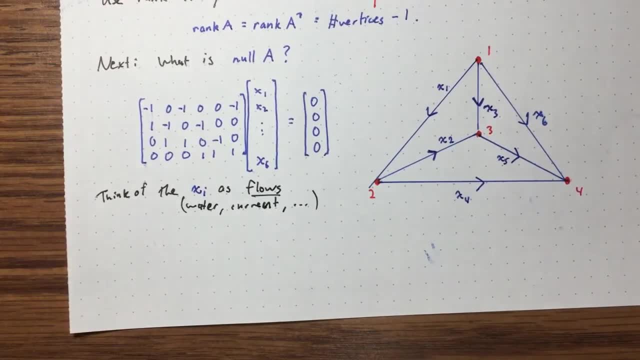 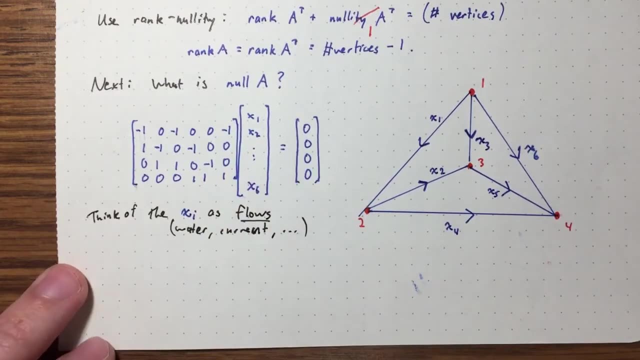 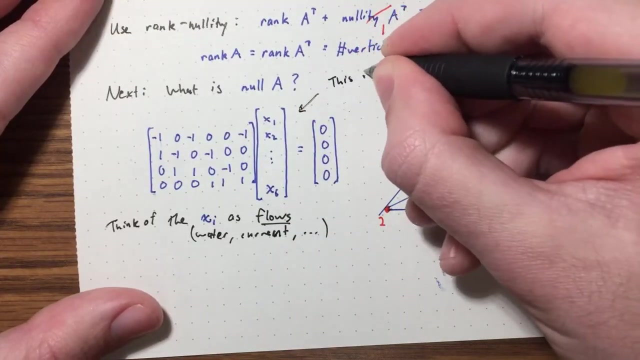 X14., X15., X16., X17., X19., X21., X23., X24., X25., X26., X28., X39., X19., X20.. so this is really cool. so this is saying. what it's really telling me is um outflow equals. 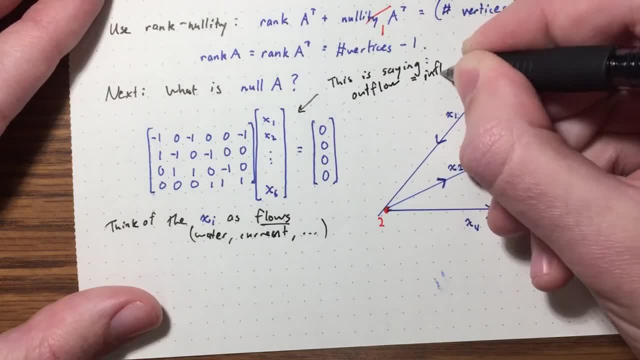 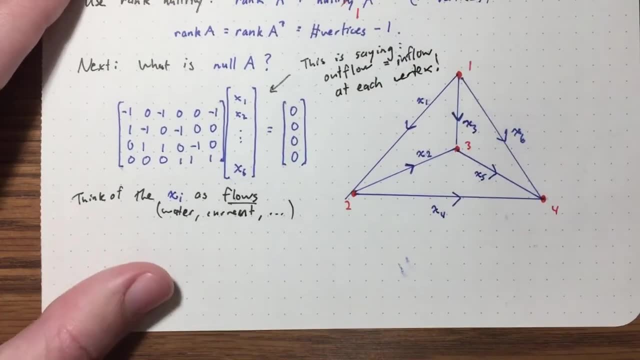 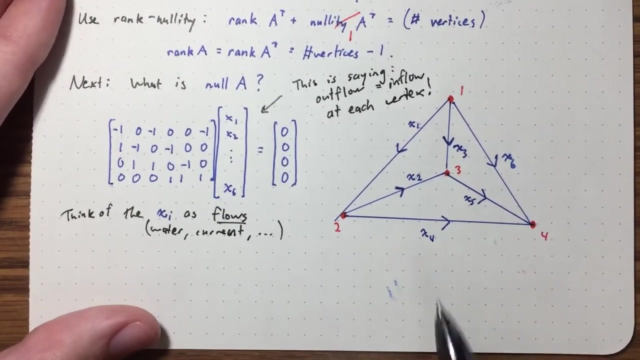 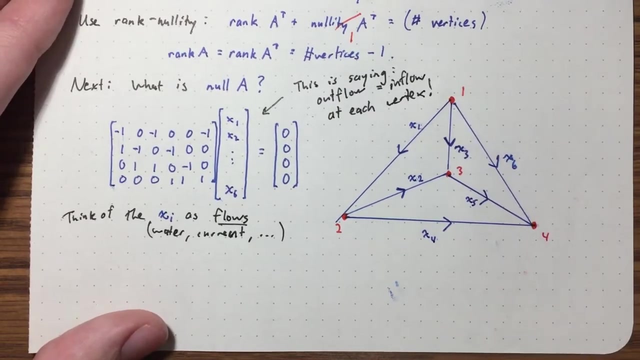 inflow at each vertex okay. so that's why i can think of these xi's as some kind of flow okay. so if i, if i have five units of flow going this way, i need to make sure that there are five units of flow kind of going back along these two okay, because i need the outflow to equal the inflow. 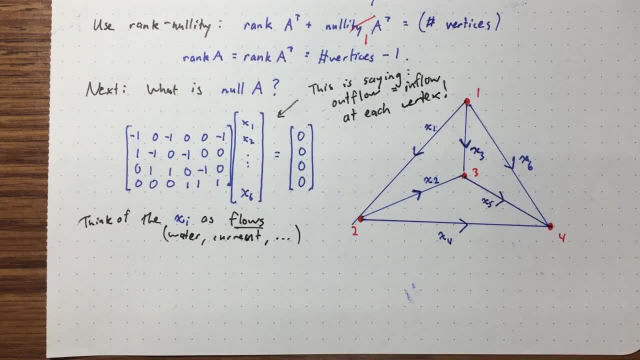 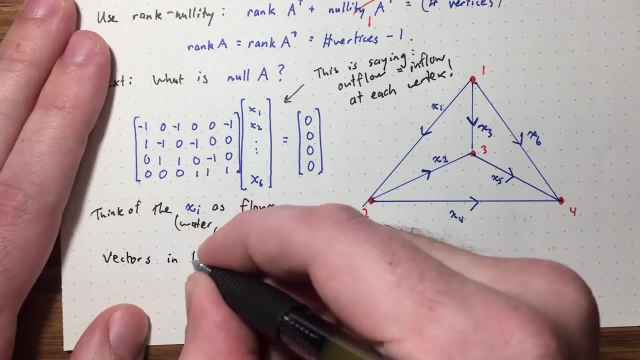 each vertex. that's what this equation is really saying, so we're taking some time to think about that, if you're a little unsure about that. um, okay, so what is the vector xi in a null space? so vectors. again, they're flows. so vectors in the null space. 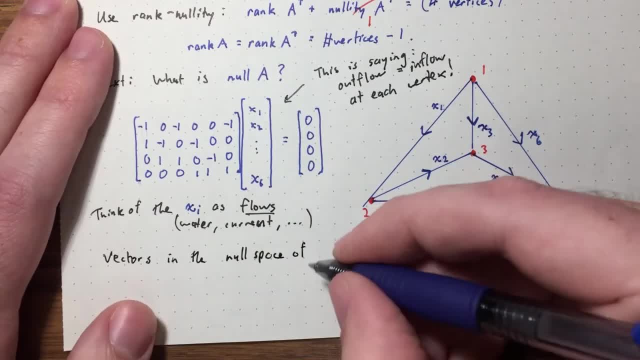 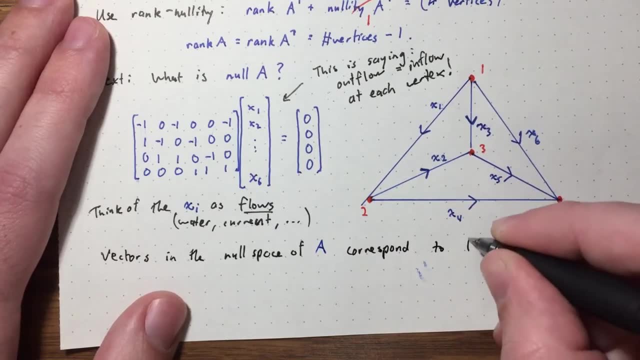 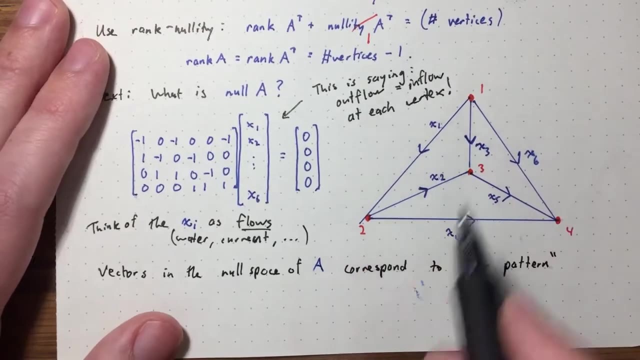 of this matrix, a correspond correspond to, you know, various flow patterns in the graph, but it needs to be a valid flow pattern, so i need the inflow to equal the outflow at every vertex. that's what setting this equal to zero is saying. the flow patterns in the graph. 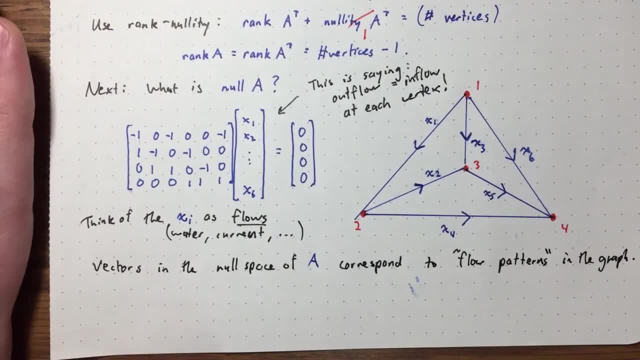 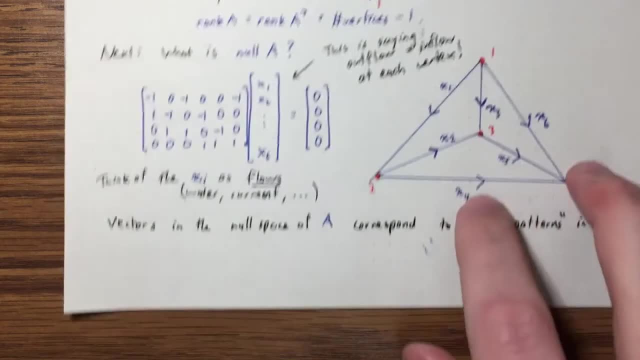 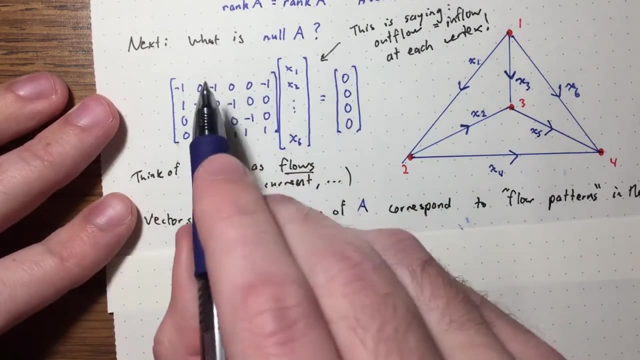 okay, can we try to find a vector that's in the null space space? Let's see if we can find a vector in a null space. Let's just stare at the columns here. So what if I take the first column and the second column? Well, I get minus 1, 0, 1.. I'll just take. 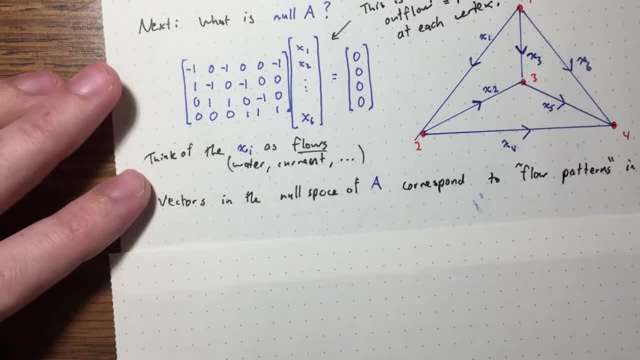 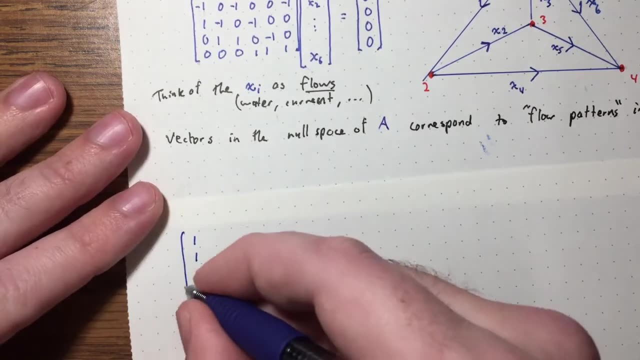 one copy of each. But see, that's exactly my third column. So I claim that this vector is in a null space. I'm going to take one copy of my first column, one copy of my second column and I'm going to subtract off the third column And I'm just going to ignore the fourth through sixth. 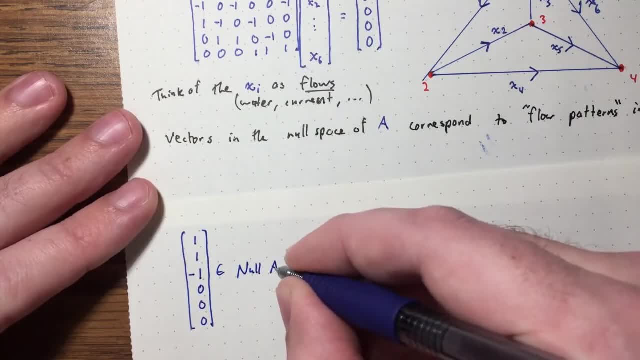 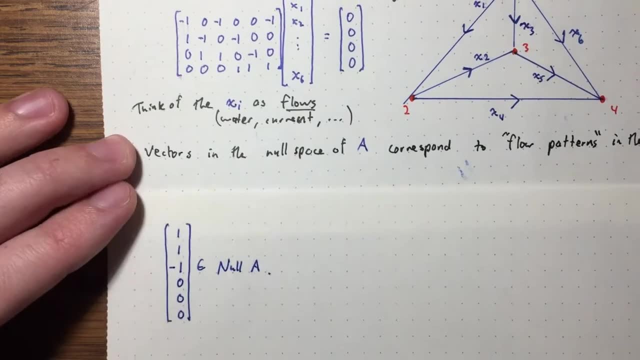 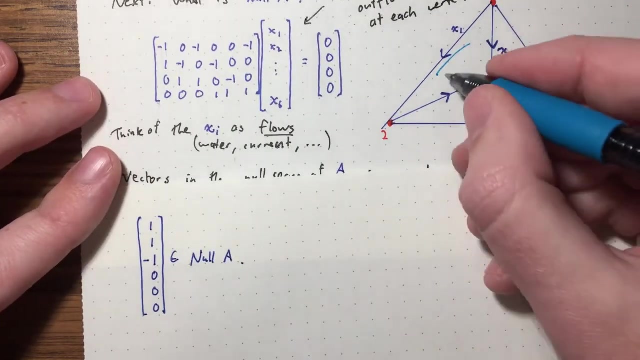 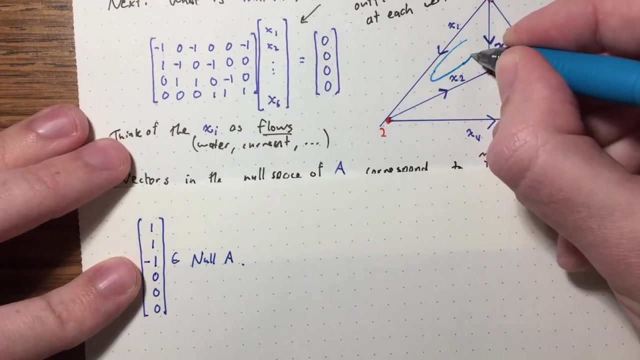 columns. So this is in my null space. What does that represent on my graph? It means I have one unit of flow going this way And I have one unit of flow going along x2.. And then I have minus one units of flow going along x3.. So that's actually going this way. 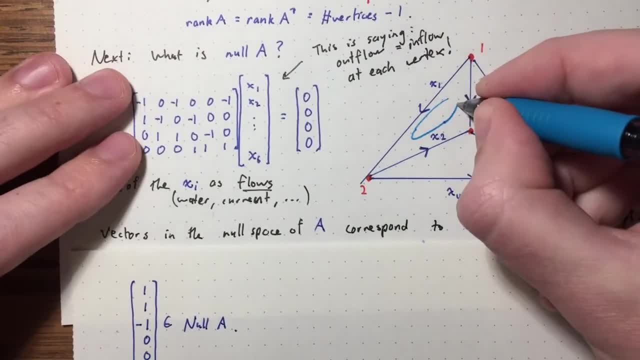 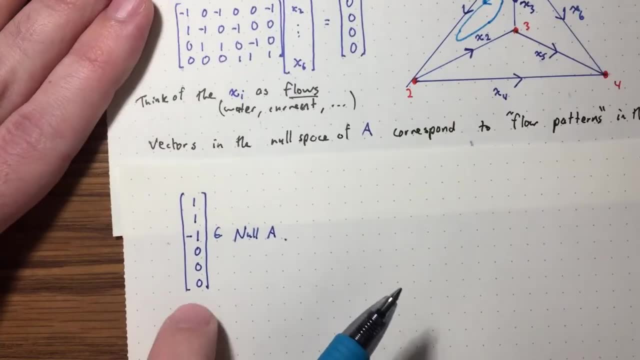 right, It's going in the opposite direction of x3. And that's a closed loop. Okay, so I have some flow going around this loop. That's what that vector represents. This is really cool. Can we see some other vectors in our null space? 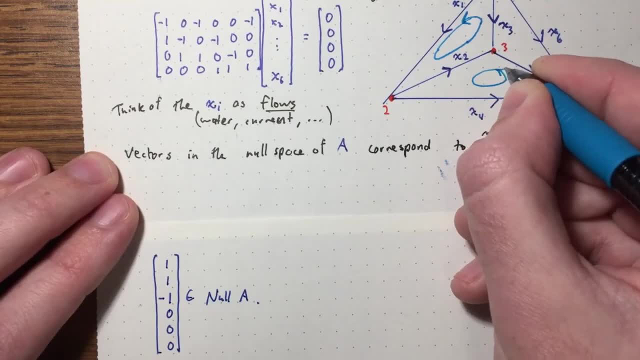 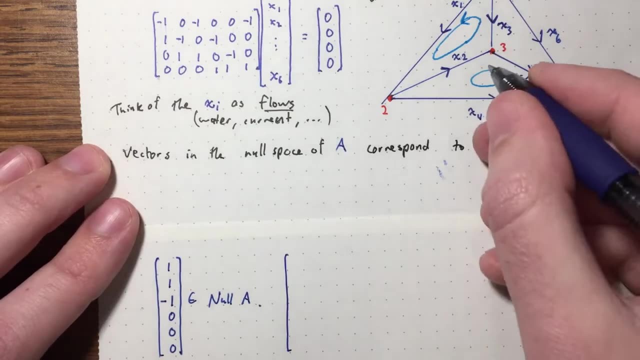 What about this one? If I take this loop here? It's so cool. You're going to see visually some vectors in a null space. I'm going to write down what that one is. I'm going backwards along x2.. So I have a minus 1.. 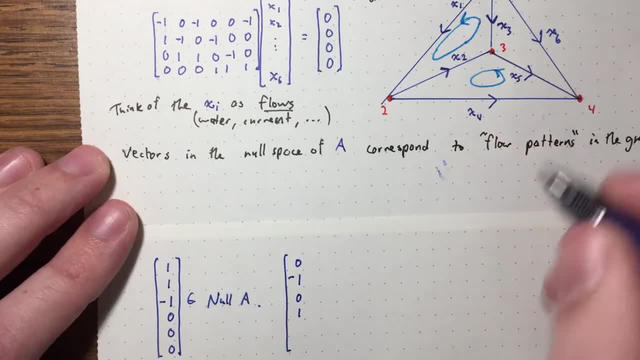 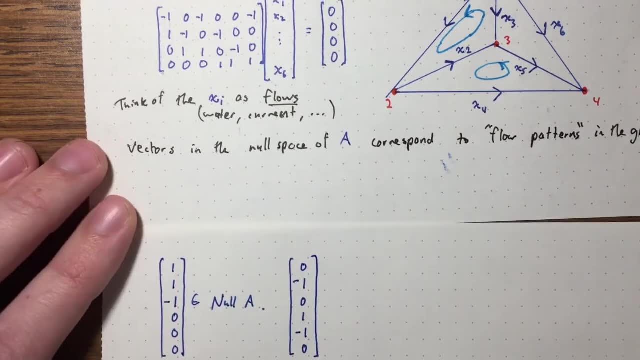 And I'm going along x4 in the forward direction And I'm flowing backwards along x5. So I'm going to put a minus 1 again. I think this vector is in a null space And you can check by multiplying it by this matrix, if you want. 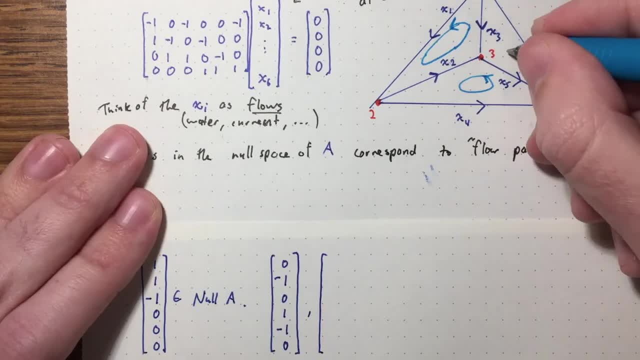 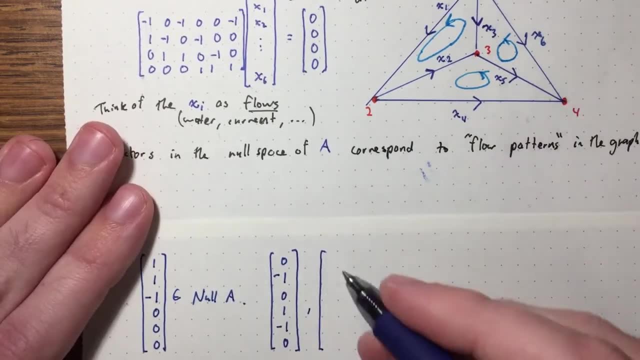 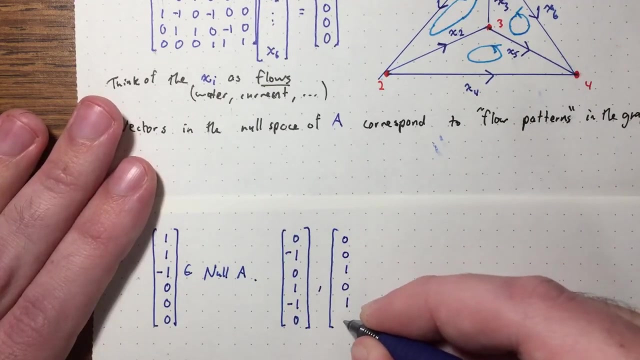 And then how about this loop here: Say we go that way, It doesn't matter which way you go, You'll get a different result. So we have x3. This should be 1, and then 1, and then minus 1.. You see how I got that. 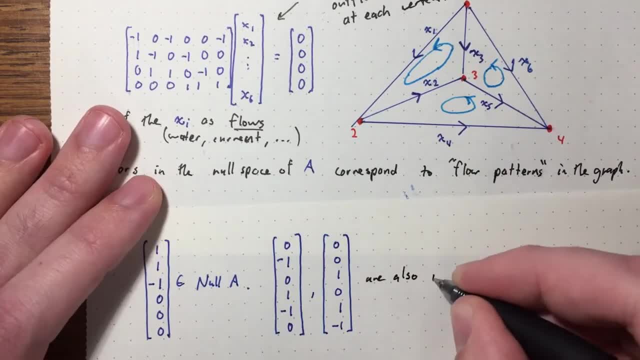 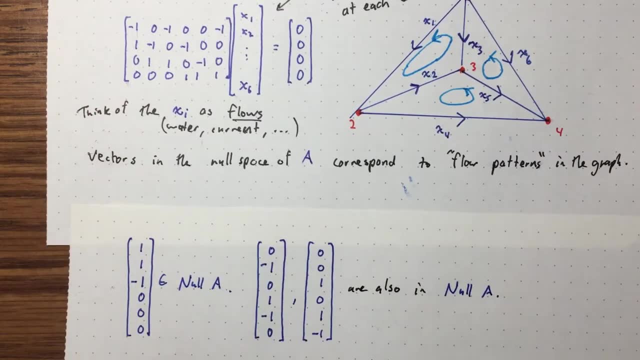 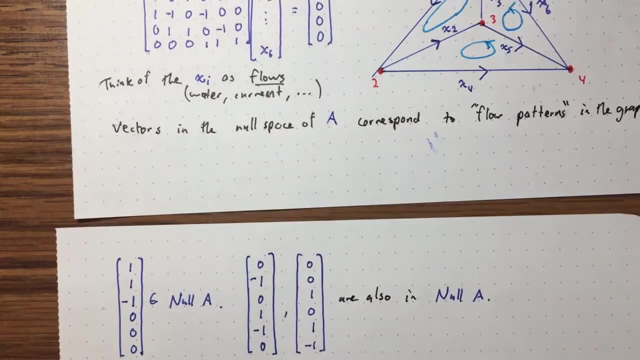 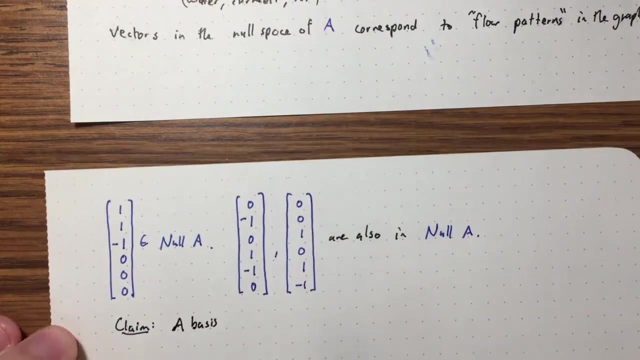 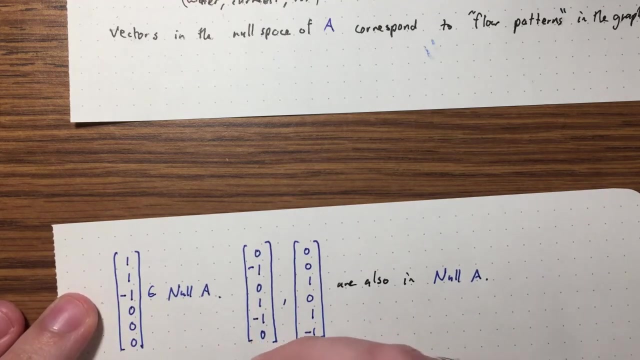 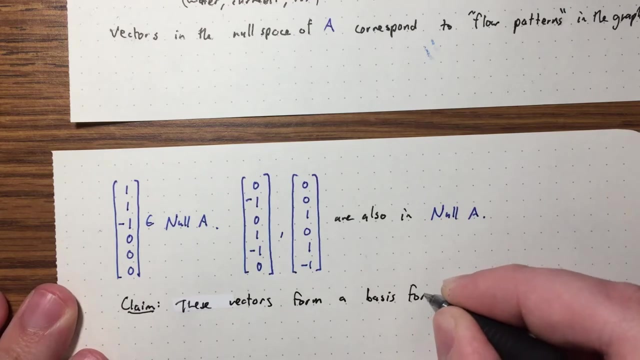 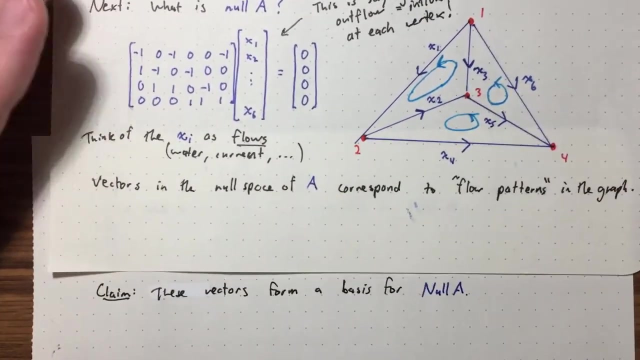 So these are also in the null space And the claim I'd like to make: is that a basis? Actually, yeah, So these three vectors I just wrote down, these vectors form a basis for the null space. In other words, if I have any kind of flow pattern on this graph, 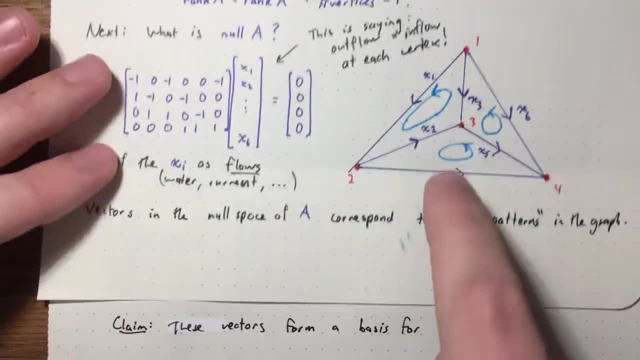 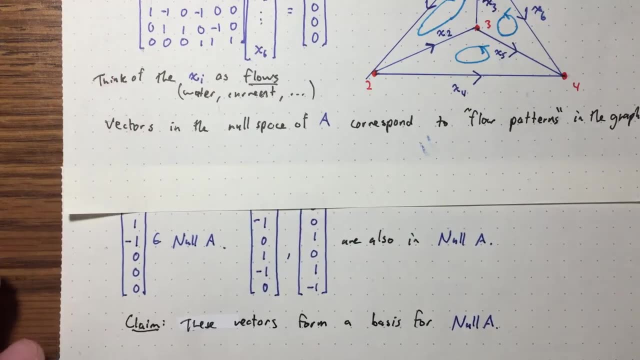 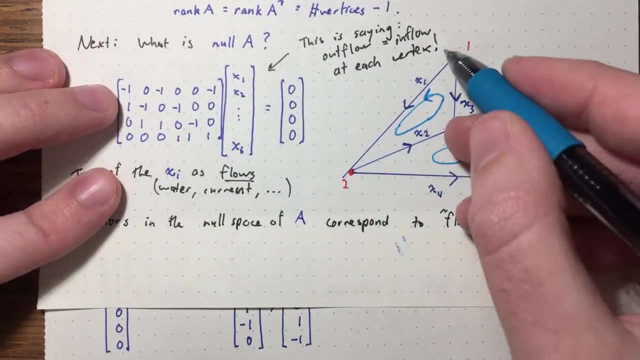 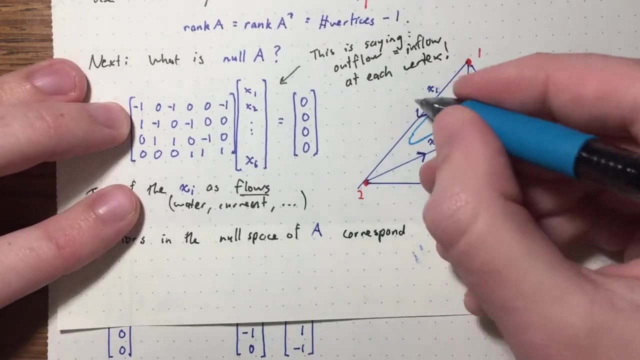 I can get it by just taking linear combinations of these loops, These small loops here. Can we just check that? So what if we had a different loop? Why don't we need this larger loop? So let me write that down. What if we had this loop here? 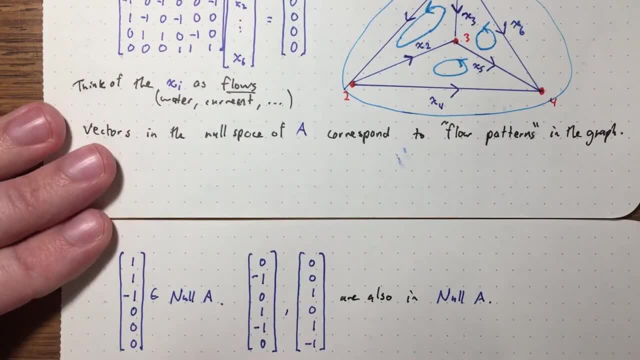 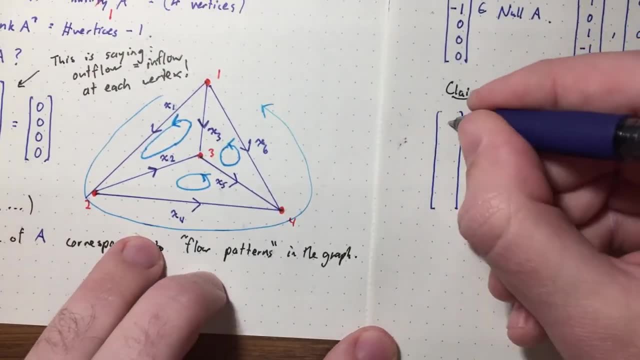 That would be this. That would correspond to the following vector: in the null space. And this is in a null space. Okay, So we do x1. Then we're going along x4. And then we're going in the backwards direction, along x6. 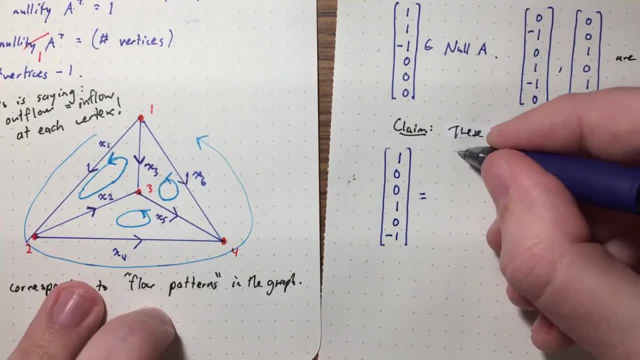 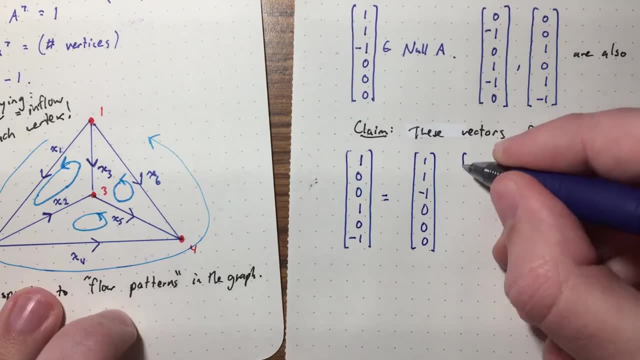 But I think I can write that vector as a linear combination of these three. Let's see if we can do it. So your job is to simply write that vector as a linear combination of these three. So that's just one way to do it. 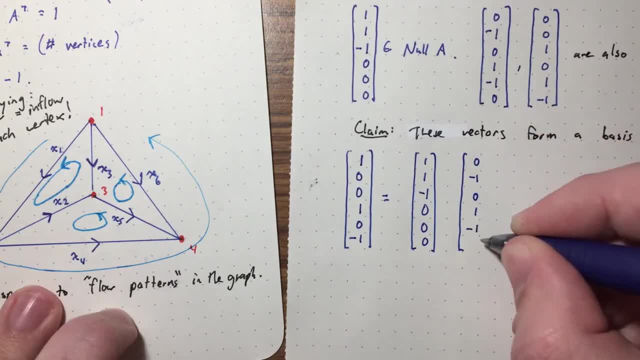 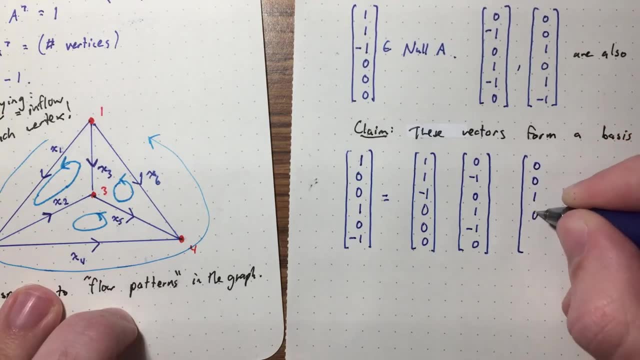 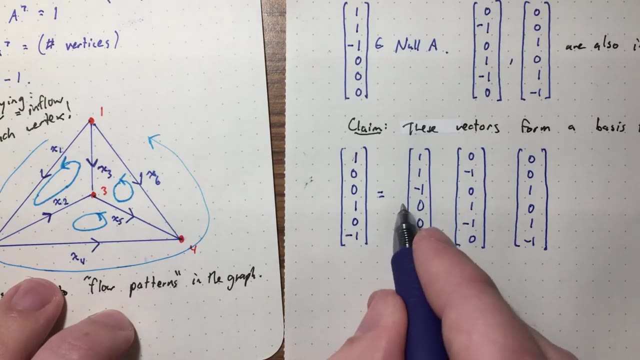 Let's see how we can do this. So your job is to figure out the coefficients. Okay, Well, for that to be a 1, I have to use that 1.. So I need 1 of this vector, And then 1 minus 1 is 0.. 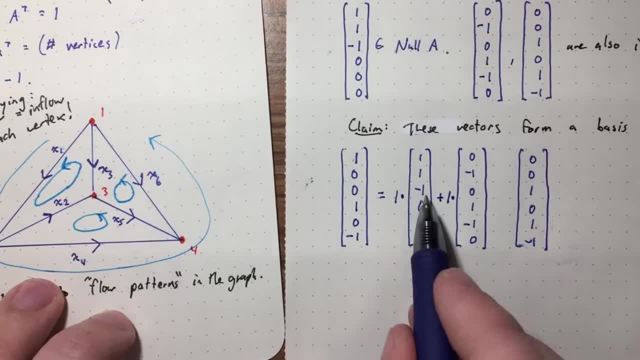 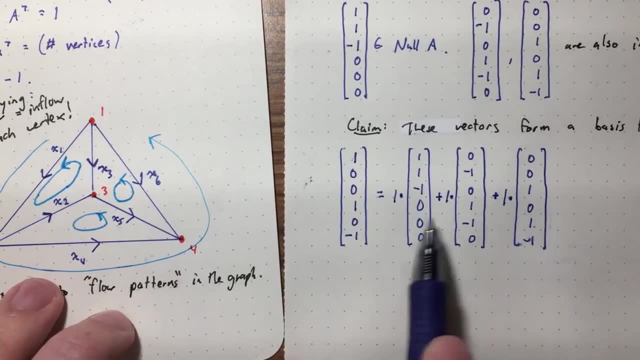 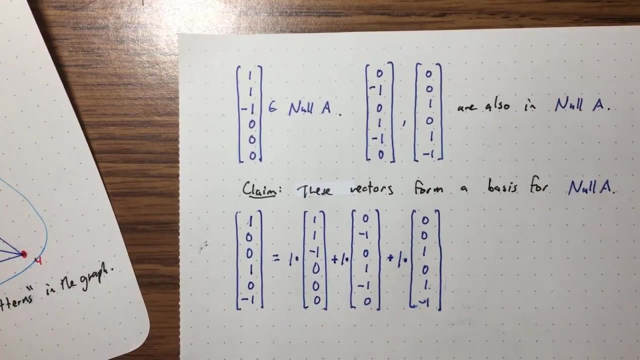 I think I want 1 of this vector also, And then I have a minus 1.. I think I also want 1 of this vector. Does that work for the rest of the entries? Yes, I think it does. Yeah, so actually this one we can just write as a linear combination of the loops, the small loops. 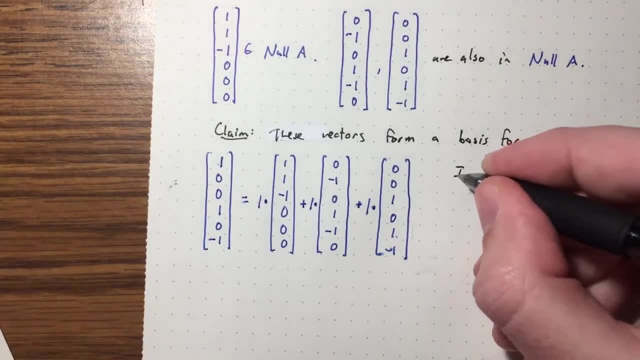 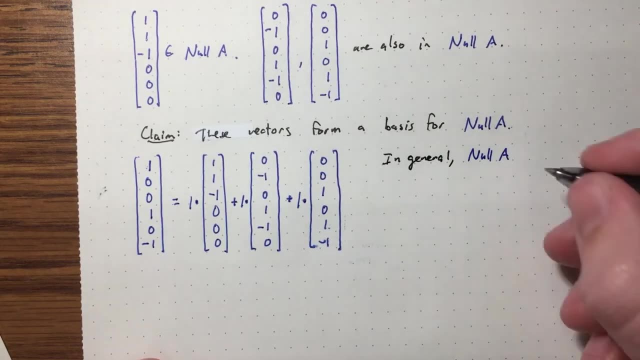 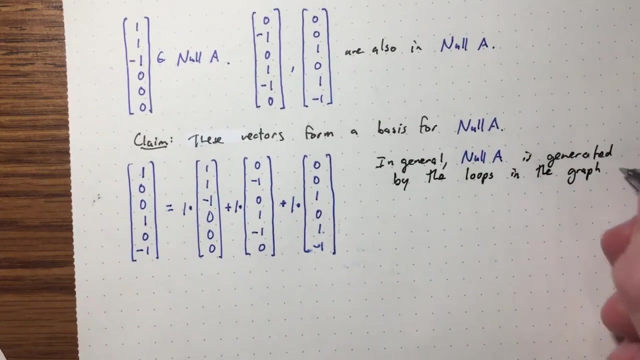 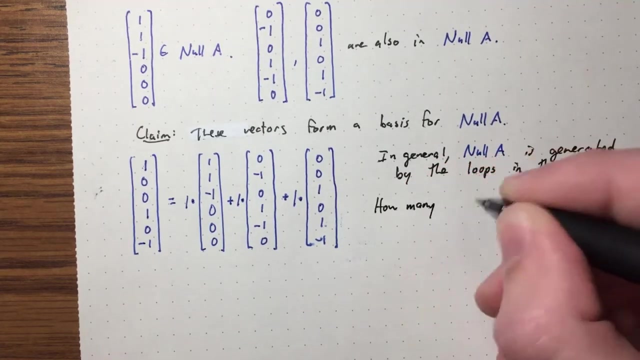 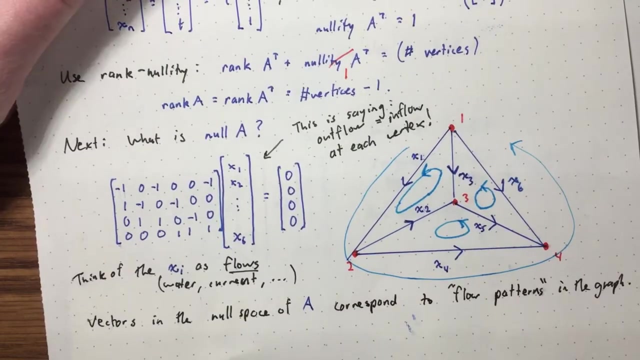 This loop here, that loop there, that loop there And, in general, the null space is generated by the loops in the graph. Okay, So how many loops are there? Ah, okay, So here there are 3 loops: 1,, 2, 3.. 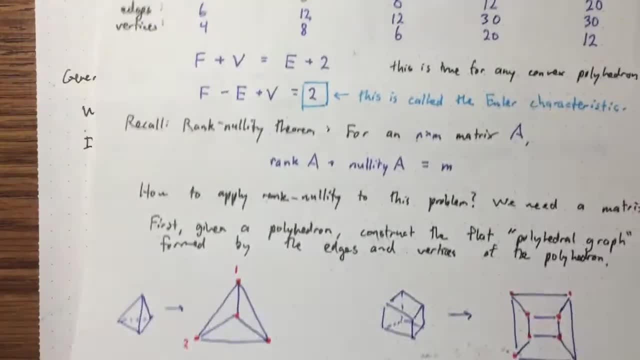 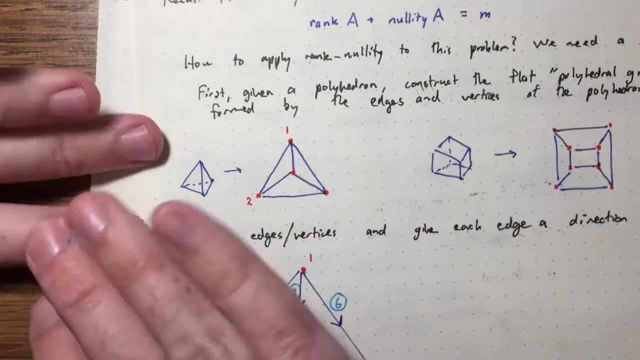 Where do those come from? They come from the tetrahedron. Remember, to get this graph, I sort of removed one of the faces and then flattened it down, So I see my 3 faces. There is one face. This is that face. there, let's say: 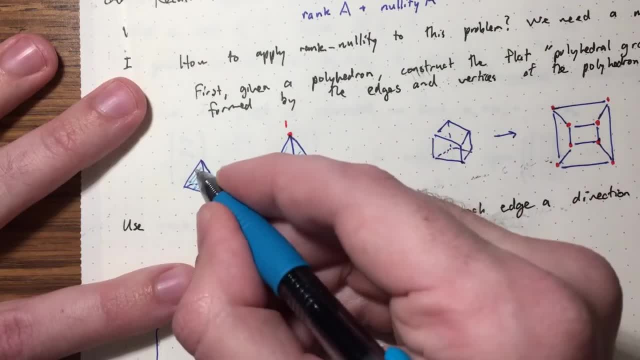 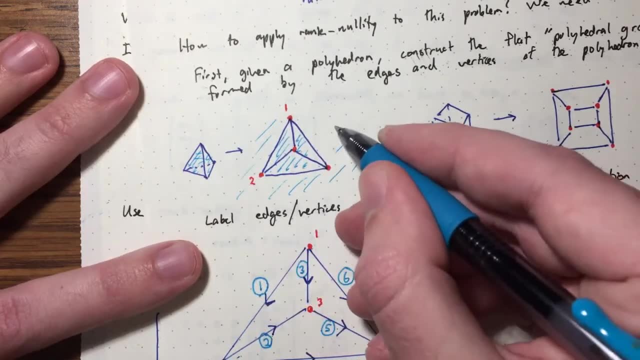 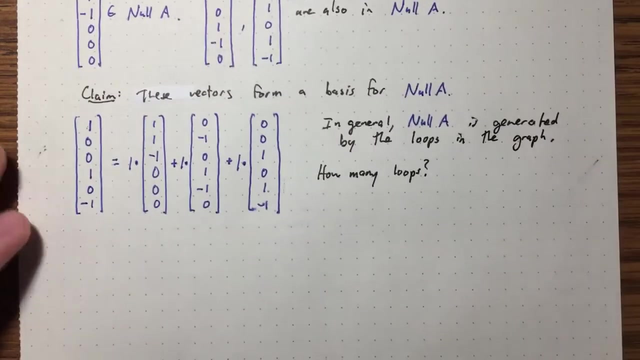 And this one here is that face here And this face here is the one in the back, But I have a fourth face. The fourth face was the outside Of my picture. It's the one I removed, if you like. So I claim that a number of loops in my graph. 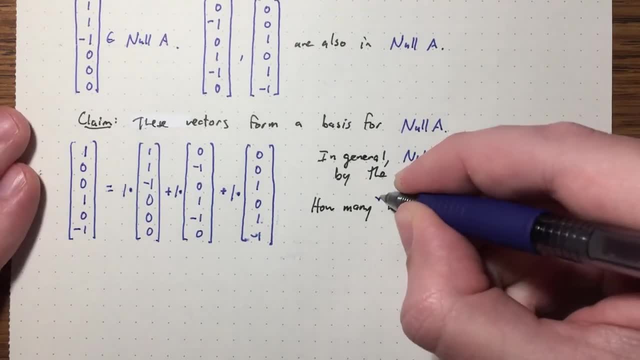 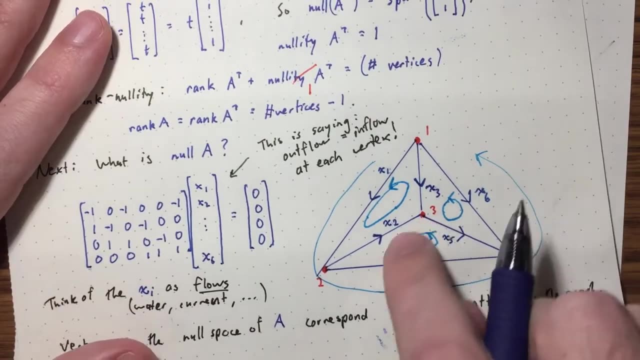 is the number of faces in my polyhedron. Maybe I should say something like minimal loops, by the way, Because technically this whole thing is a loop also, But I just want the smallest loops Because again, I can generate any other loop by just these three. 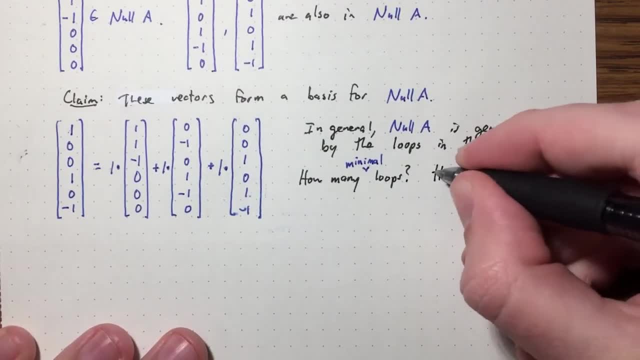 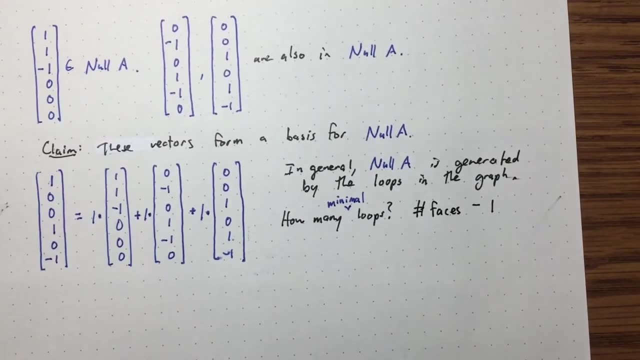 Okay. So how many minimal loops do I have? Well, it's the number of faces in my polyhedron, But I have to take away one Right, Because I took away 1 just to be able to squash it down and do it. 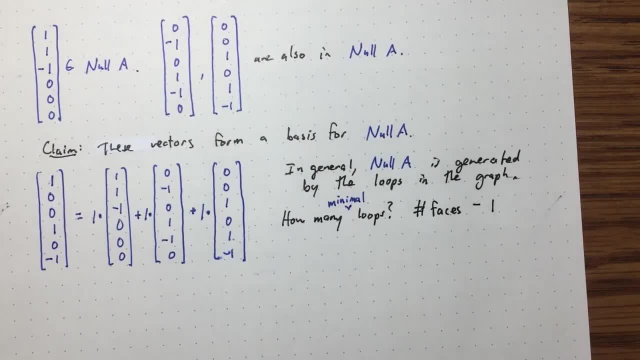 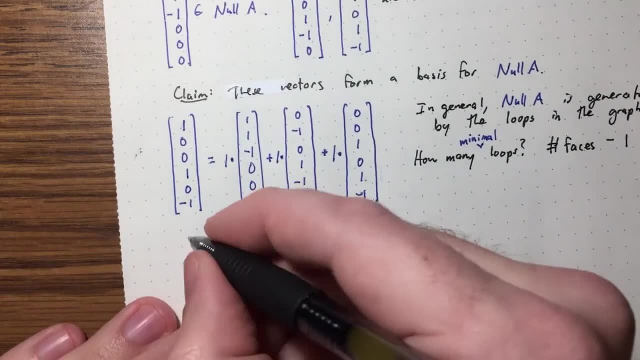 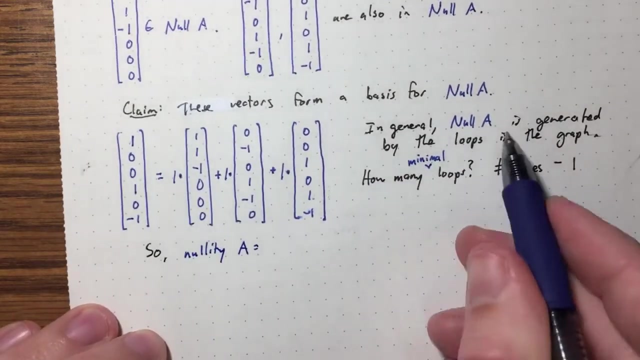 Okay, So I'm going to take 1 and do a polyhedral graph. Okay, What did we just see here? We saw that So the nullity of A is the dimension of the null space. But what is the dimension of the null space? 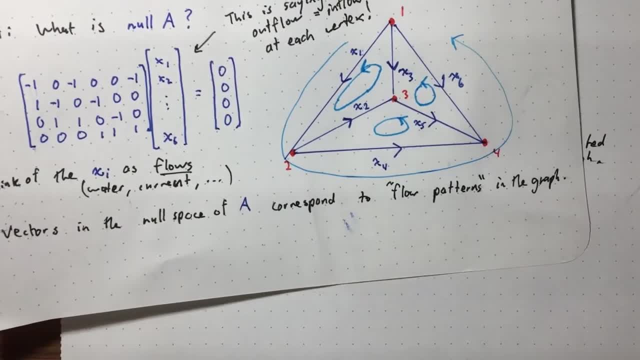 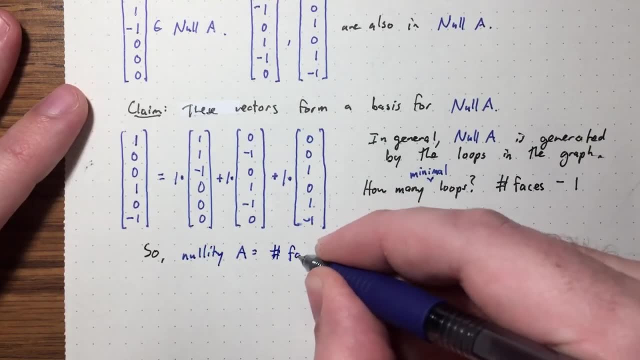 The null space we decided was generated by these loops. Okay, The vectors corresponding to these loops, Which is the number of faces minus 1.. The number of faces minus 1.. I should do the same thing. That's the dimension of the null space. 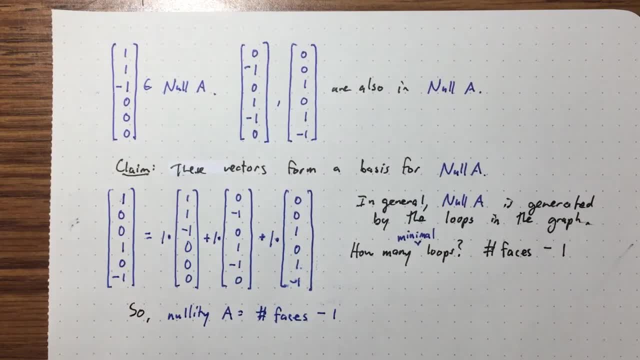 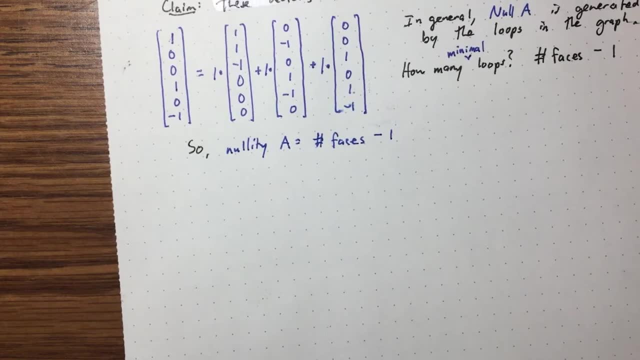 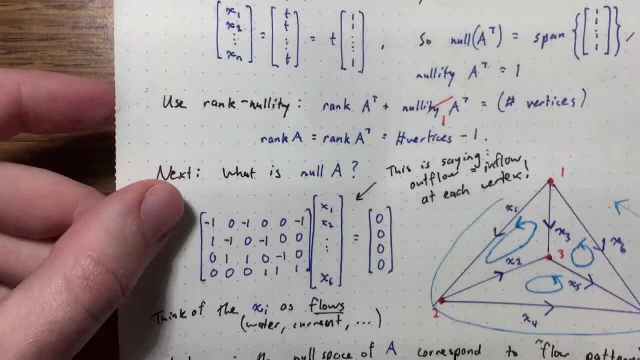 So we have three basis vectors. So we have three basis vectors. Okay, What next? We know the rank of A. Well, where was that? That's right here. So the rank of A is the number of vertices minus 1.. 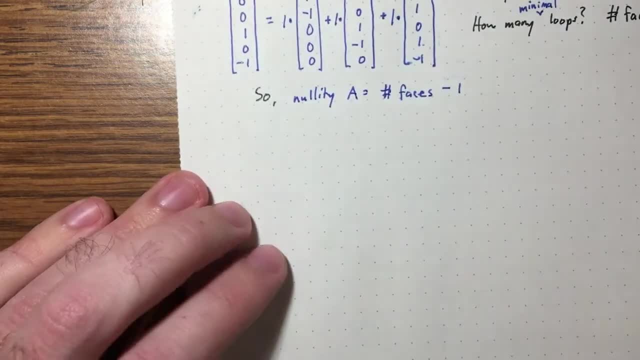 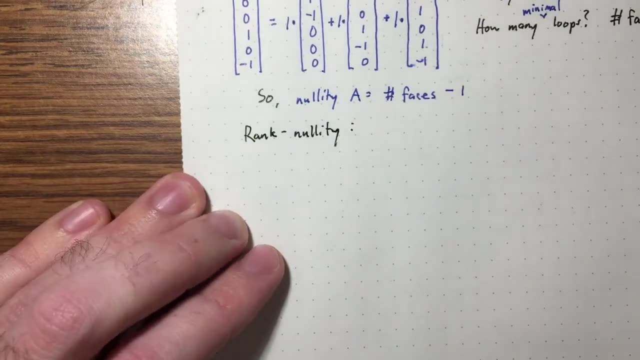 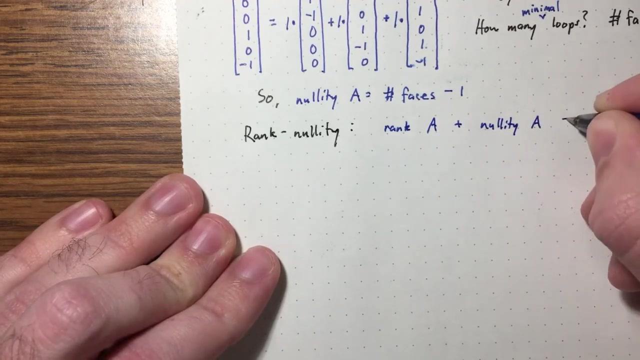 We know the nullity of A. We know the nullity of A, We know the number of vertices minus 1.. what does rank nullity tell us? It tells us that the rank of A plus the nullity of A equals. what is it going to equal? 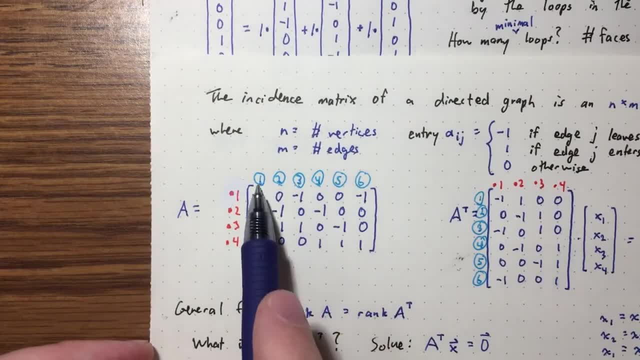 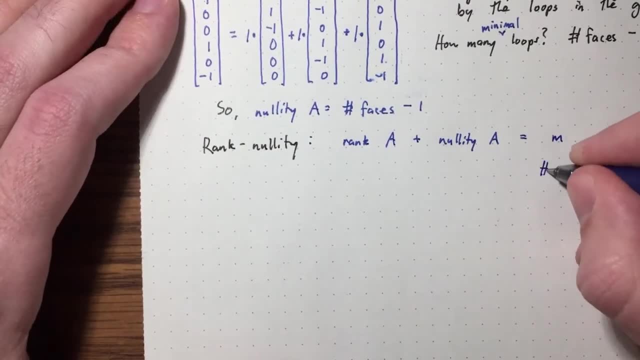 It's going to equal the number of columns of A, which is the number of edges, That's M, Which is the number of edges. So I'll just immediately write: that's the number of edges. The rank we found was the number of vertices. 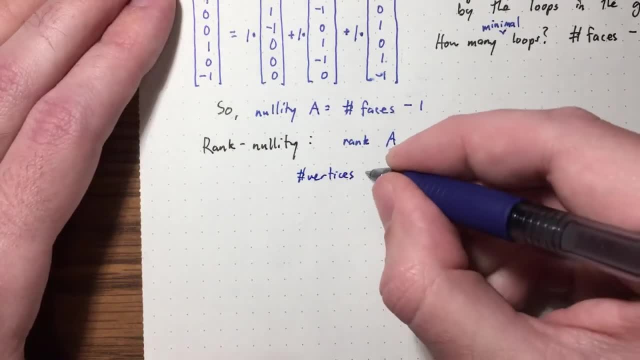 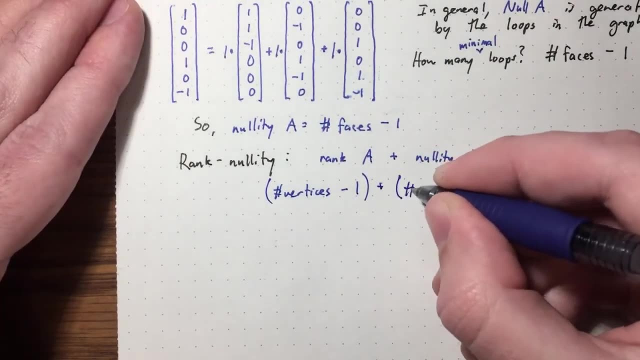 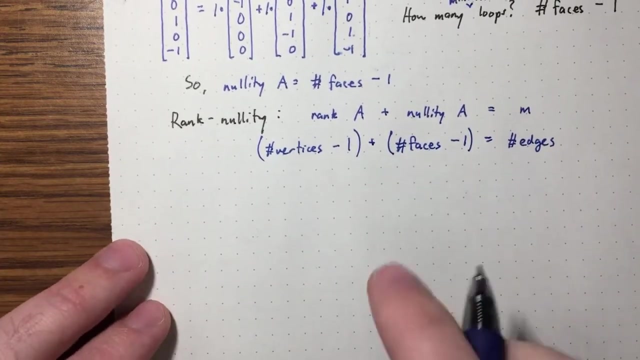 minus 1.. That's the rank of A. The nullity is the number of faces minus 1.. Rank nullity tells us that that equals the number of edges. So let's rearrange this. We have a minus 2.. We'll move that to the other side. 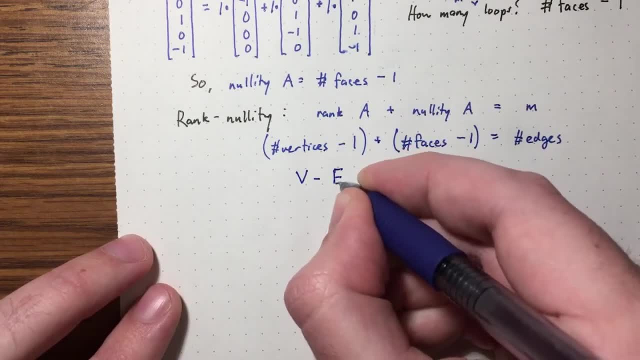 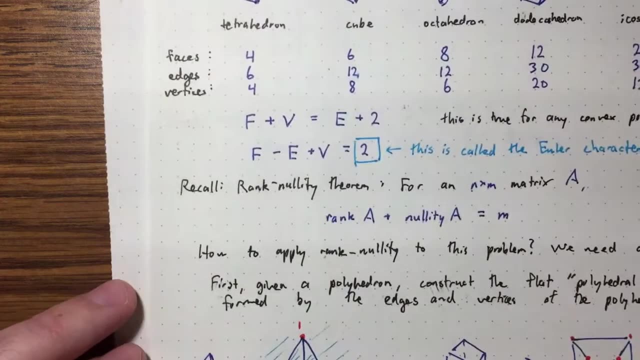 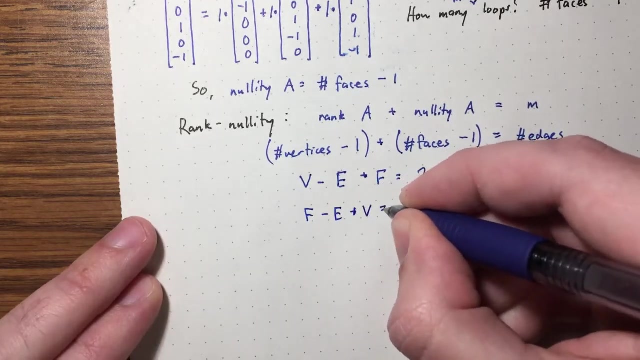 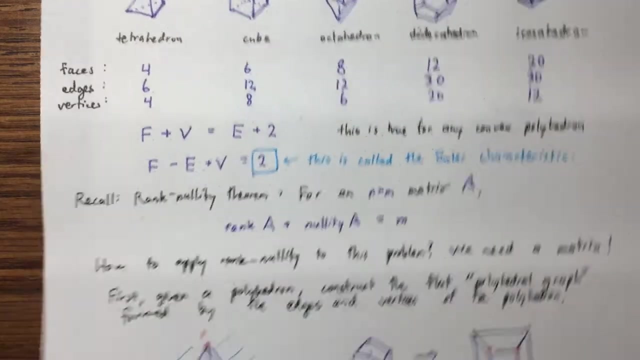 And we get our formula: V minus E plus F equals 2.. So we wrote: F minus E plus V equals 2.. It doesn't matter, Wow. So that's pretty unexpected, right? You can get some statement about the geometry of polyhedrons. 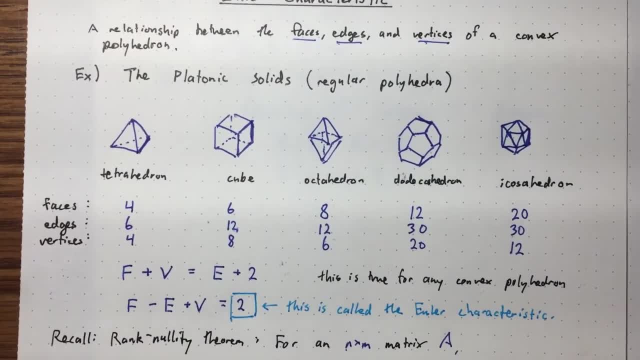 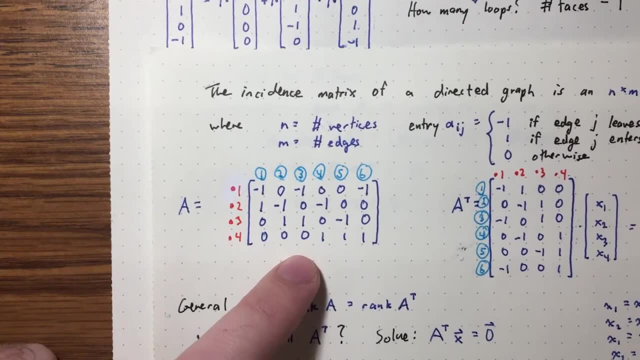 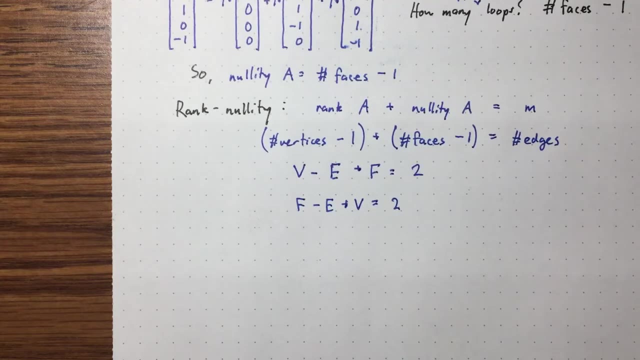 from the rank nullity theorem, And it's not just the rank nullity theorem, It's the rank nullity theorem applied to a matrix, And that matrix that we applied it to was the incidence matrix associated to the polyhedral graph. Okay, 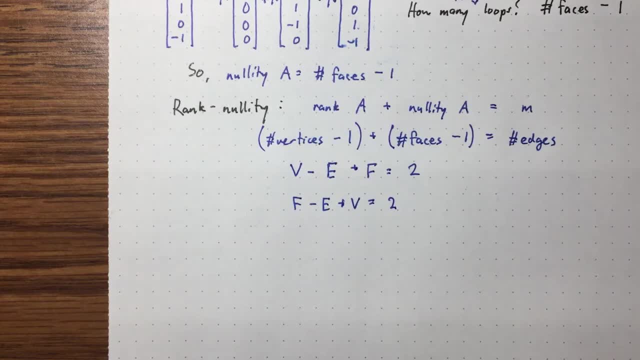 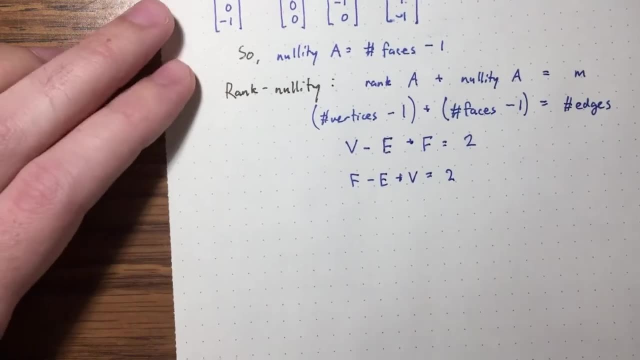 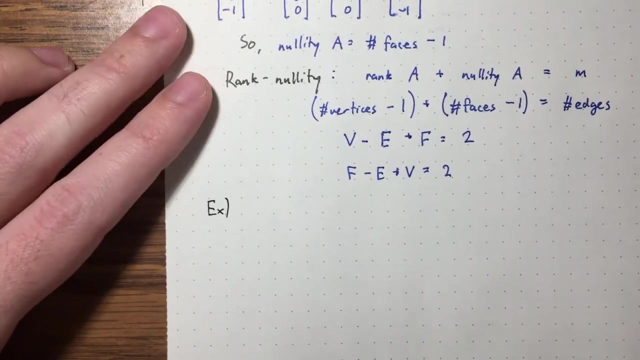 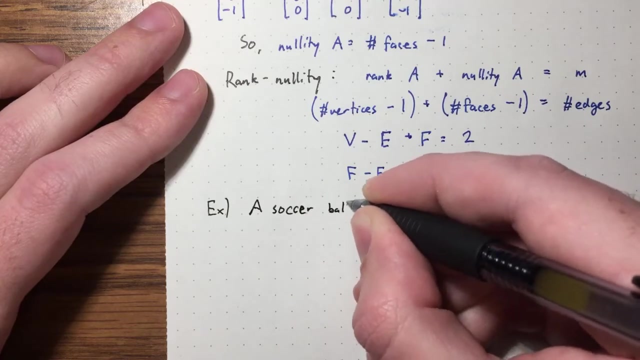 This has a lot of cool applications, So let me just show you one. Let's do the following problem. So here's an example Just of how you might use this. Okay, I mentioned a soccer ball earlier, So a soccer ball is made. 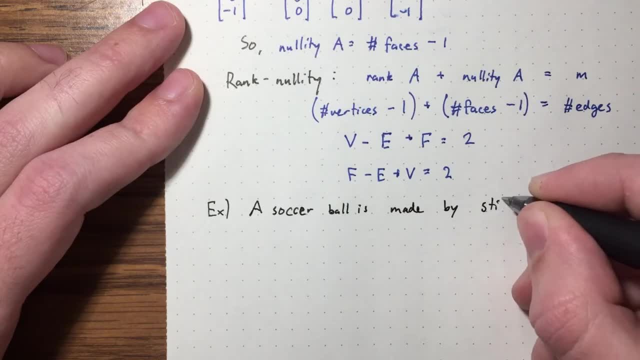 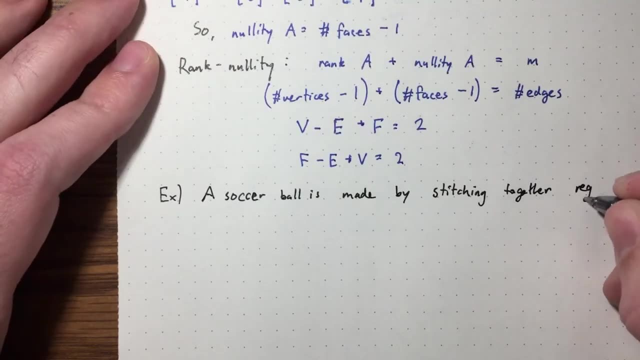 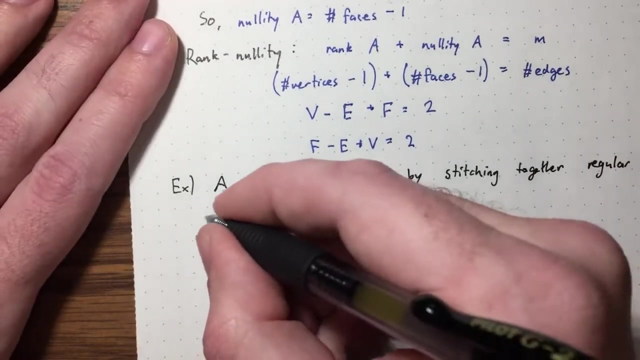 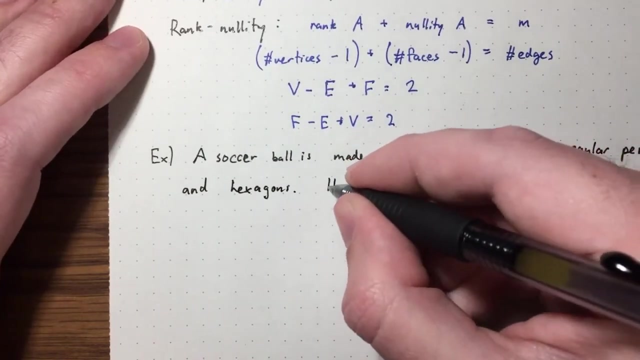 by stitching together two kinds of shapes. You've probably seen this. So you use regular pentagons and hexagons, Some number of pentagons and hexagons. I'm going to ask you a question: How many pentagons are needed? 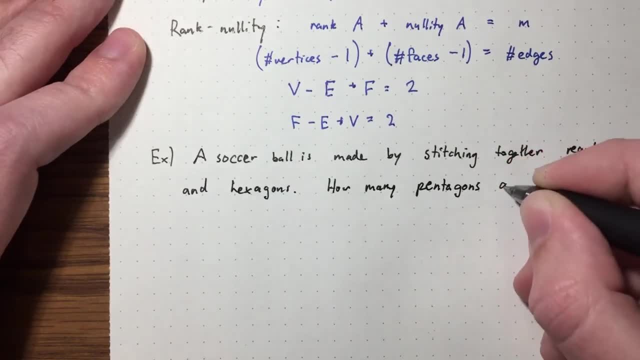 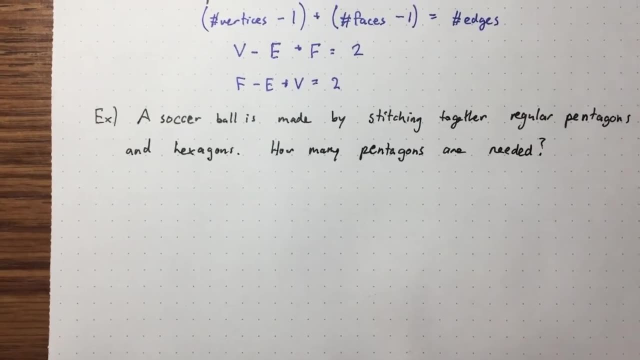 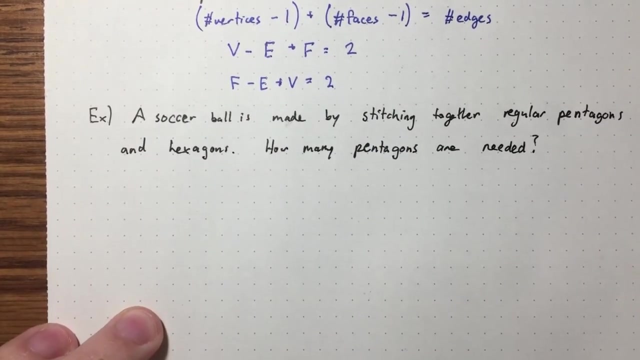 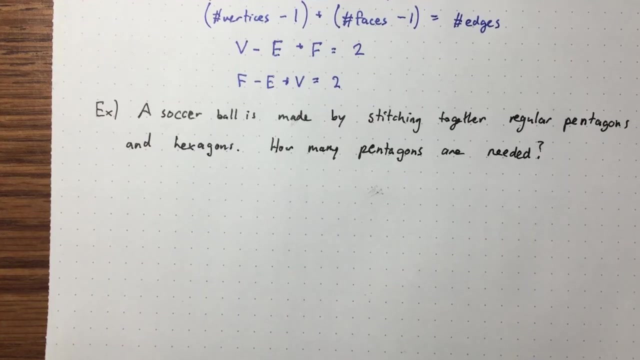 Without even looking at a soccer ball or looking this up, I claim that we can use this formula here, the Euler characteristic, to say exactly how many pentagons there are. Let's see how many pentagons we need. Let's see if we can do it. 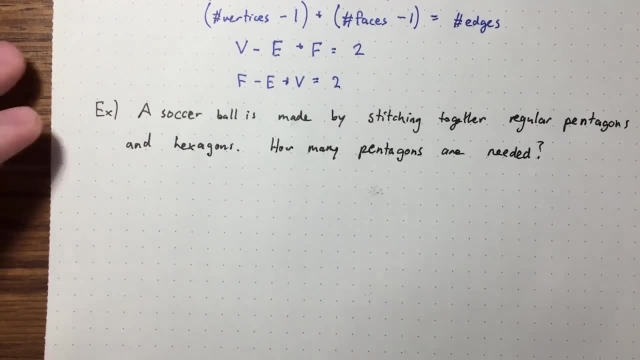 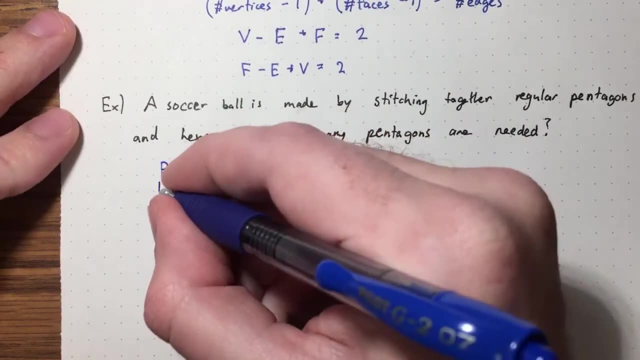 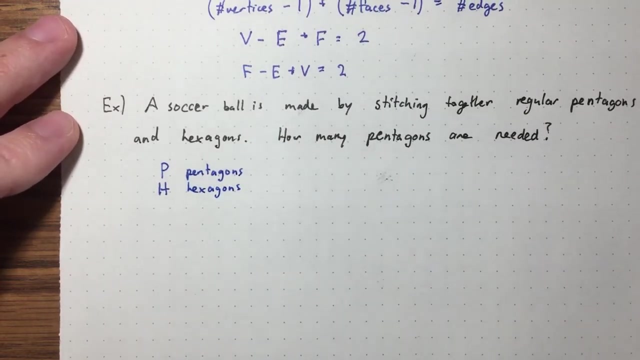 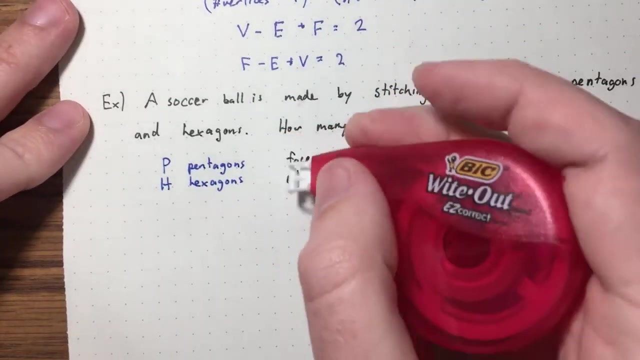 So let's say, our soccer ball uses P- pentagons- We'll give them variables- And H- hexagons. Okay, Let's see if we can write down the number of faces and the number of edges. That'll leave some room. 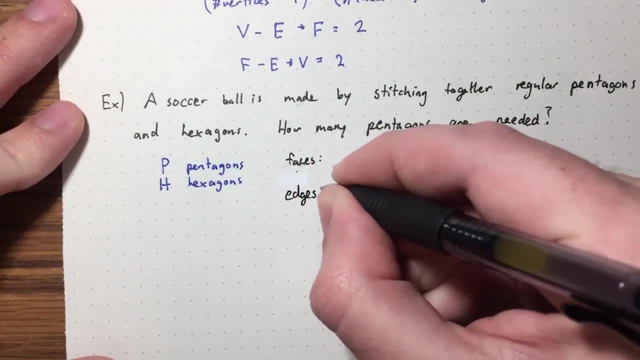 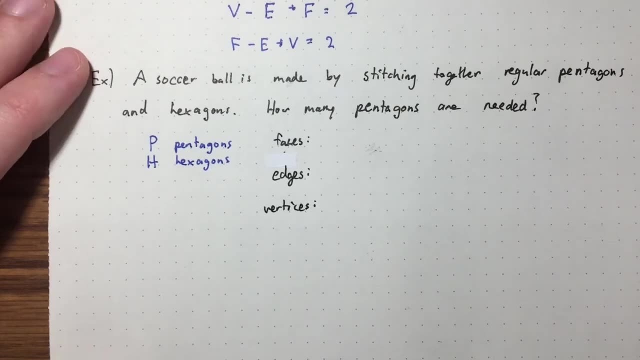 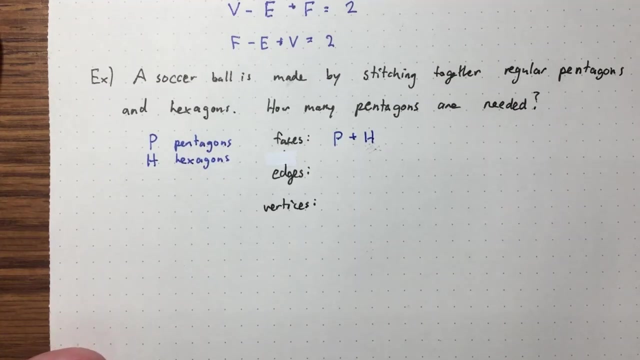 In case we have to do some calculations: Number of edges and a number of vertices. Well, first of all, if we have P pentagons and H hexagons, then certainly my soccer ball has P plus H faces. How many edges does it have? 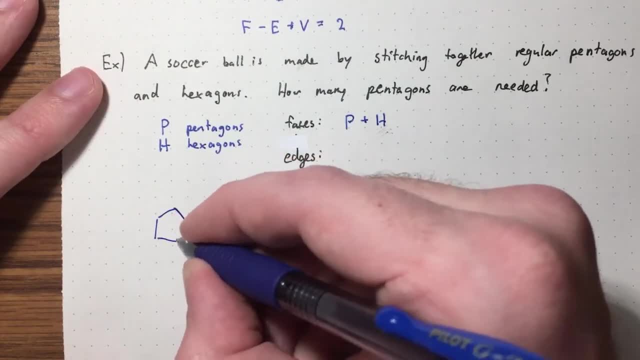 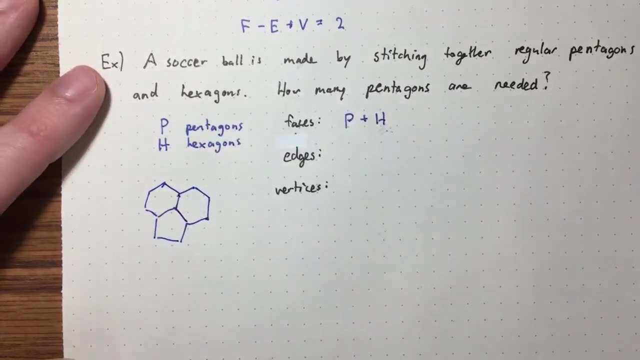 Well, I mean, what's the typical situation here? So I could have a pentagon and then maybe I have it connected to, Let's say it's connected to, two hexagons, But we don't even know that. So here's my pentagon. 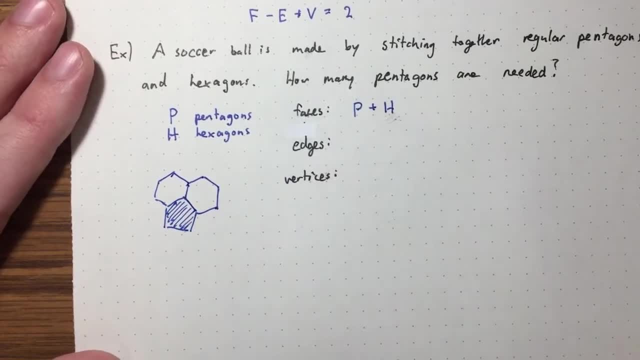 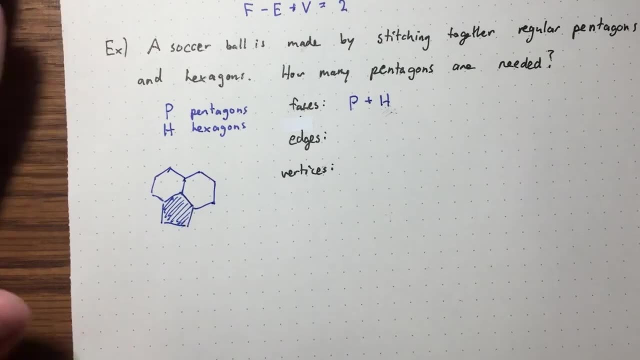 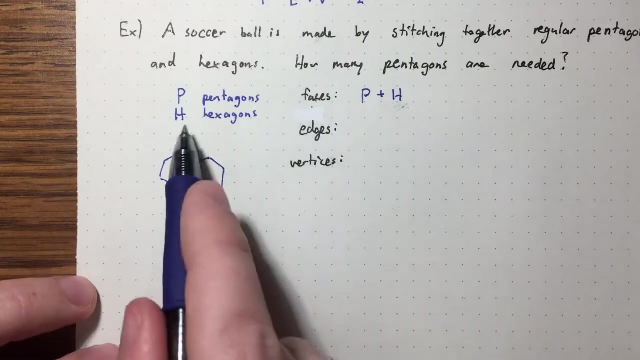 And I can continue this pattern. Put a hexagon there, pentagon. We're not really sure yet How many edges is this going to have? Well, here's how we can figure that out: Let's just count up all the edges of all of the shapes. 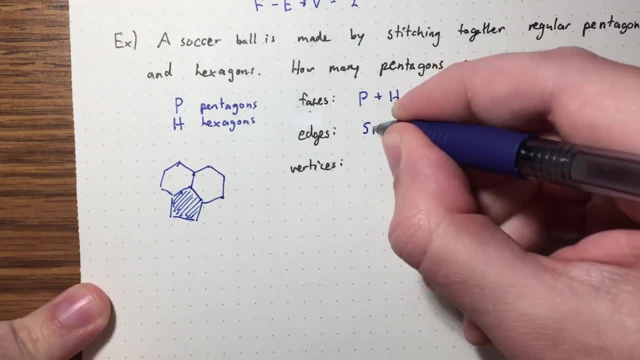 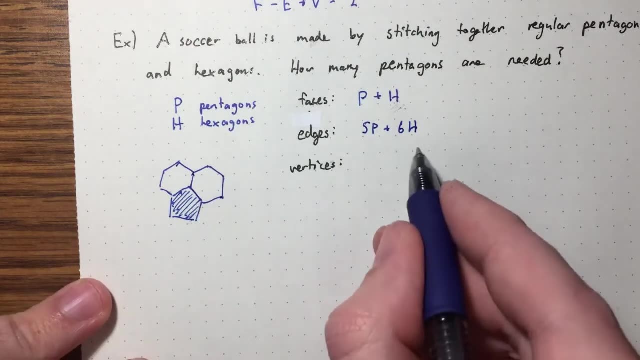 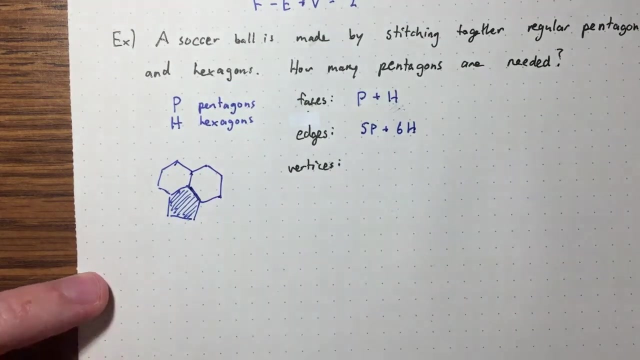 So what would that be? A pentagon has five edges And a hexagon has six edges. However, I actually overcounted, Because look at this edge. This edge is shared by the pentagon and the hexagon, So each edge is actually going to be shared. 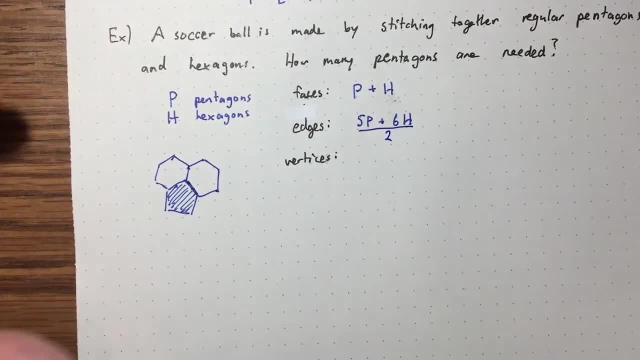 by two shapes, So I need to divide by two. I overcounted everything by a factor of two, So that should be my number of edges. This is a very typical problem-solving strategy, by the way, called overcounting. You overcount things, but you keep in mind what the factor. 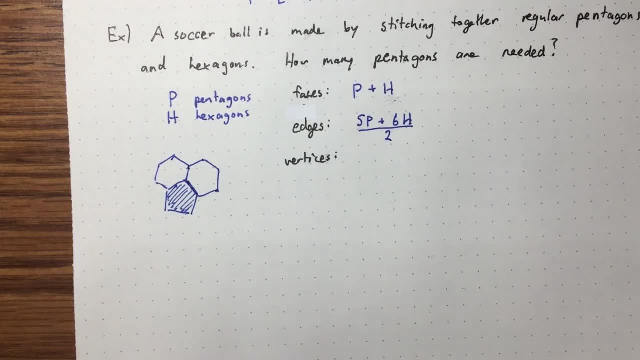 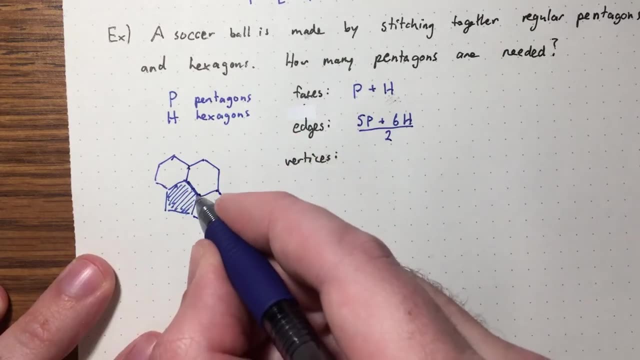 that you're overcounting by is. It's a good way of counting things. How about vertices? Well, each vertex- Maybe I have another shape here, So each vertex is shared by three shapes. How do I know that? by the way, 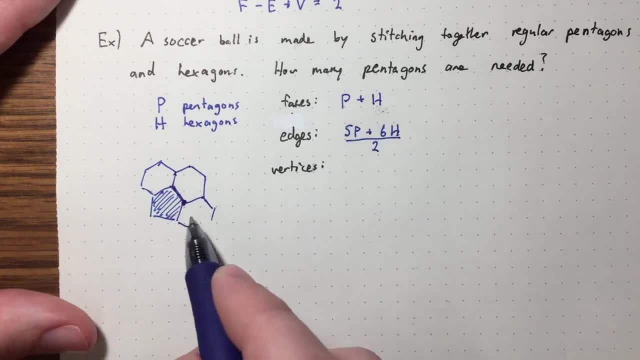 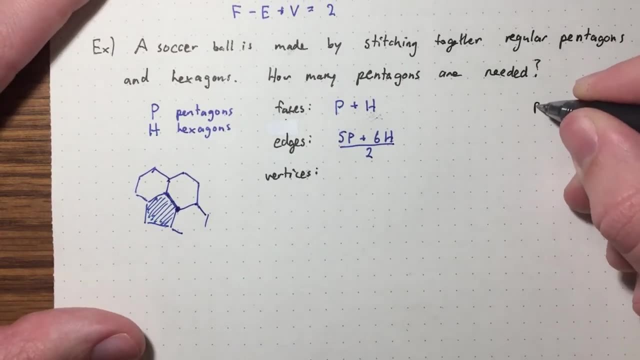 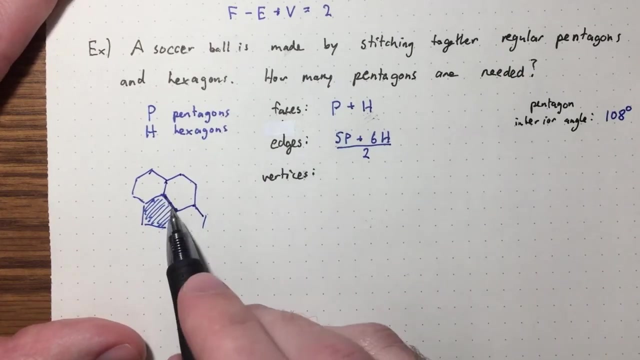 Can I have a vertex shared by four, Four shapes? Well, the answer is no, because the pentagon has an interior angle of 108.. So, even if we use four pentagons, if we add 108 plus 108 plus 108 plus 108,. 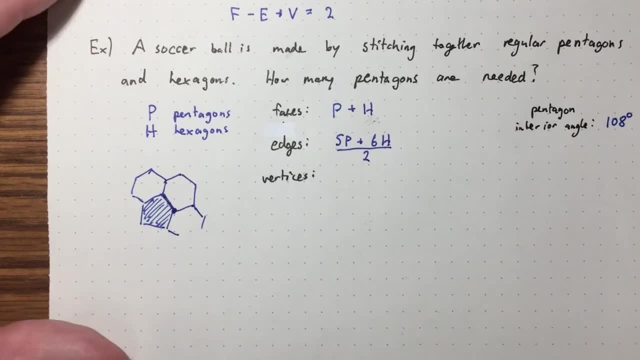 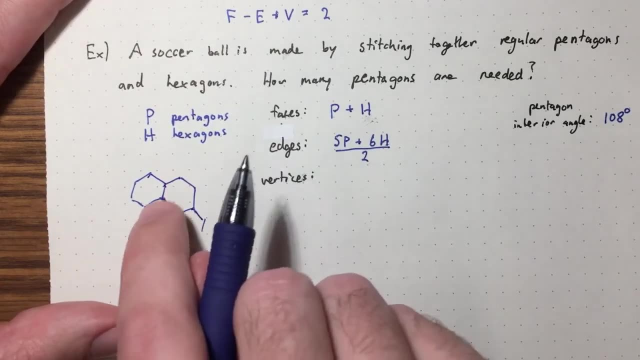 we're over 360.. So that's not a valid shape that we can make. So every vertex is going to be shared by three faces. So here's what I'm going to do: I'm just going to add up the number of vertices. 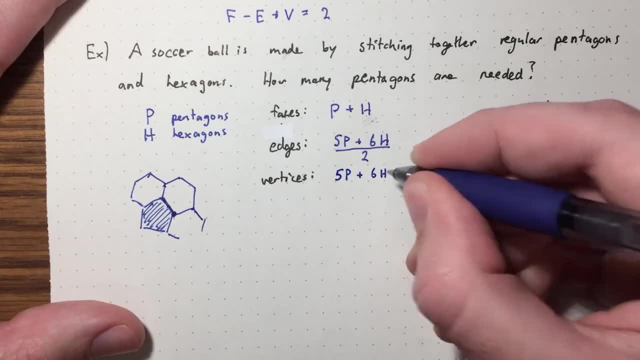 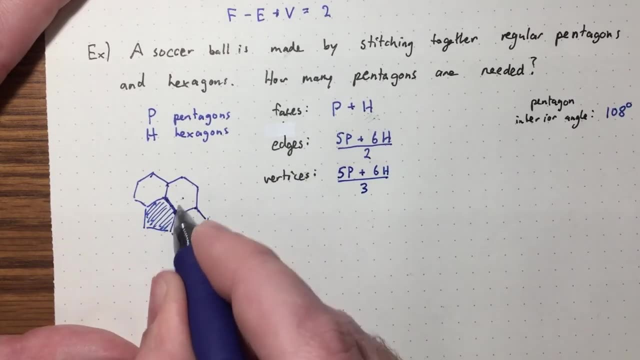 Each pentagon has five vertices. Each hexagon has six vertices, But I need to divide by three Again, because I counted this vertex three times: Once when I counted that one, once when I counted that one and once when I counted that one. 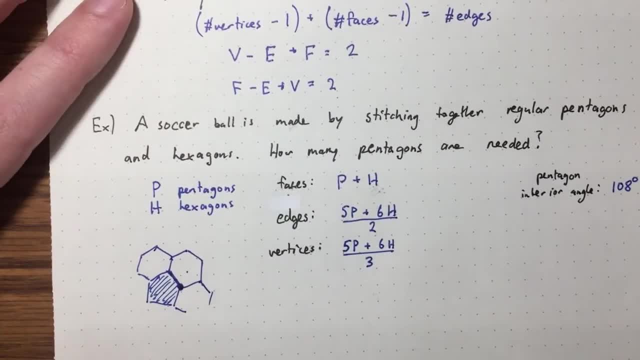 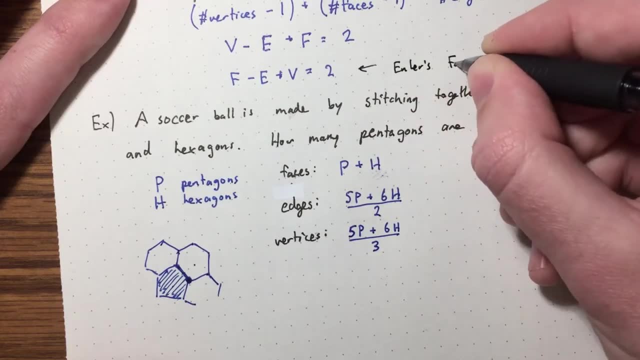 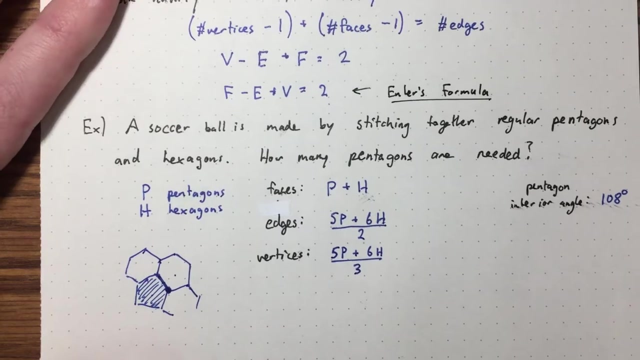 Let's apply this formula. So this two is the Euler characteristic, but this is also called Euler's formula. I don't like using the word Euler's formula so much, because there are probably about ten things that could be called Euler's formula, Most famous being this one. 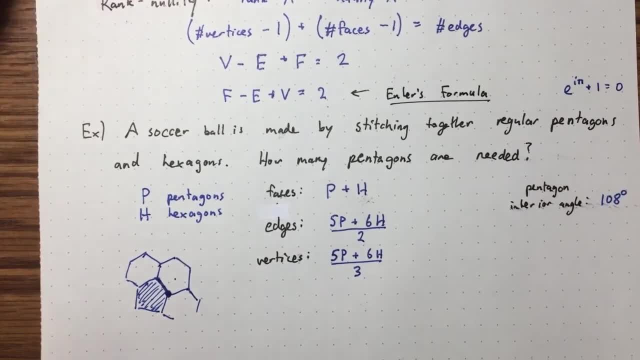 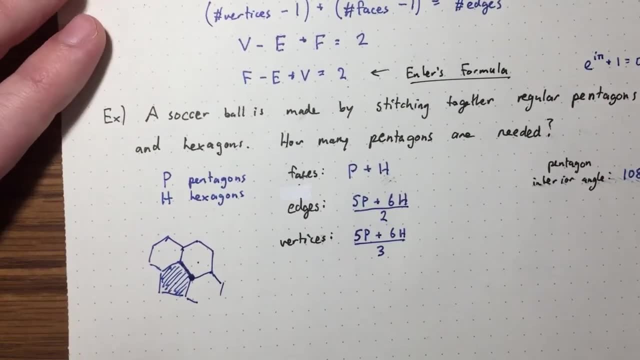 e to the i. pi plus one equals zero. But this really is a wonderful formula. It's probably the second best Euler's formula after this one. Okay, so let's use the Euler's formula here. So we're going to do p plus h faces. 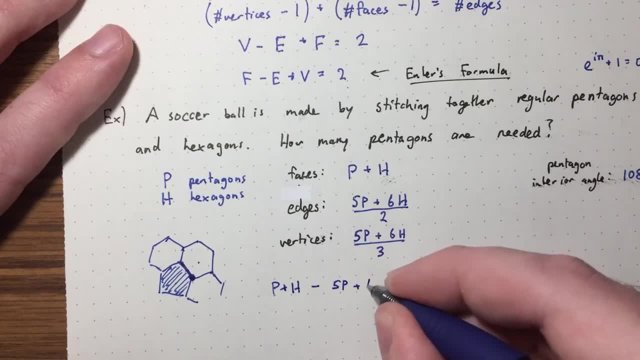 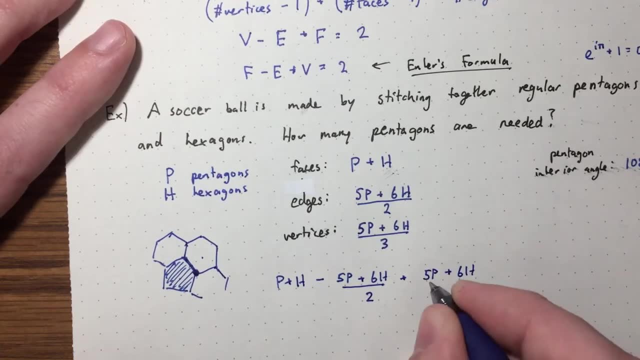 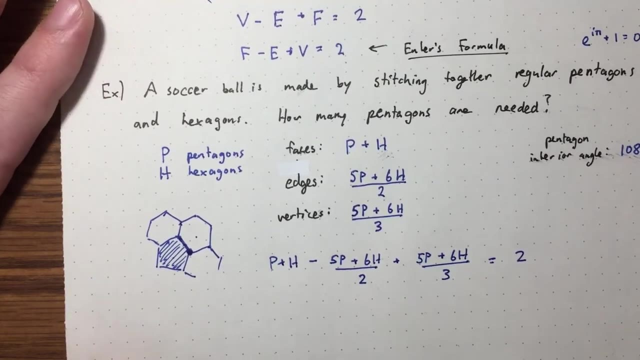 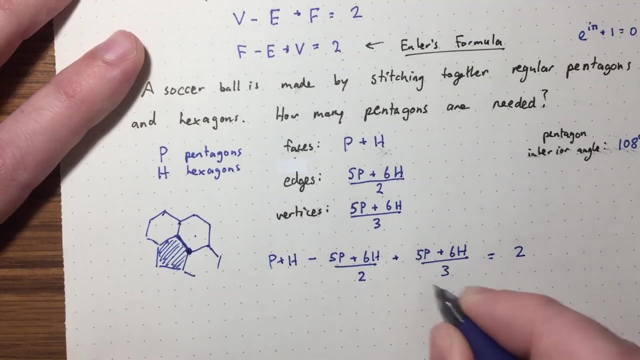 minus edges, plus vertices, That has to equal two. That's what Euler's formula says. Okay, let's try to simplify this in hopes that this might cancel out and be something nice. So I need to find common denominators for the. well, yeah, let's split off. 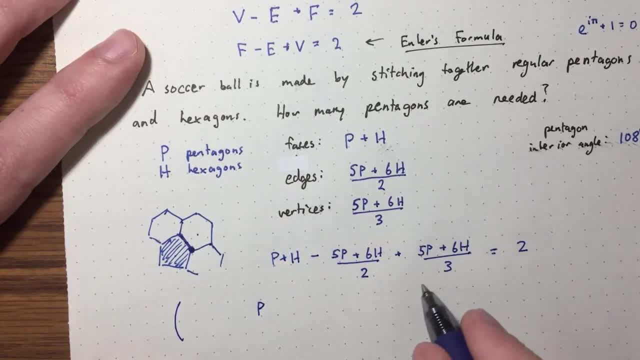 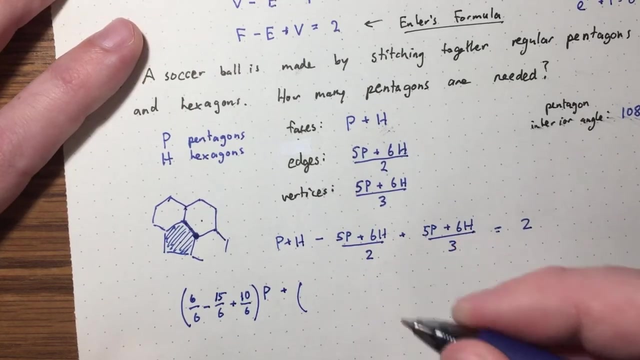 the p terms. So I have p. and what is my coefficient? My common denominator will be six, So it's like six-sixths minus fifteen-sixths plus ten-sixths- Is that right? Plus how about for my h? So I have one h. 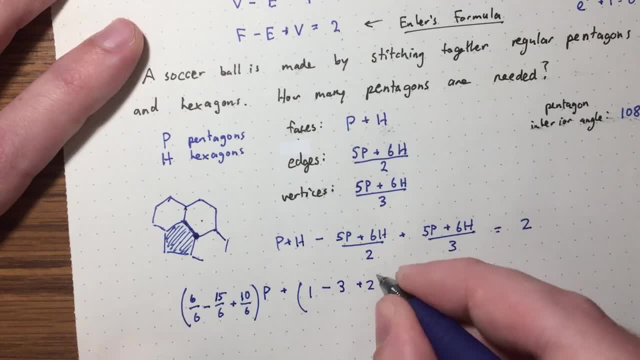 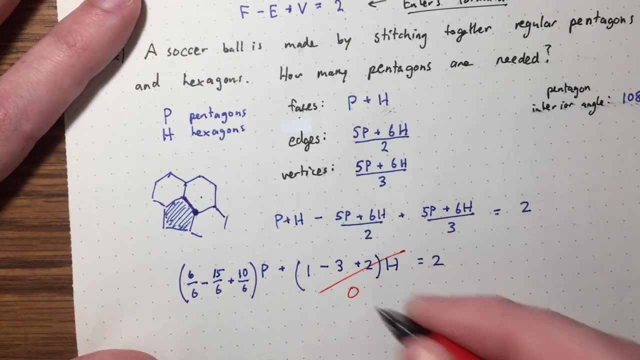 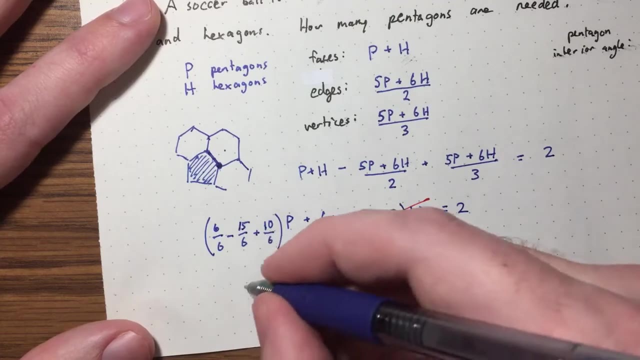 minus three, h plus two, h, That has to equal two. Oh, look at this right here, That's zero. One minus three plus two is zero. What is this? Six minus fifteen is negative. nine plus ten is one, So one-sixth p. 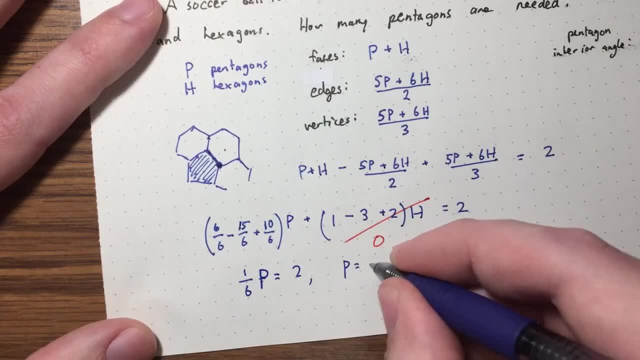 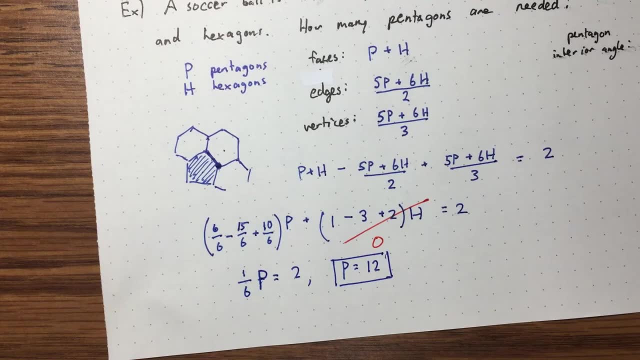 equals two, Which tells me that p equals twelve. That's really cool. So I need twelve pentagons to make a soccer ball. We just figured that out, even though we have no idea how they're arranged And we still don't know how many hexagons we need. 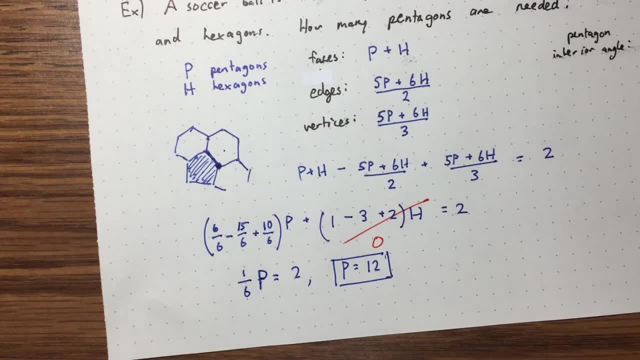 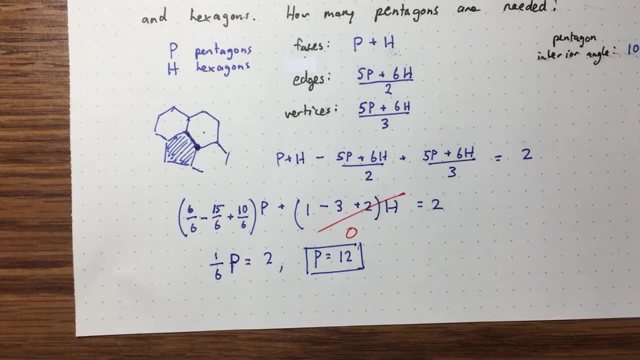 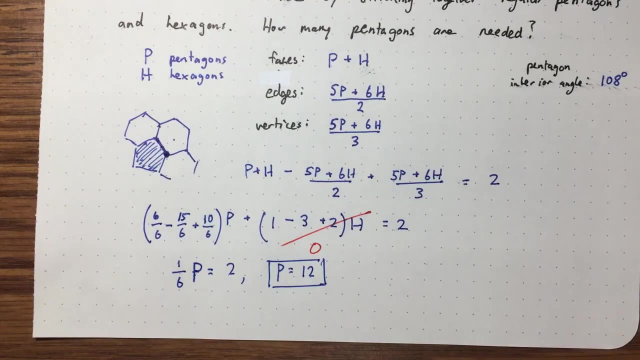 by the way. So maybe that is actually a variable. I think an actual soccer ball uses twenty hexagons and twelve pentagons, But we know we must use twelve pentagons And this came from the Euler characteristic. One other thing I just want to. 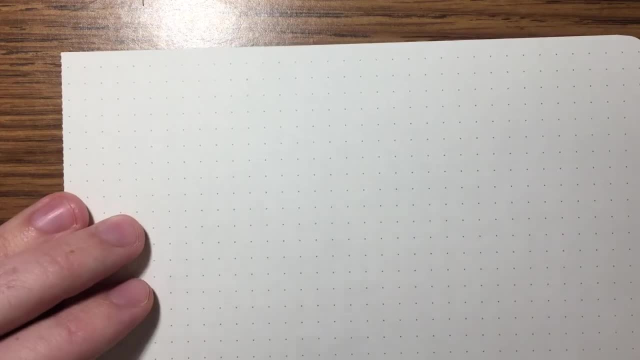 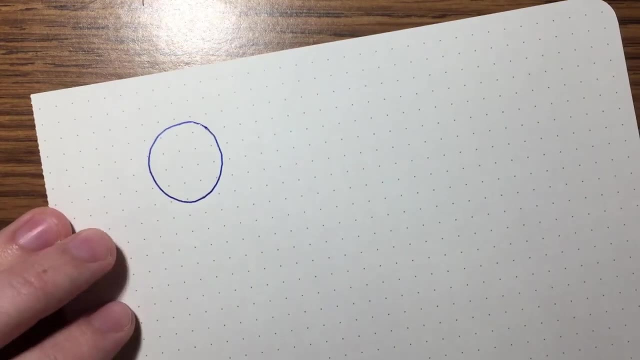 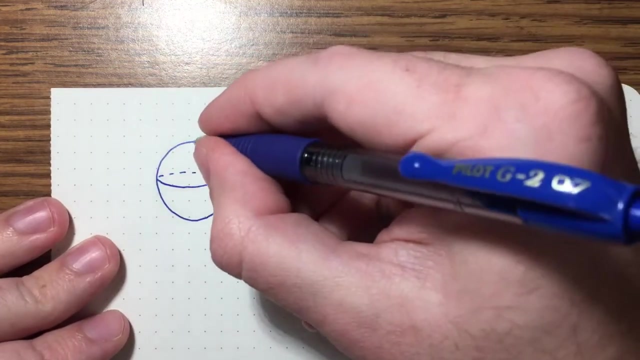 mention quickly, if you're interested in this topic, is that this works even if we have a sphere. So if we start drawing, let's draw an edge on this sphere. So there's an edge And here's another edge that's going to go around this sphere. 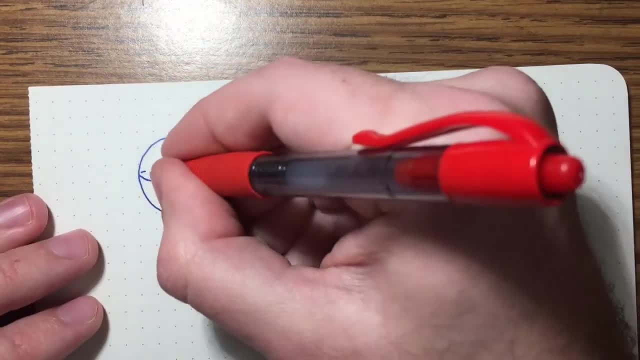 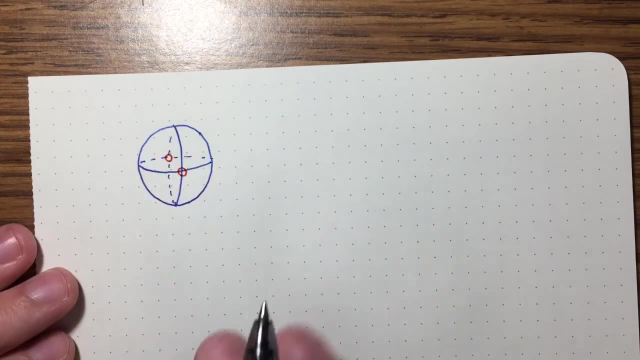 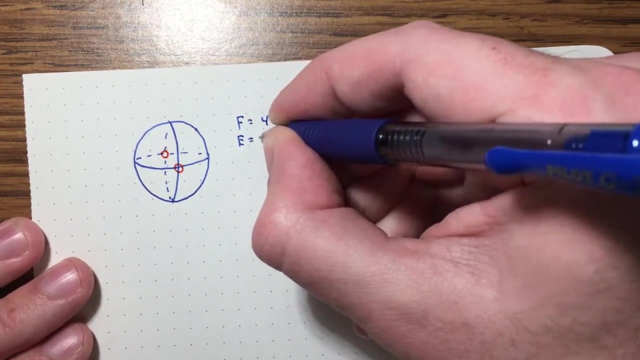 And these meet in two vertices. So there's one vertex, there's another vertex, And we sort of divided this up into four faces. So there are four quarters of the sphere. So we have four faces. We have four edges: One, two. 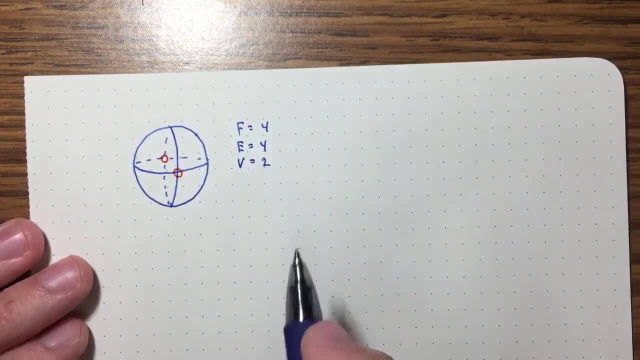 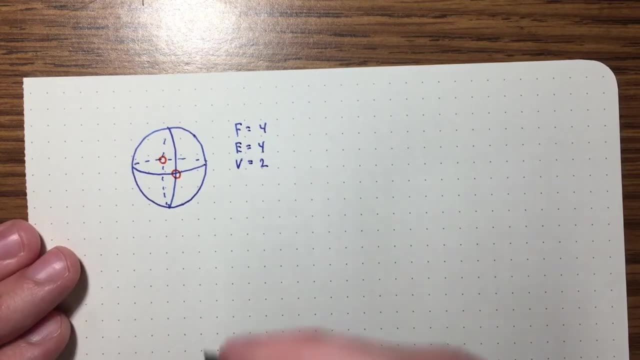 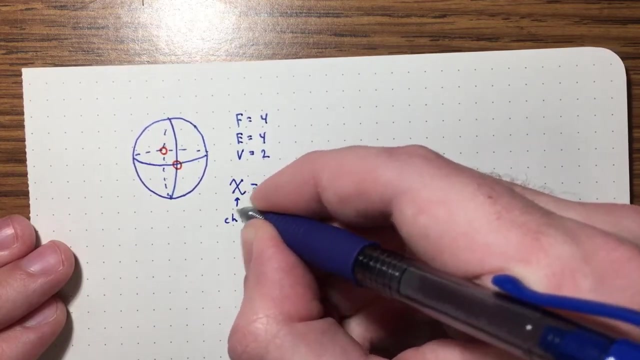 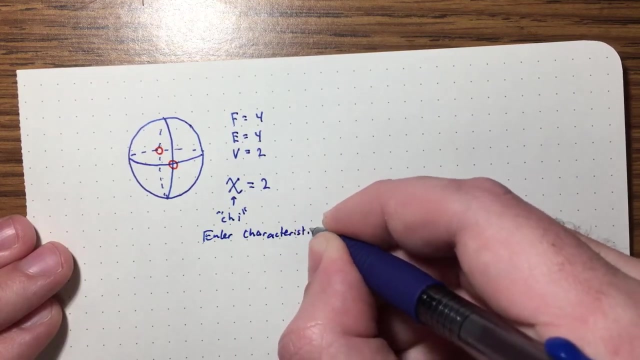 three, four And we have two vertices. Four faces minus edges plus vertices equals two, So the Euler characteristic is two. This symbol is sometimes used for the Euler characteristic, So this is a key, which is the Euler characteristic. Okay, Here's something crazy. 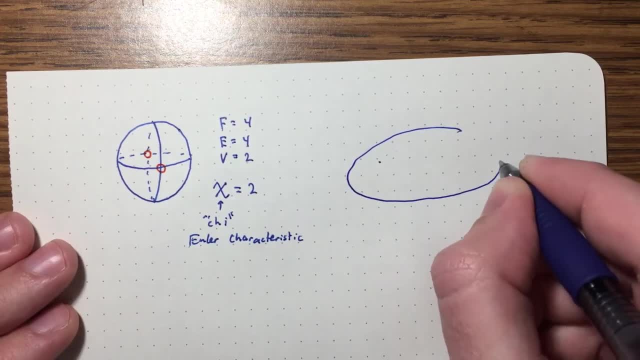 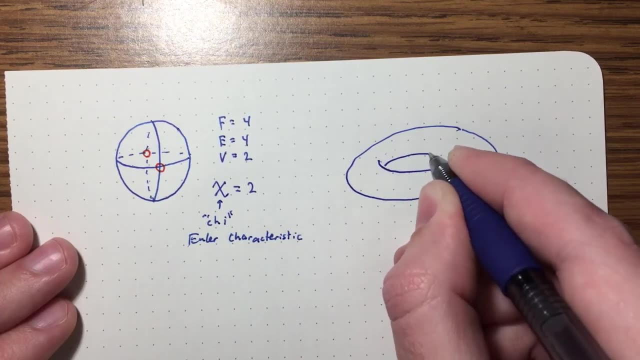 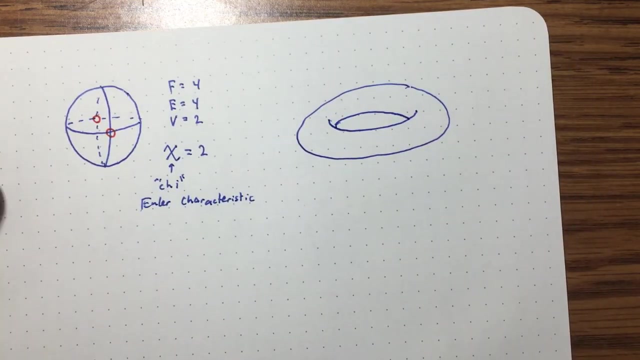 So let me take a donut shape, Also known as a torus. It's a little bit tricky to draw, But let me draw it like this maybe. Okay, I'm going to take this torus And again, I'm going to. 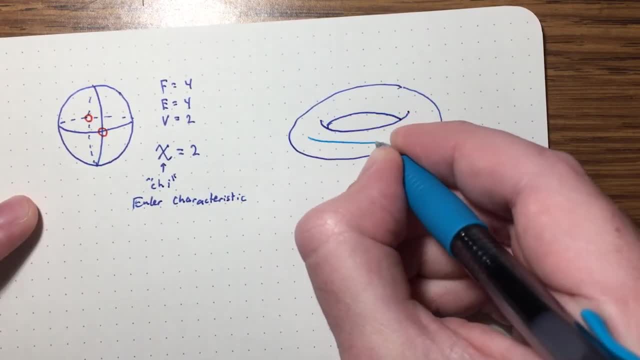 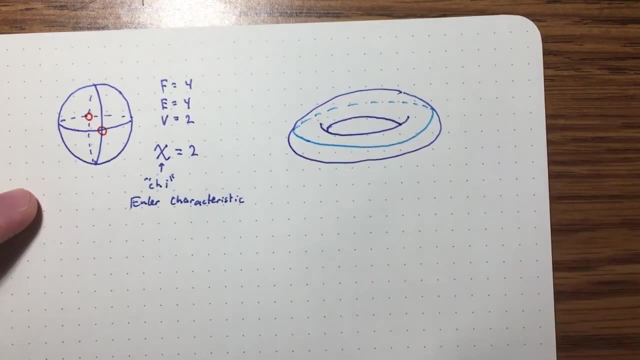 try to use a different color. I'm going to put some edges on here, So I'll put one edge that kind of goes around the donut like this. Now another edge I'll put going this way: I'm just going to wrap around this loop here. 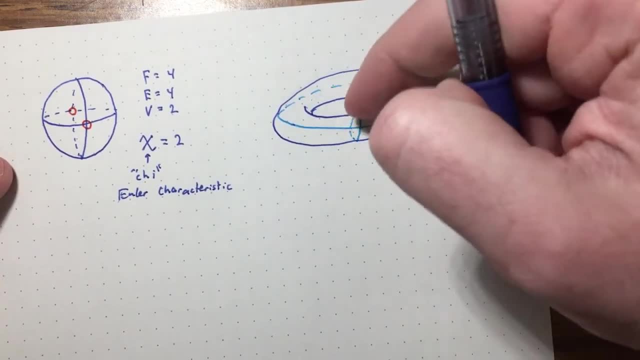 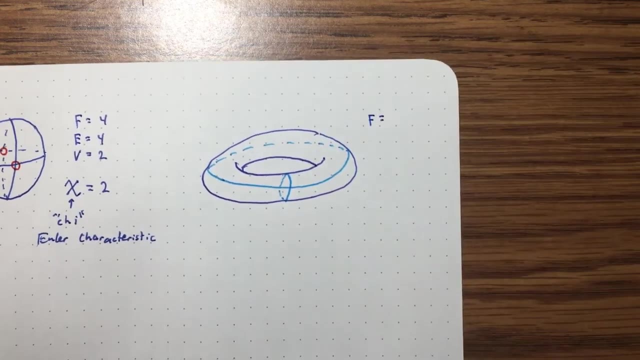 You see how I'm drawing this torus. There's a hole in the middle, So it's like a donut. Okay, Does Euler's formula still work? Okay, So F is going to be. Ooh, this is kind of tricky. 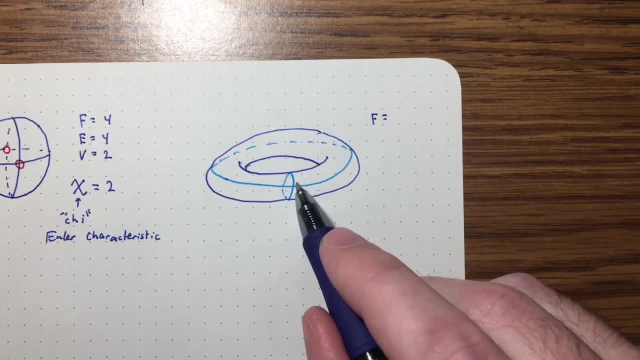 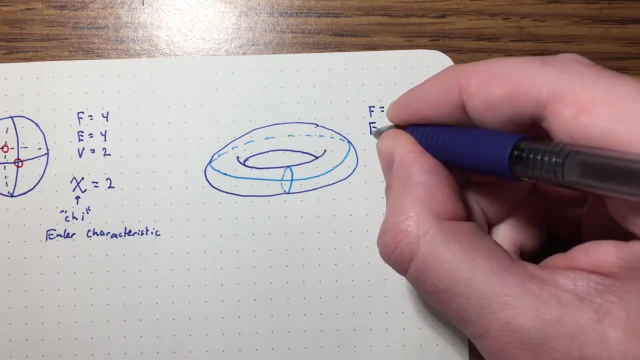 I think there's just one big face, Because if you imagine cutting it here and sort of traveling, you just get one large sheet here. So there's one face. How many edges do we have? Well, we have this edge, and so the only vertex: